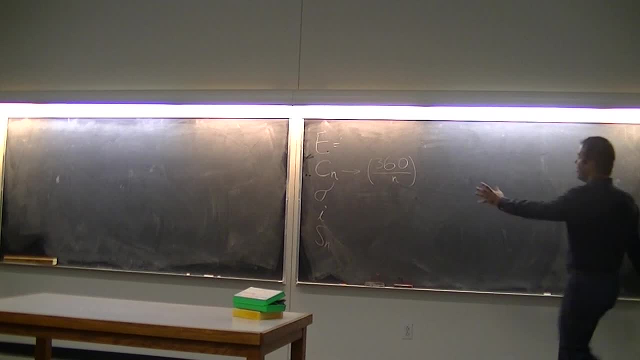 indistinguishable by rotating it by this much. we say that that molecule has that particular c. what do I mean? for example, EF3- right, we know this hybridization is sp2, right? so if you rotate this molecule by 90 degrees, it does not become indistinguishable from itself, right? if you rotate it by 90 degrees, it becomes. 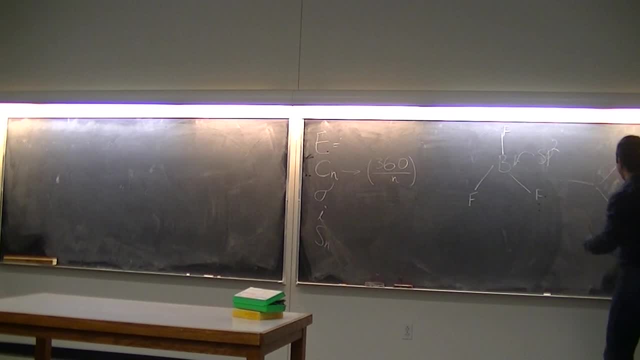 something like that, right? so we don't say that, that by rotating 90 degrees it becomes indistinguishable, so it does not have c4. but if you do the same by 120 degrees it becomes itself. so we say that this particular molecule has c3. it's quite obvious. if you look at the 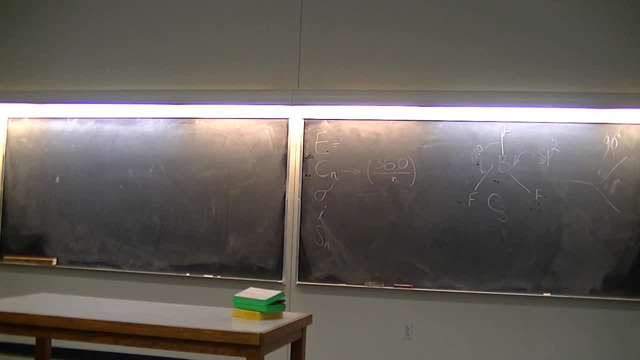 number of elements that needs to be, you know, rotated that that's usually this number down here. all right, is it clear? so if I number this fluorine with F2- sorry, F1, F2 and F3, if I apply c3 once, what does it convert to it's? 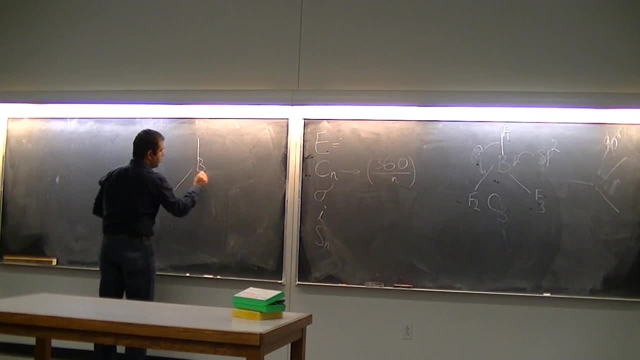 will look like what: F1 will go here, F2 will go here and F3 will go here. this is after applying one c3 right. right it is, and then indistinguishable from this starting point, but at the same time it's not exactly this right, it's a different. 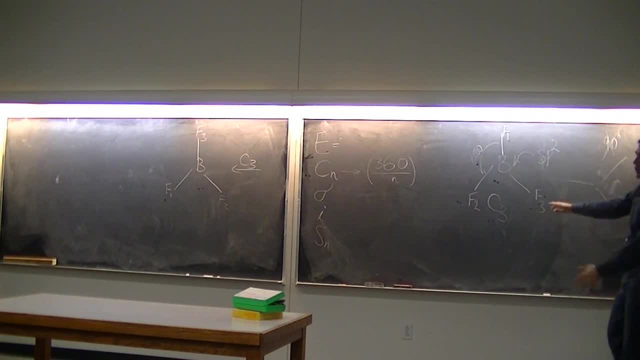 form of this molecule, but it's similar to the starting point state. right, if you do it twice, what is it gonna look like? F1 will go where. come on, guys, talk to me. F1 will go first here and then there. right, so F1 will go here. 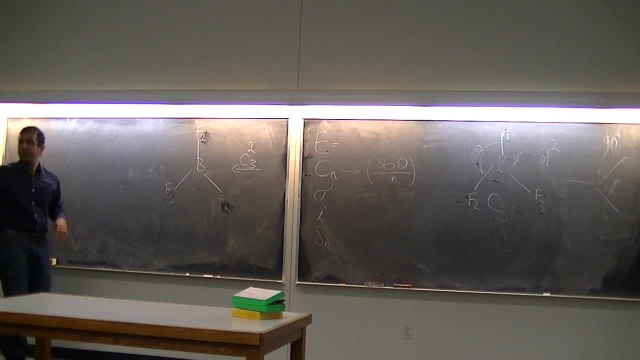 F2 will go there and F3 will go here. there, if you do three times, you retain the starting configuration. right, it exactly becomes similar to the starting structure that you right. so F1. so doing c1, c3 once and doing c3 twice will give you structures that are not exactly the 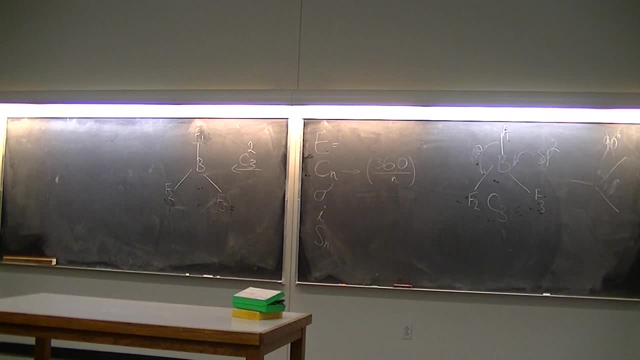 same but it's similar. but doing it three times will retain the structure, right that if by an operation you can retain the starting structure, that's And that is called E. So basically, C3 equals 3 times E. So you might wonder what is this E good for right? 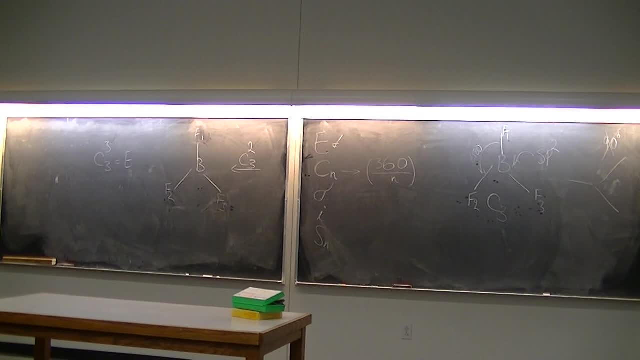 It's always there, right? So why do we have E if all molecules have E? We use E to distinguish C1, C3 one times from C3 three times. This is like exactly the same, something similar to the same. So do you get why we have E? 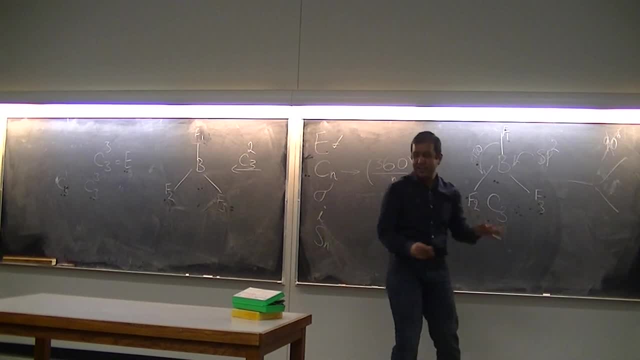 All right. so E is when something becomes exactly itself, And basically it's C1.. If you rotate the molecule by 360 degrees, it becomes exactly itself. Are you good with C and Cn rotating by one nth of a turn, Anti-clockwise, Okay. 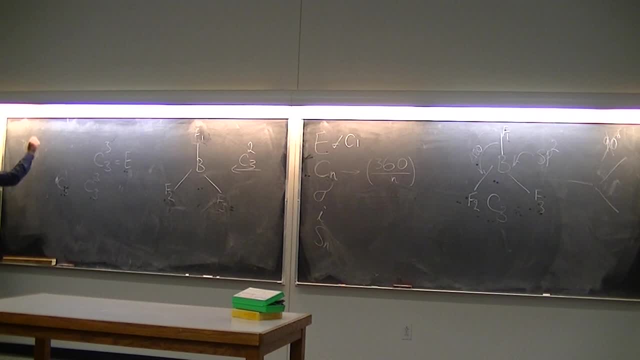 And it's obvious that Cn. if you do Cn n times, it's actually E, right, It becomes itself again right. If you rotate the molecules by 90 degrees and do C4, okay, If you do it twice, what are you doing? 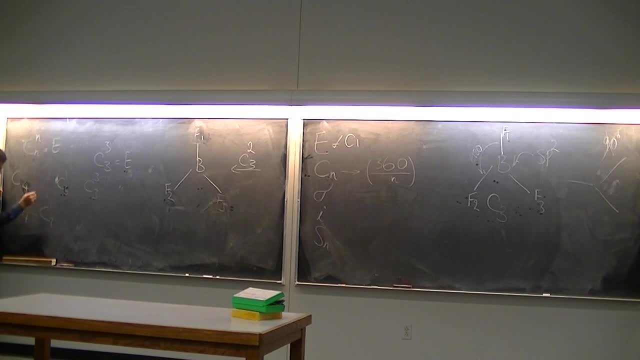 C2.. Yeah, exactly. So if you can simplify those numbers up and down, go ahead and do it, It's fine. So, Yeah, Okay, Let's go to sigma. What is sigma? It's reflection, right? So if you have a mirror plane inside your molecule, 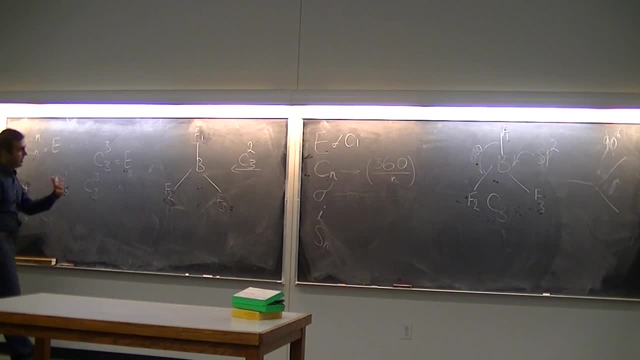 which can reflect the two sides of the molecule so that you get the structure that is similar to itself. we say that that molecule has a sigma. Okay, So, for example, let's take this molecule- First point, Flat molecules, planar molecules. they always have a sigma. 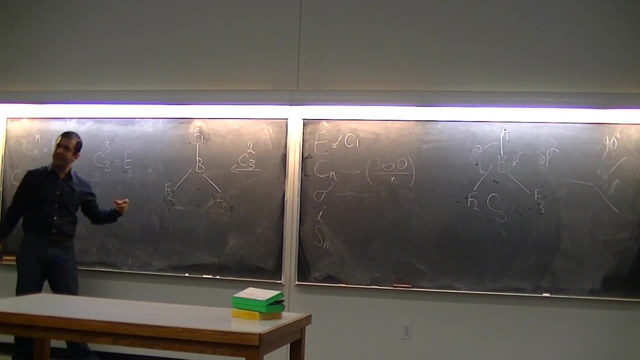 Because they are flat, Okay. So the first sigma that you see here should be what? The plane of the board? Okay. It also has some sigmas that are like this: right, If you can think of a mirror plane that goes through this M and this Br. 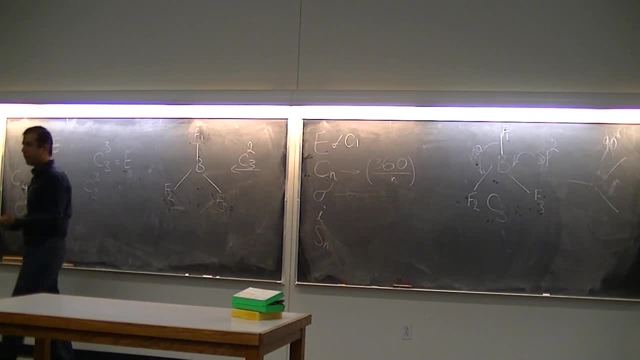 and reflects this F2 to that F3, that's also another sigma. Do you all see it? Alright, There's: If you apply C2, does it not do the same thing here? If you rotate it by 180 degrees, it just does not touch those two. 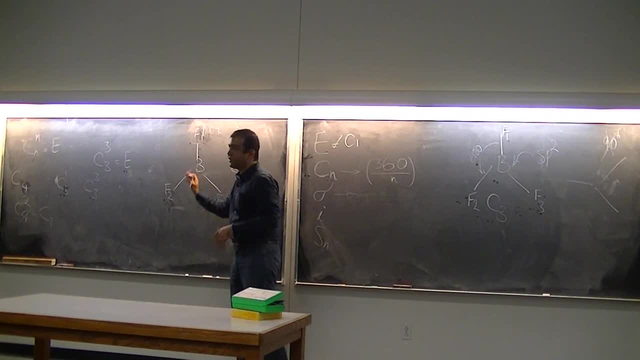 It reflects this to this and this to this, And if you apply sigma, it does the same thing, right, Do you agree? Yes or no? Yes, Yes, but So, but sometimes they. So I'm trying to tell you where you can make mistakes. 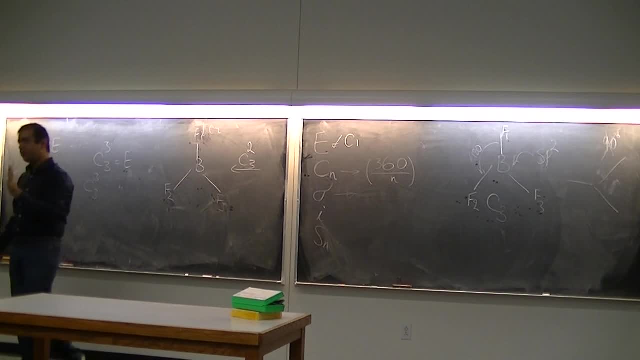 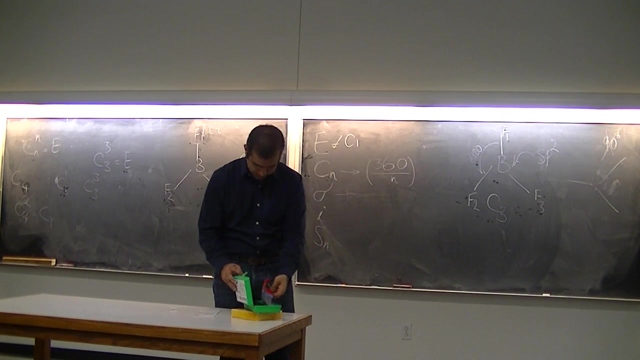 It looks like C2 and SEPA sometimes do similar stuff. But be careful They are. They sometimes do similar stuff but with different mechanisms. So let's say, Okay, let me use this one. I'm not very used to that. 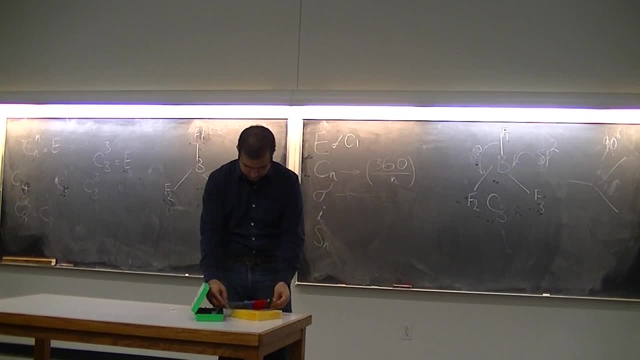 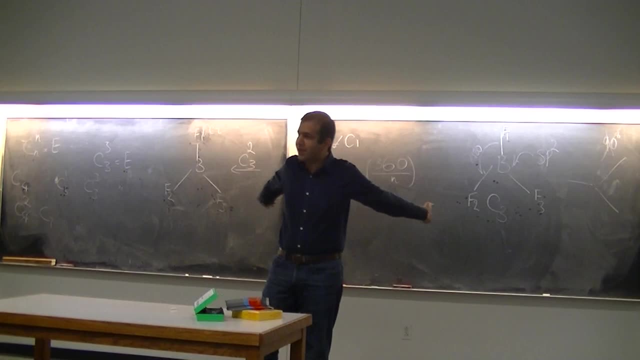 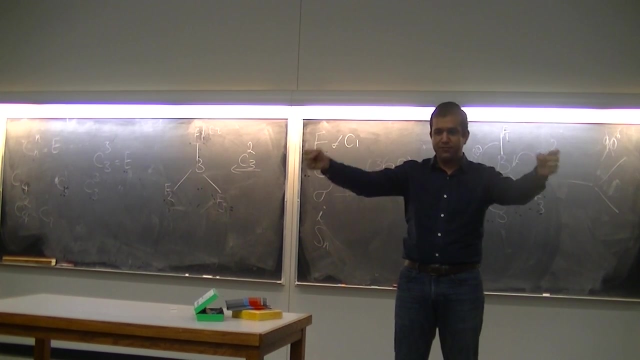 Let's see what I have here. Okay, let's use my hands. It's easier. Assume that I have two more hands in the back, Okay. So two hands here, two hands there. Okay. If I do sigma through my body, okay, my front hands will be reflected as well as my back. 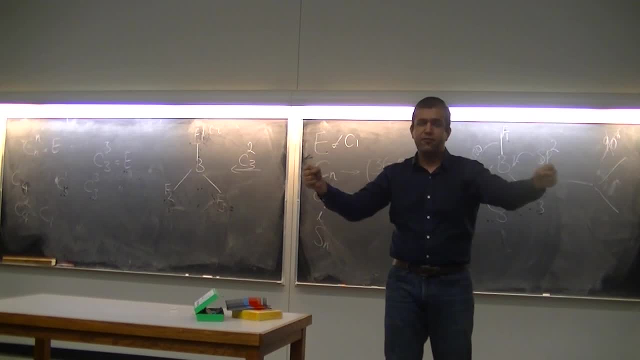 hands Okay, But if I do C2, the front and back will be, you know, kind of related to each other. So the idea: Have you seen like horror movies, When there's like souls and they go through walls? 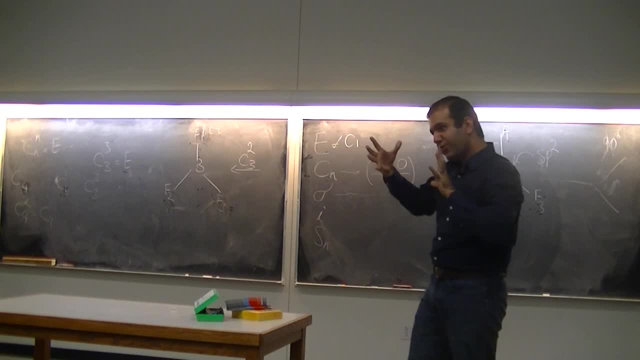 No, really. I mean that's a good projection. Souls that like go through the wall, that's sigma Okay. But if the like, whatever, that is that thing, that horrible thing if it opens the door. 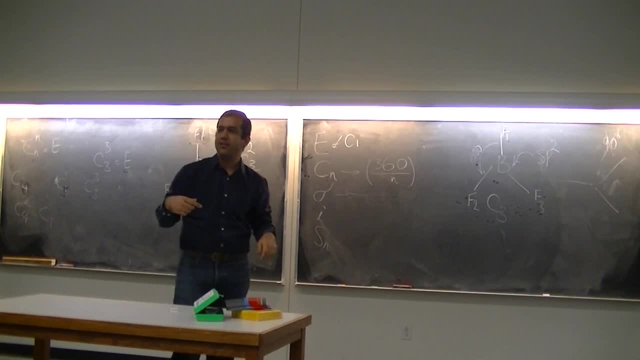 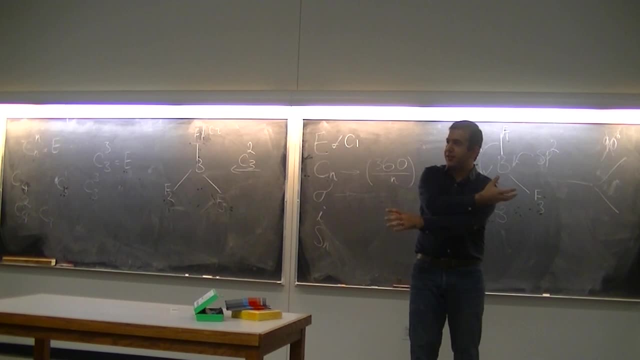 and goes to the other side. it's CN. Okay, So CN takes something from left and side, bring it to the other side by rotation, Okay, But sigma does it by just going through the wall. So these two kind of go that way. 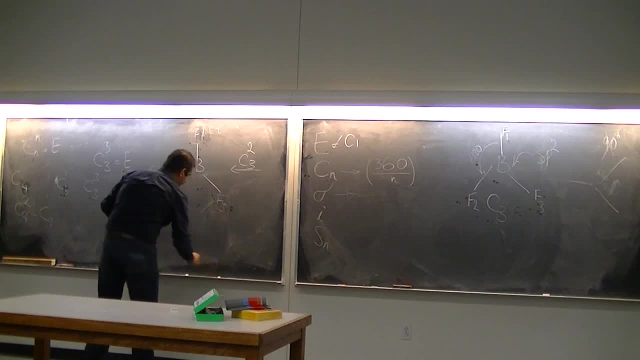 Okay If I were to give you an example with molecules. let's say we have a molecule that is like XEF3.. F1, F2, F3, and F4.. Okay, Okay, So, Yeah. So, for example, if I do a C, 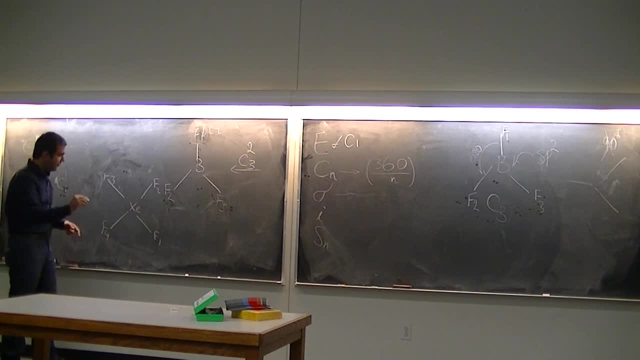 I know it has C4. But if I do a C2 here, right, what will happen? It will just rotate and go to the other side. So this goes there, Right. But if I go to do reflection, it just goes through the wall and goes to the other side. 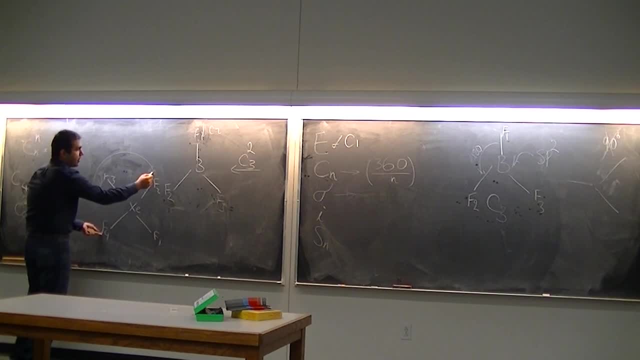 It's important to distinguish. Okay, So sometimes they do similar stuff, but with different mechanisms. One of them is just reflection, the other one is rotation. Okay, So I'm going to show you how to do it. Okay, So I'm going to show you how to do it. 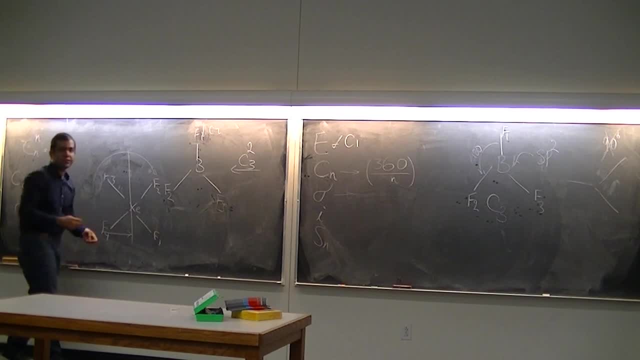 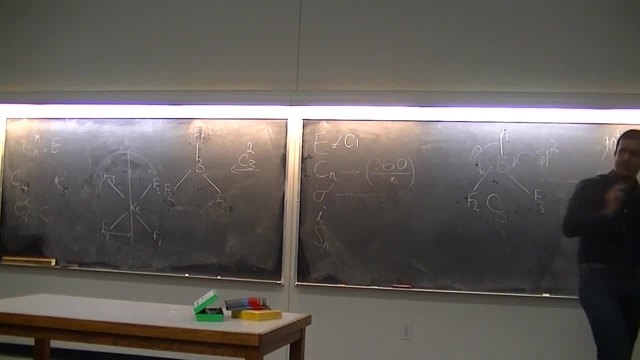 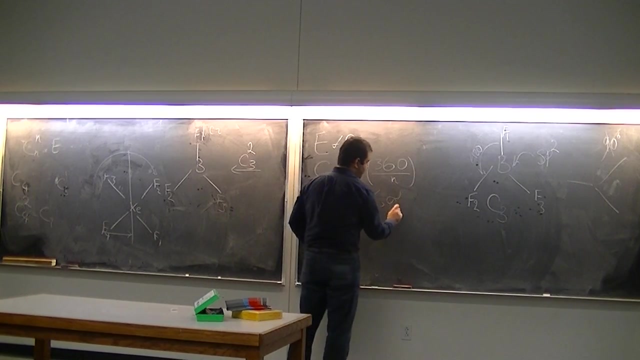 One of them is just reflection, the other one is rotation. Okay, You got it. Okay, What else? Okay, We have two different kinds of sigma. Okay, We have sigma h and sigma d. We also have sigma d, but you don't have to distinguish sigma d and sigma h. 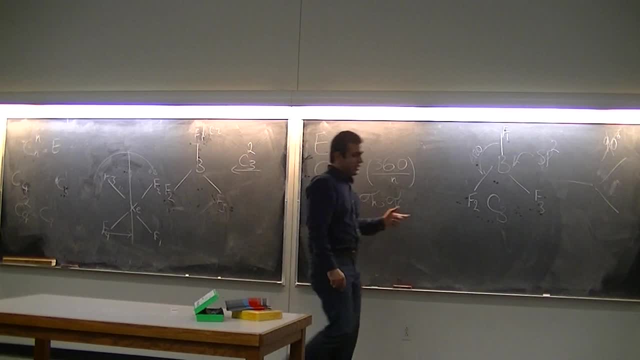 So what is sigma h? Usually the molecules that you will be given have the same mass, have different types of Cn. They have like a C5 and a bunch of C2s. for example, They have a C4 and a C3 and some bunch of C2s again. okay, 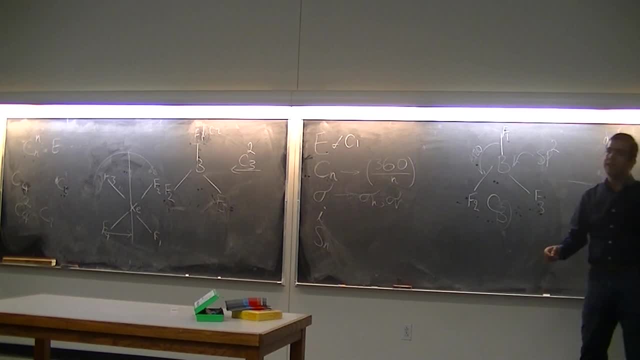 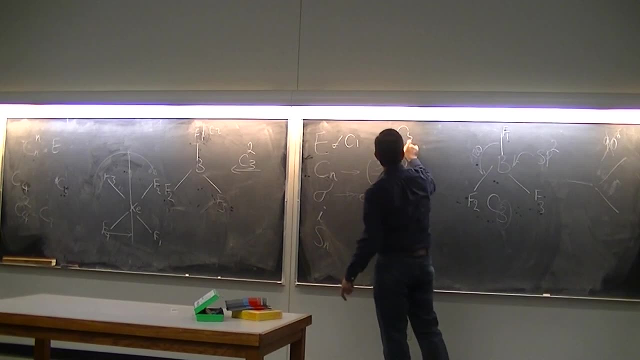 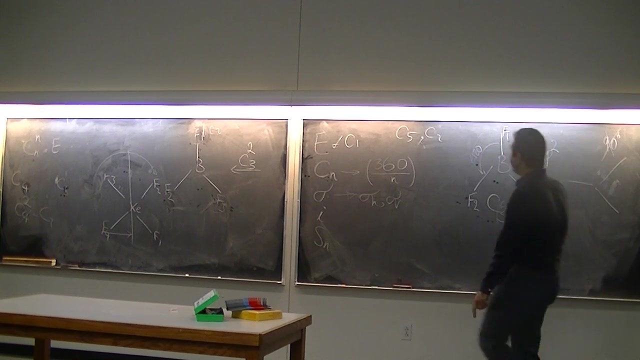 So we usually call the Cn, the highest number, as the main principle rotation, rotation axis. okay, So if your molecule has C5 and C2, which one is the main rotation axis? C5. C5, so C5 is the main one, okay? 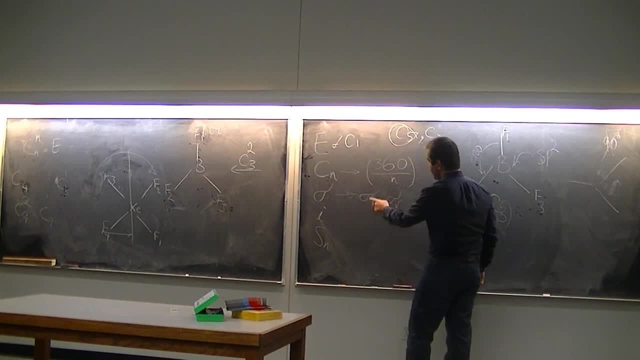 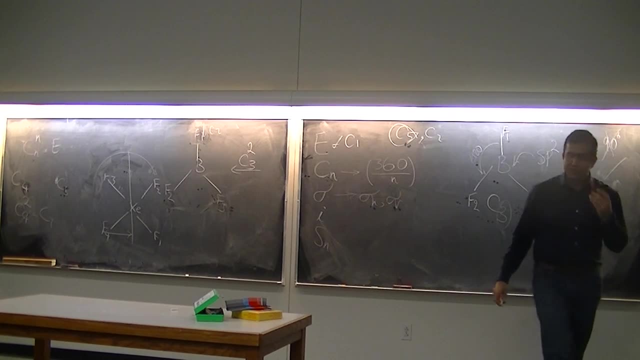 Now, in order to figure out which one is sigma H and sigma V, and which one is sigma V, we have to compare the sigma with that C5.. If your sigma is perpendicular to that C5, we call it what? Sigma H. 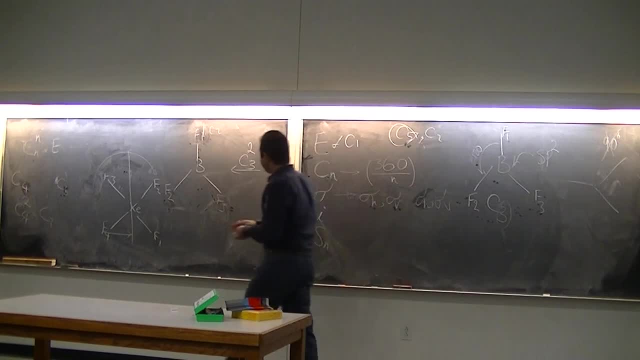 And if it's parallel, we call it sigma V. Let's get to that BF3 example. So what are all Cn's that this molecule has? C? what C3.. C3, very good. Where is it Through that thing? 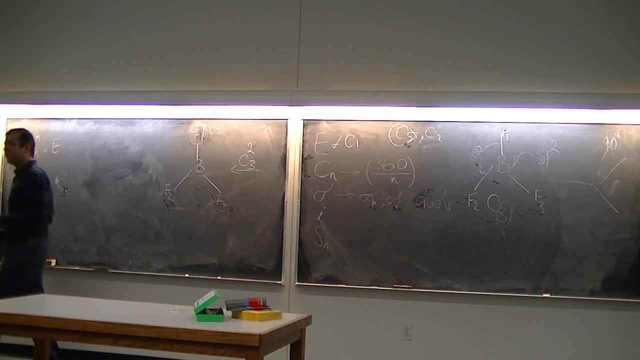 Yeah, So we have a C3 like that and what else C2.. Yeah, how many C2s? Three. So it has three C2s, one through there, one through there and one through there, right? 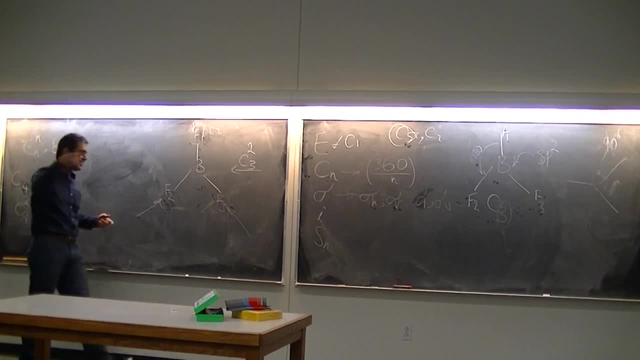 Which one is the main principle: axis C3.. C3, so this is the C3. So, to judge whether it's sigma H or sigma V, we do not use those, okay, We just use the C3.. Now, where are the planes? 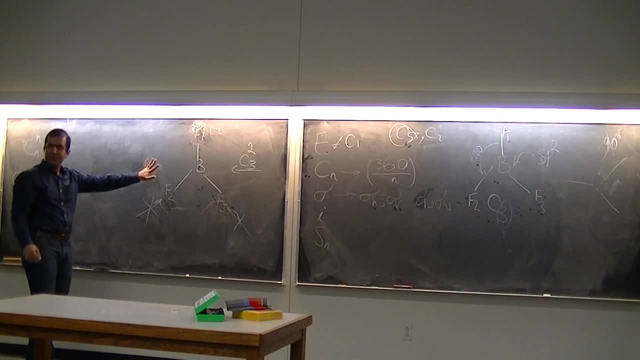 It's a flat molecule. so where's the first? This is the easiest to pick. Yeah, the plane of the book. Yeah, So we have this and we have some other planes. Can you identify those? The one that is parallel to C2?? 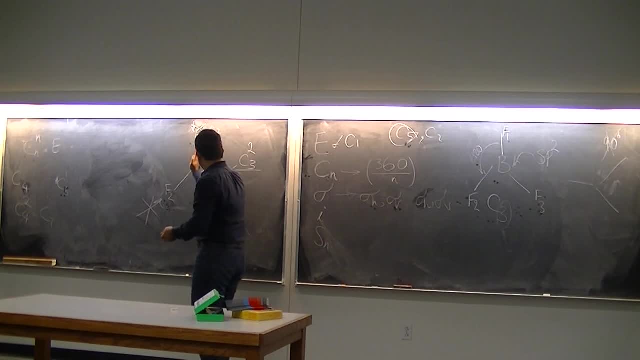 Yeah, exactly. One of them is like that: right, That goes through this B and F and reflects this F2 and F3.. Another one is like that that goes through this F and this O Reflects those two. and there's another one like that: 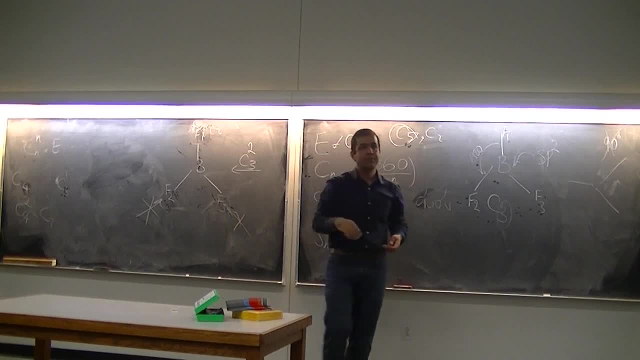 That goes through this and this and reflects those two. Right, So this, let's pick the first one, this sigma. Where is the CN again? Yeah, exactly, So these two are what? what is the relationship? They are perpendicular. yeah, 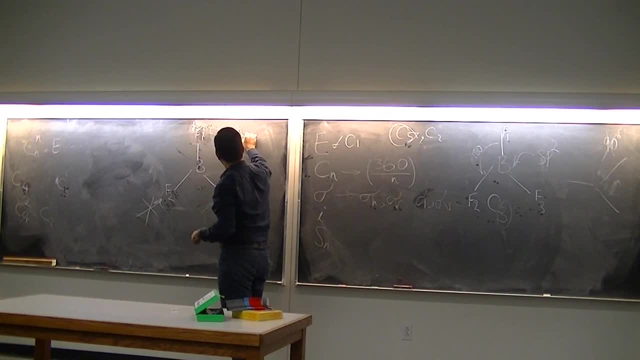 So this is what the plane of the board is. sigma H. Another way to tell is this: You always have one sigma H, Okay. You cannot have multiple sigma Hs, Okay. What about the other sigmas? This, this, this: 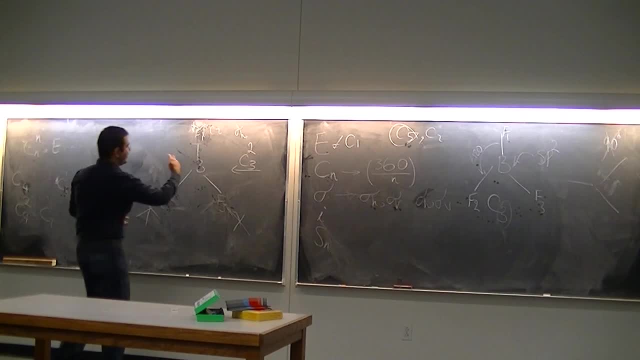 They are somehow similar, right, They are parallel to that CN. So if this is one of your sigmas, the C3 is also there. So since they are parallel, we call them sigma B. Okay, You got which one is. so, if they ask, 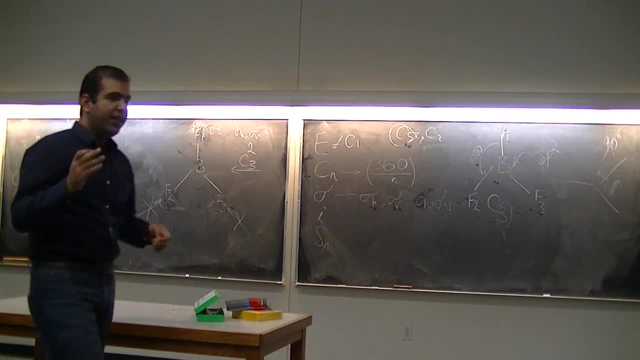 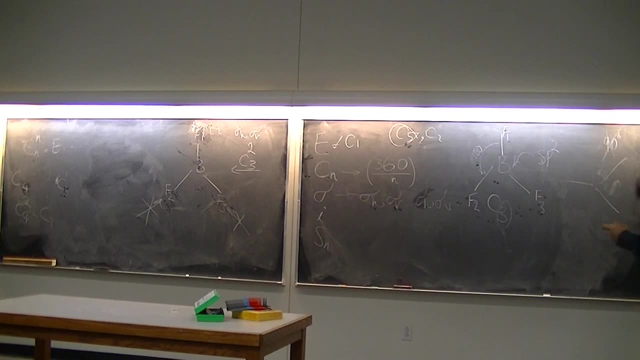 if I ask you what is sigma H and what is sigma Three, The answer you have to first consider C. Here is CN. Okay, Tell me. okay, here is CN. Now, with respect to that CN, you are playing a sigma H or sigma? 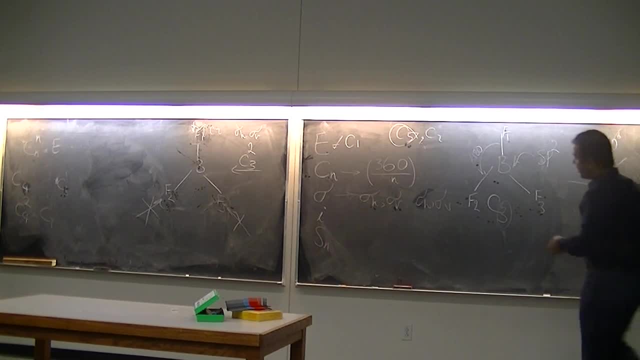 Is it clear? All right, What is I? I is center of inversion and it's similar to sigma as like things have to go through it and find the other side. But all of those you know, reflections are through the center, Like this molecule it does not have I. 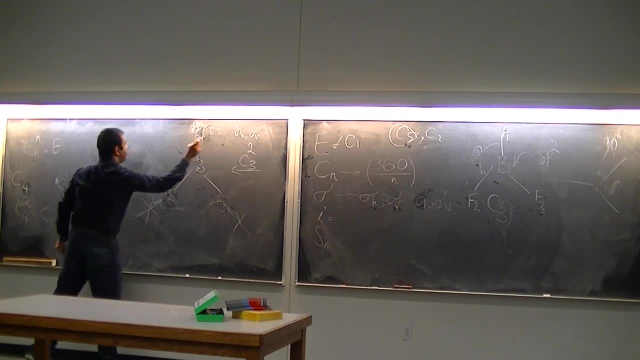 If you apply I on this molecule, this will go there, This will go here and this will go there. It is not that Okay. So this molecule does not have I. But if you take the XE, this molecule does have I. 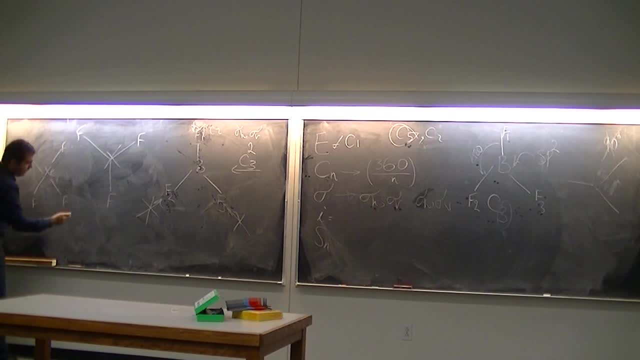 I think I is there. And a quick thing: S2 is the same as I. I'll explain it later. Okay, I'll explain it a little bit later, but just memorize it. Okay, S2 is the same as I. 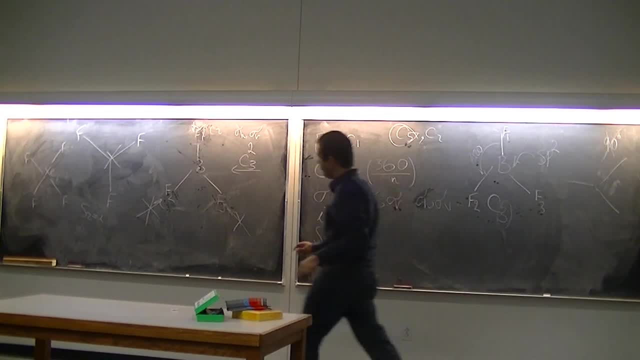 Any questions about? okay, before I continue this, let me tell you something. So sigma is applying a miracle, right? What is sigma squared? if I do sigma twice, what happens? What E? Yeah, exactly What is I squared? 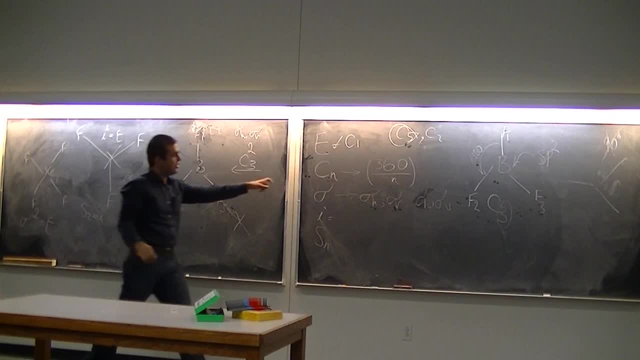 E, E again, okay. So what So? CN? You have to raise it to N to reach E. But sigma and I, you have to raise it, you have to square it. Okay. What is SN? SN is applying CN and then applying sigma H. 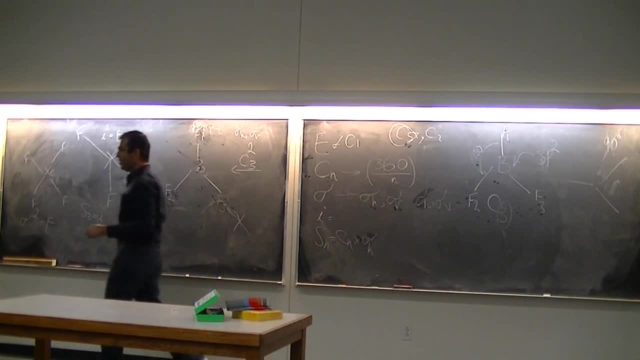 And this sigma H is perpendicular to that CN. Okay, So it's not necessarily the CN of the molecule, It's the CN that you just applied. So what is that? Why do we need such a thing? What is SN? What is SN? 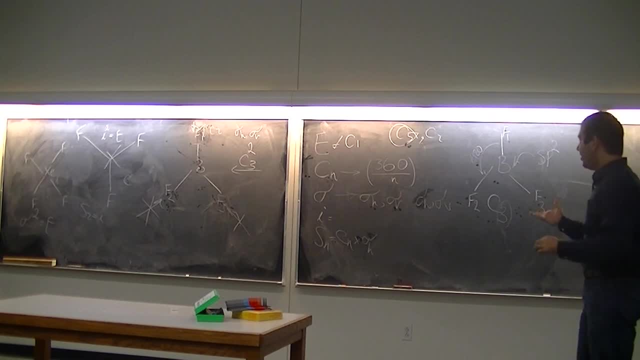 Okay, Yeah, I know. So why don't we make another combination from CN and I? What is this? Where did it come from? There are some molecules that do have the CN and do have the sigma H, And it's not a surprise that they will have both of them together, right? 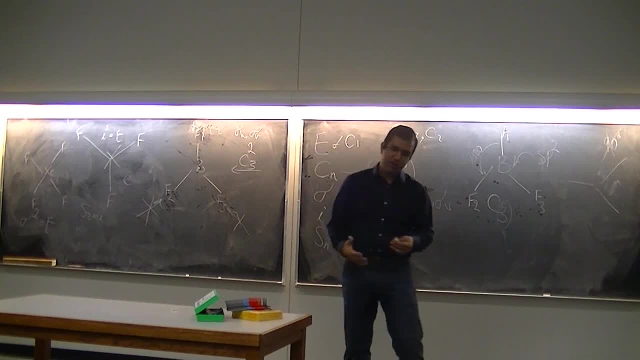 So this is an example. I said yesterday: I am a boy and I'm 30 years old, right? So it's not a surprise to say I'm a 30-year-old, 30-years-old boy, okay. But there are some molecules that are not going. they are not 30 years old, but they are 30-years-old boy, okay. 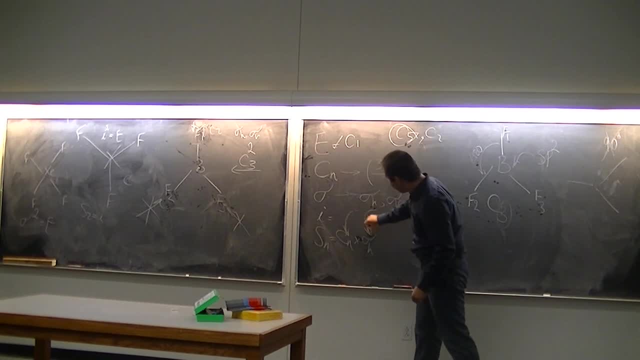 There are some molecules that don't have that, don't have this, but they have them together And that's why they invented that SM, Because there are some special molecules that have some sort of symmetry that cannot be described by any of them alone. okay, 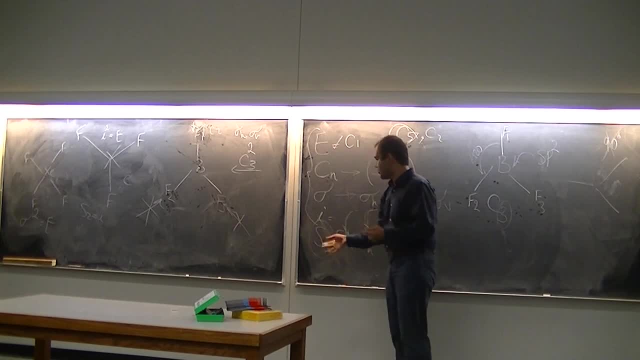 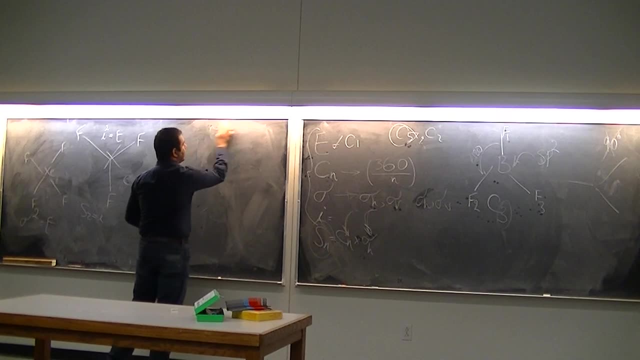 That's what, that's what. so they said, okay, we have to make another operation and that's the SM. I'll explain to you the SM. Okay, okay, But don't worry, those molecules are not like so frequent. 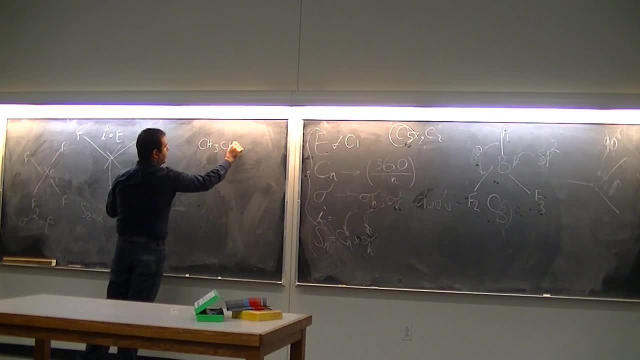 So C3, CH3CH3, right, SM. So if you think of this molecule, it well you know this Newman projection from organic chemistry, right, What is this structure? Staggered, right, If you have the staggered configuration, what is the highest CM? 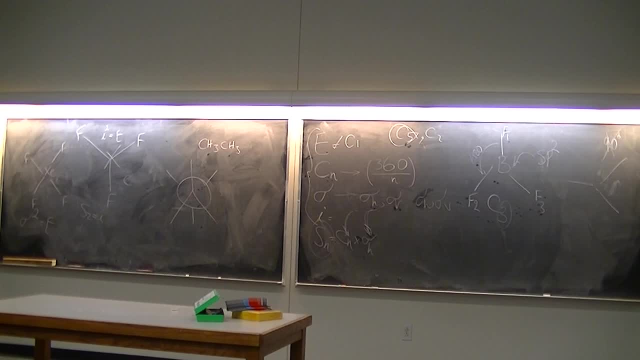 C3. Do we all agree that it does not have C6? Right, It does not have C6. And it does not have the sigma H. agreed, Remember sigma H. And if you apply it, if you apply the plane of the board to a molecule, everything in front will go in the back and everything in the back will go in the front. 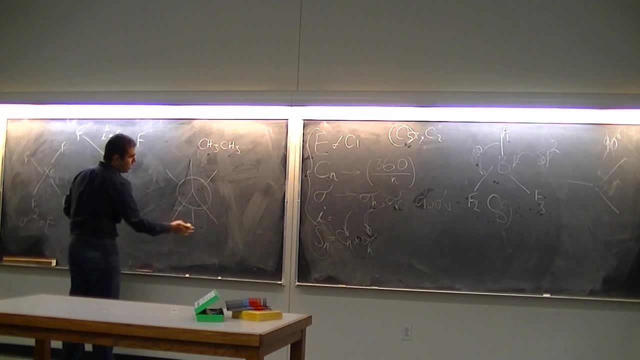 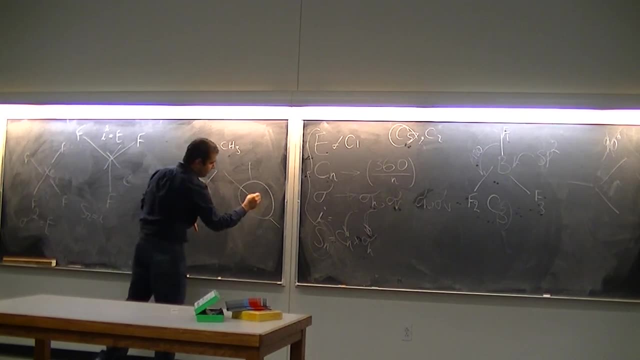 So that triangle that is in the front and is pointing up will go in the back, And that triangle in the back that is pointing down will come in the front. This is not that, And if you, and so it does not have C6, it does not have sigma H. 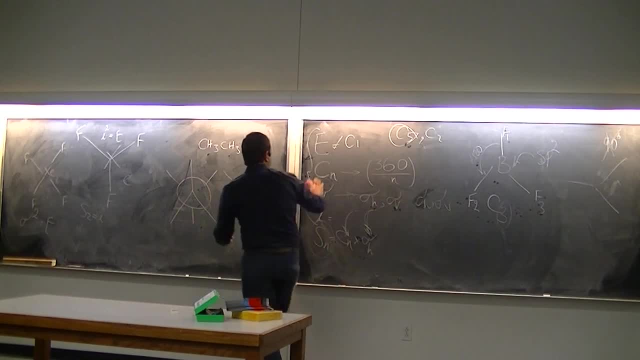 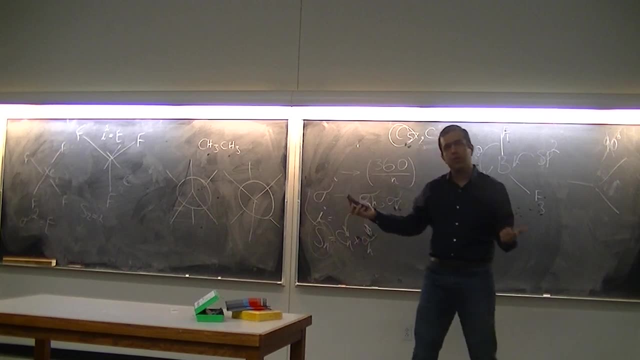 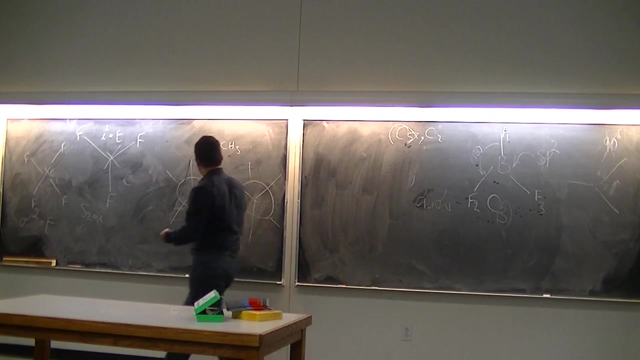 But if you apply both of them, it will become itself, And this, this sort of symmetry, cannot be explained by any of those. That's why we have SM. Okay, So let me take this and apply C6.. If I apply C6, what is it going to look like? 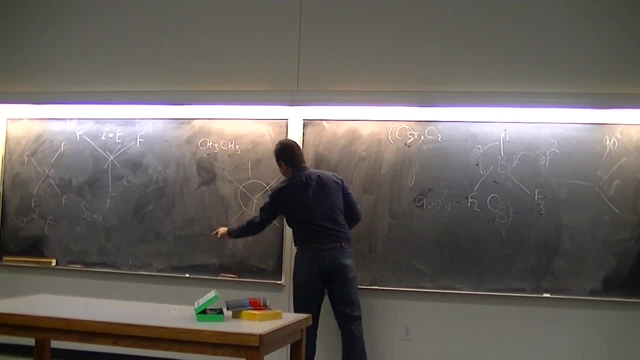 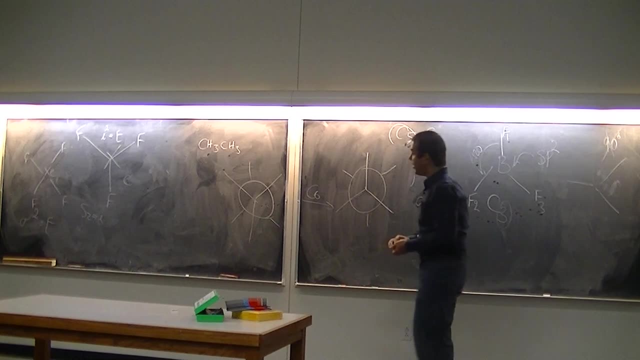 I'm going to rotate it by 60 degrees, So this will go there. It is going to look like that, Do you all agree? Right, If I just rotate so this, there's this triangle in the front, because it's. it's the way the Newman projection works. 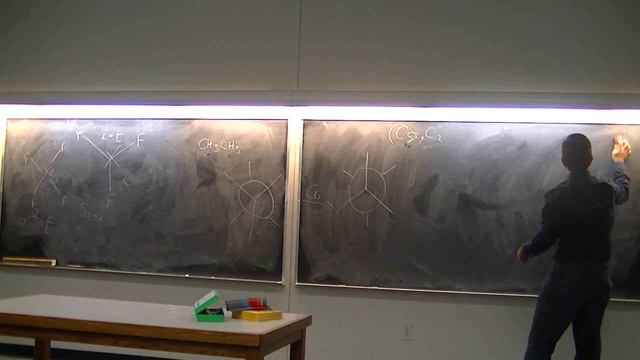 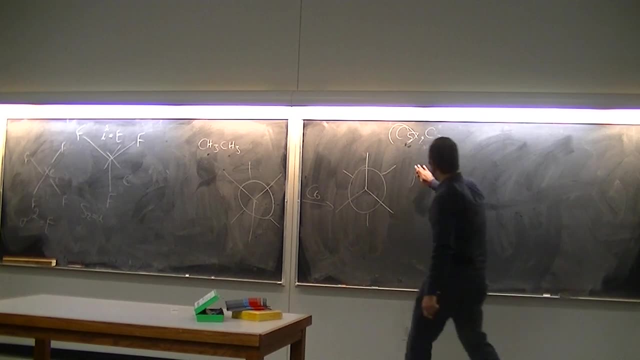 There's this triangle in the front right And I just rotated it by 60 degrees right. It becomes and it's different from that. But if I apply sigma H, This one in the front, It will be and it will go in the back. 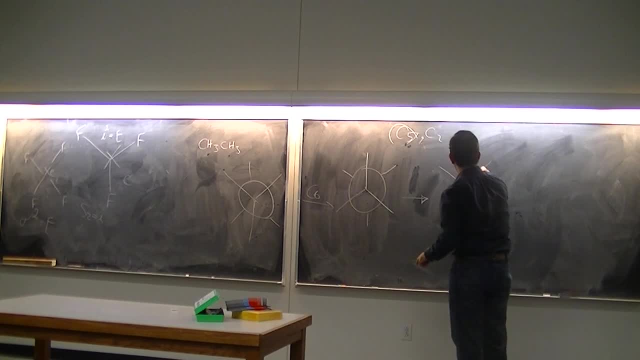 And that triangle in the back will come in the front Right. So it is going to look like that, Right, And it is the starting point. Okay, So we say that this molecule has what? S6. If your molecule has CN and it has sigma H, it will have SM. 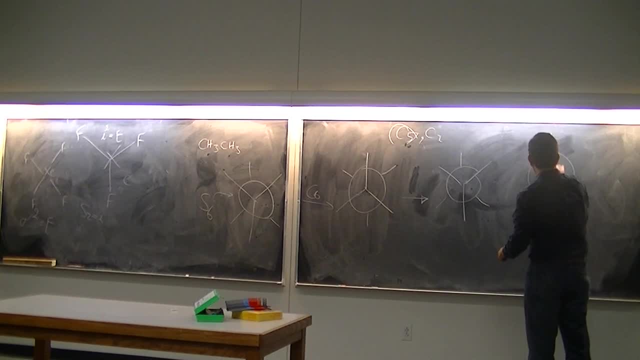 Okay. So if I think of the eclipse configuration Right, Does it have C3? Yes. Does it have sigma H? Yes, Right, There's no surprise that it has S3. Okay, It's there, but it's actually useless because we already knew that it would have it. 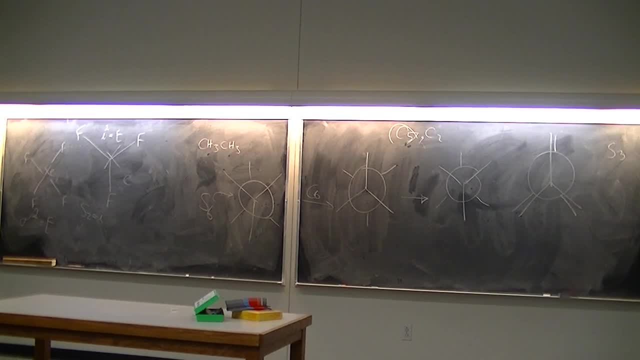 Right, But it is important to discover SM for molecules that don't have CN and don't have sigma H, but they will have them again. Those structures are usually staggered structures- Not usually all the time, But they are usually staggered structures. 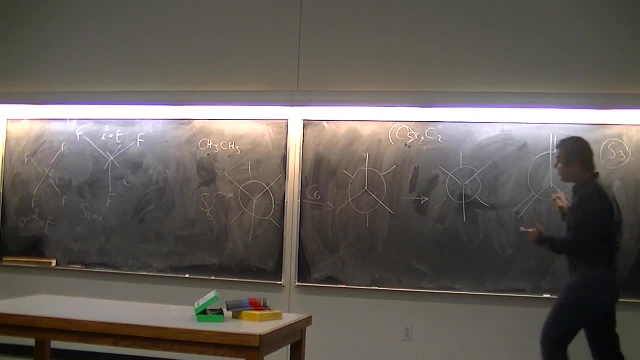 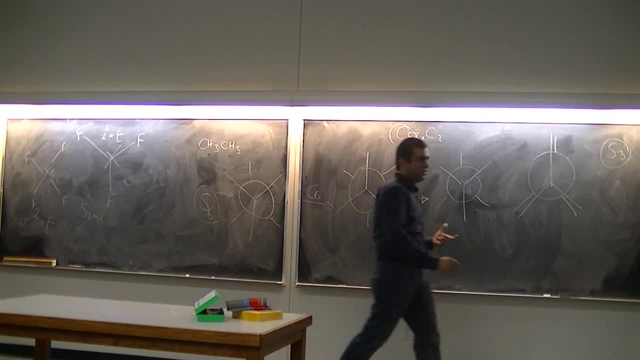 It's a problem. It's a problem. So it is usually staggered structures, not usually all the time. If you have a molecule that has some sort of staggered structure, if you have a structure that looks like this: There's a square on top. 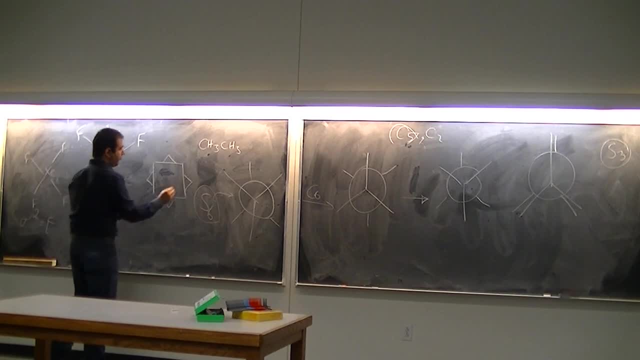 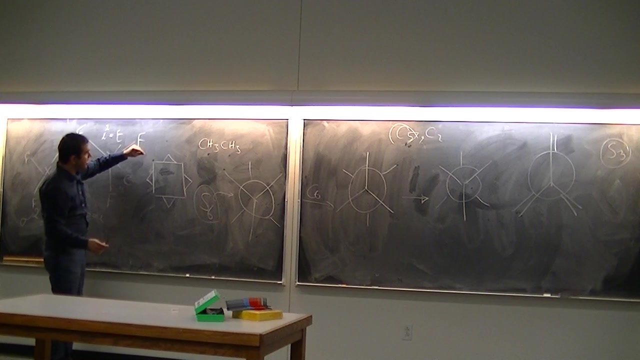 There's another square at the bottom. It has what? S4? S4. Well, it already has C4. It has S8.. If you're on it, it will be C4.. Yes, Yes, eighth of a turn. this in front goes where that is, but that's in the back and 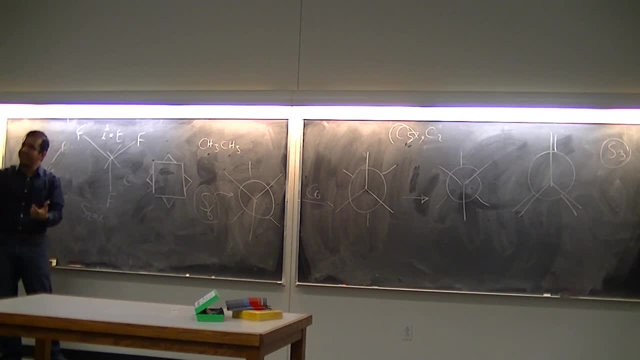 this is in the front, so that that's the cut. that's the other thing, much kind of work together. the CN brings this in the top on in front of work, where that is, and the Sigma is just sends it back. right, that's, that's what this, and so if 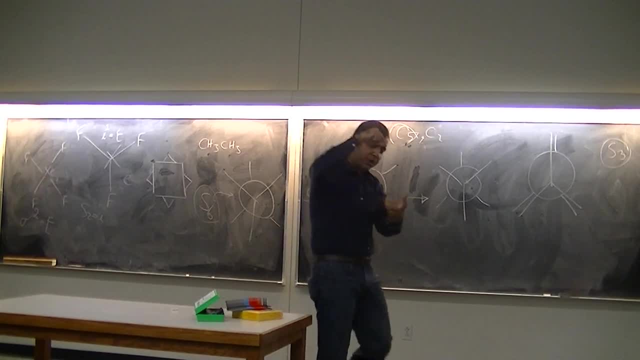 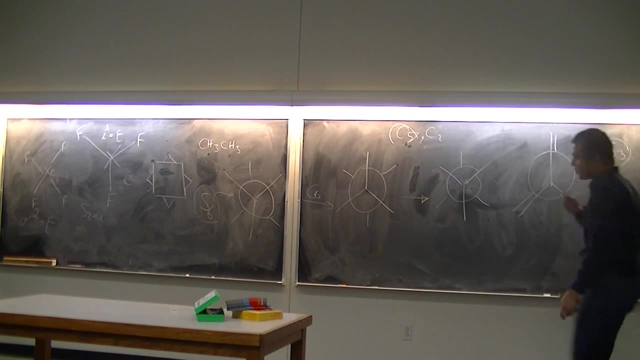 you think of the sphere. if you rotate a little bit and go from up to bottom, that's SN. so it's difficult to imagine, but that's what it does. if you can have some sort of understanding what that SN does, then it's easier to find it you. 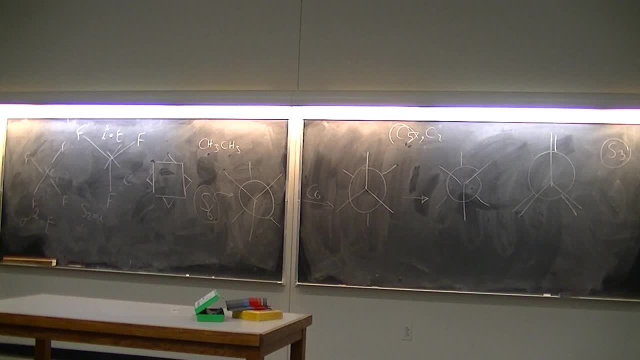 notice: the end is just rotation. Sigma is reflection. it's just rotation and reflection. okay, oh, and now you probably understand why. as to this I because, as to think of a sphere, if you use as s2, what do you do? you do c2, Sigma, H, right. so what is c2? how many degrees? 180, 100? so if you think of a 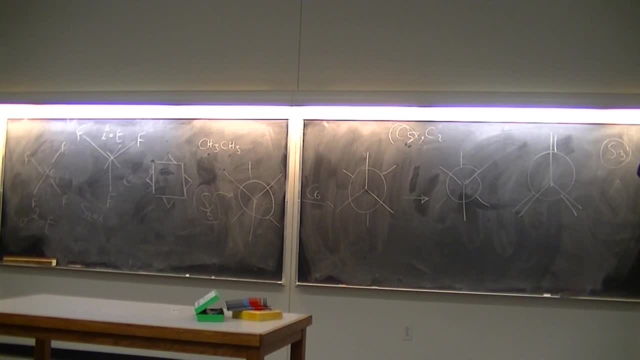 sphere, like. think of United States, like, I don't know, Texas. if you rotate it 180 and then go from up, from north to south, is it not the other side of earth? so s2 180 and Sigma H is actually I. you got it okay, all right. any questions about these? 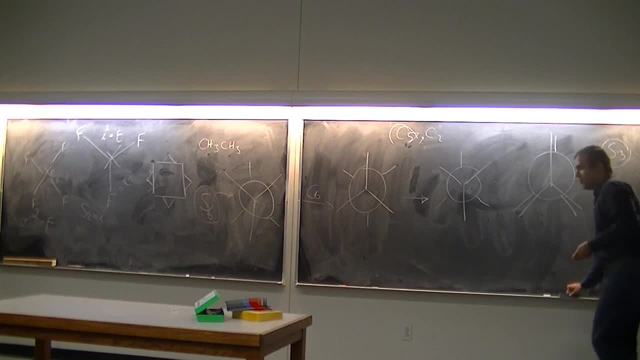 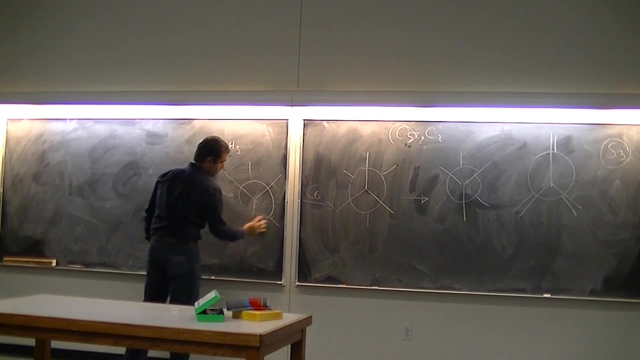 you, are you seeing these? you're good with those, right, okay, so let's do point. okay. so for point groups, you have to check whether your molecule is linear or not. if it's linear, right, you just have to adjust it. okay, at this point you make the available tact here. 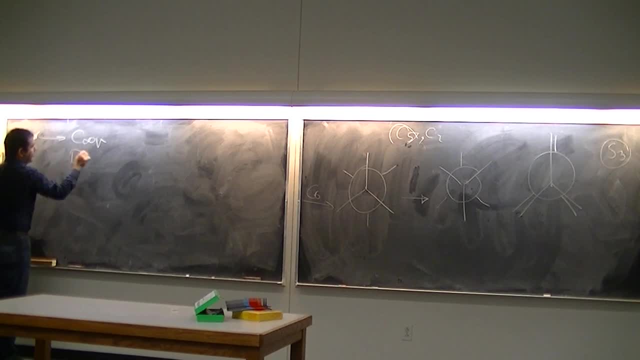 next you have to—so this is your. Yes, it's somewhere. we all know this one. it's c infinite H. if it's not symmetrical, you call it c infinite, okay, Saintser Bay at. it's a symmetrical if it's fn, b or di h. if it's not symmetrical, we call it non-s сколько. we call it c infinite. you call it c infinite, okay. okay, here there, c infinite, there. 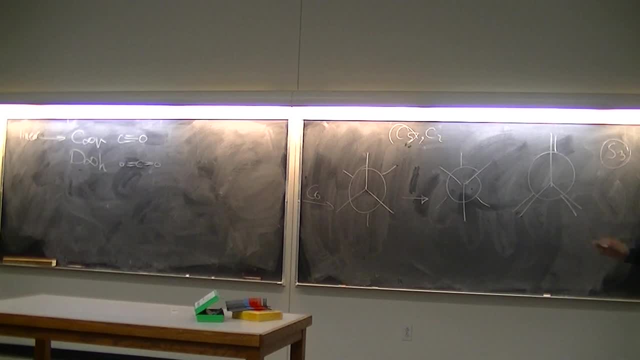 be the infinite, and by the end of the session you know why that is the case. if your molecule is not linear, it could have a different number of highest CN, like what. so, for example, if you think of CH4- right, what does it look like? it's. 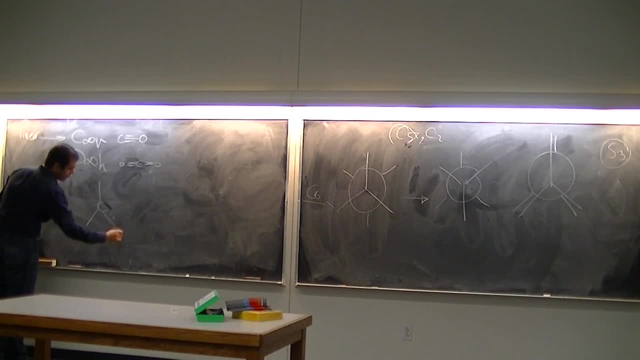 going to look like right. so what is the highest CN hereleret? would you know those angles? C3, right? you said C right. c3, exactly, okay, Although those angles are 109, but their projection on 2D are 120. If you look at this molecule from top, okay. 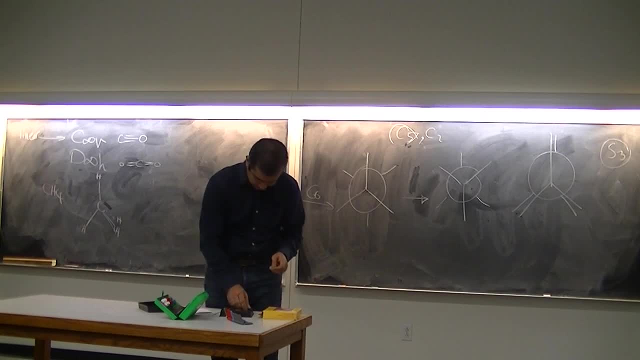 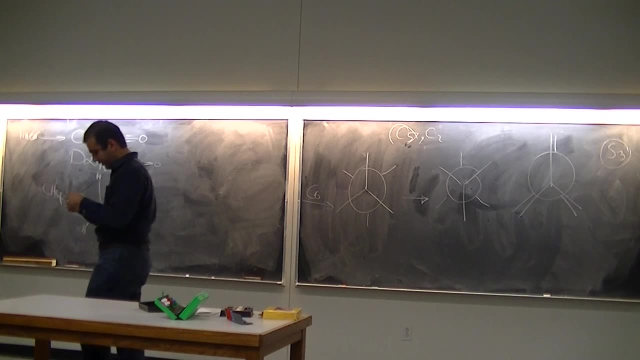 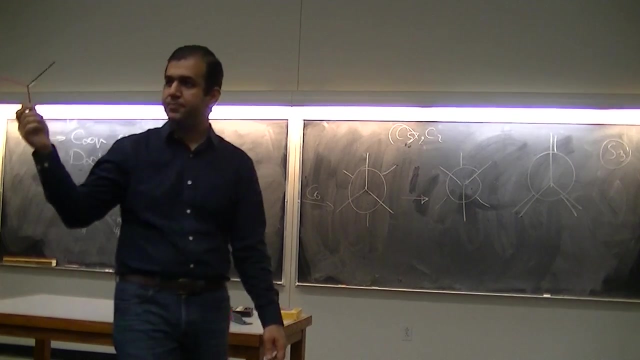 Okay. Okay, I was supposed to take the same color, but Okay. so this is CH3, right. What are those angles? 109.5, right, But if you look at it through one bond, the projection on 2D is 120.. 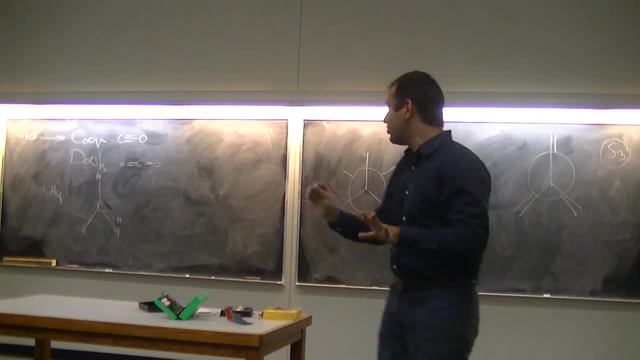 Exactly, it's a triangle right in the back. So don't be so. remember, don't say that, don't you know? sometimes, When you want to think of like a shortcut, you might make a mistake. 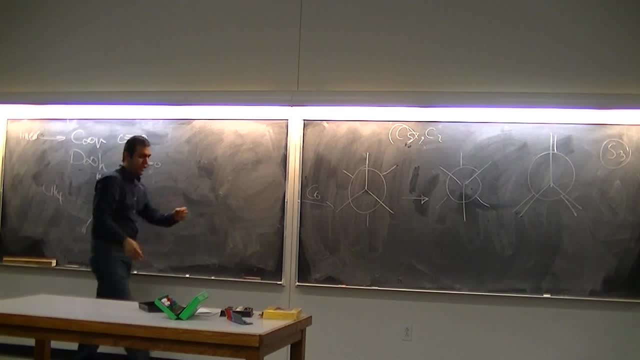 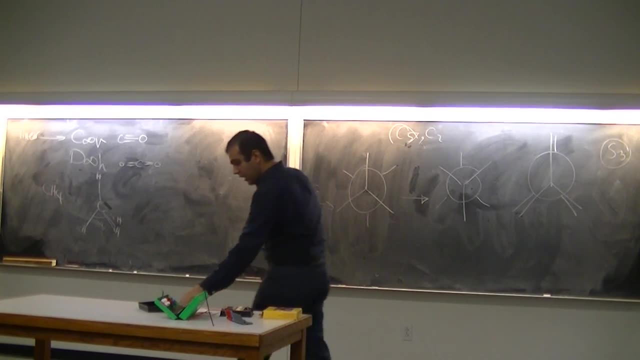 Don't say that this angle is 109, so it cannot have a C3. You have to look at the projection on 2D and it has a. you all see it right: it has a C3. So, but how many C3s does it have? 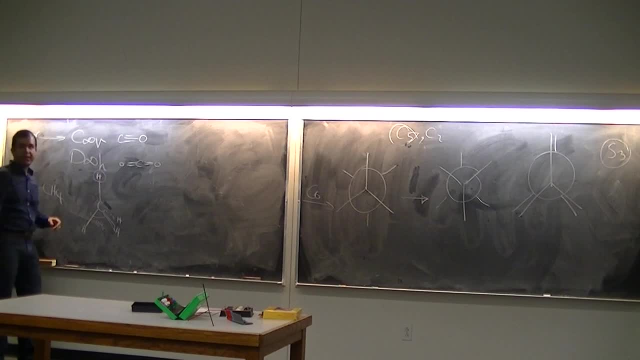 What did you do to make a C3? You picked any hydrogen with the carbon and it gives you one C3, right. So why not going into the other carbon hydrogen? How many hydrogens do we have? Four, Four, So we can make four C3s, right. 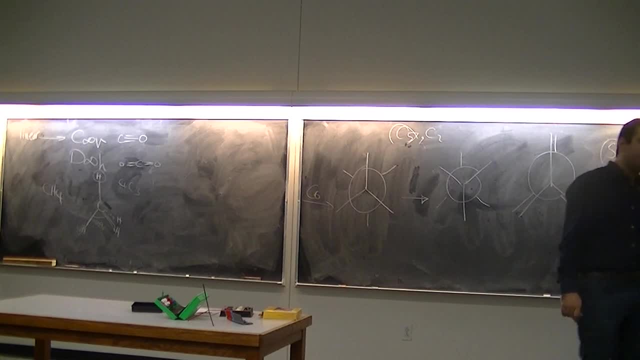 This. in this case you have multiple Cn's with higher, highest order okay, And these are usually very easy to pick. These are either tetrahedral or octahedral And usually by just looking at it you can tell which one it is. 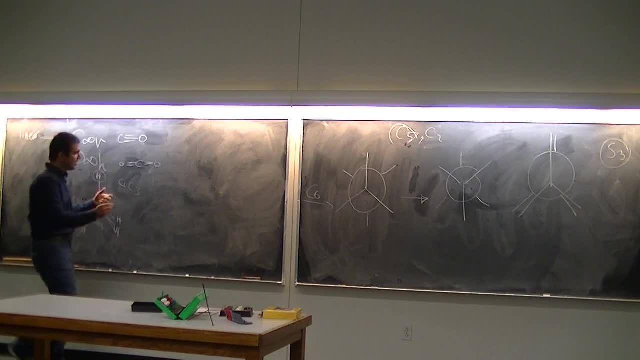 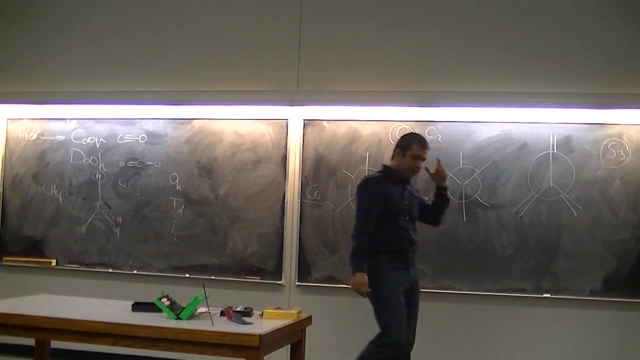 So the if you have multiple highest Cn's, your point groups are either octahedral, octahedral, tetrahedral or ith, I guess Right, And these are usually easy to pick up: If you have, I, if you don't have I it's tetrahedral. 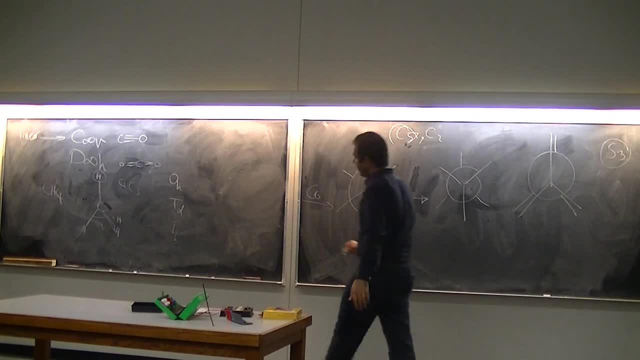 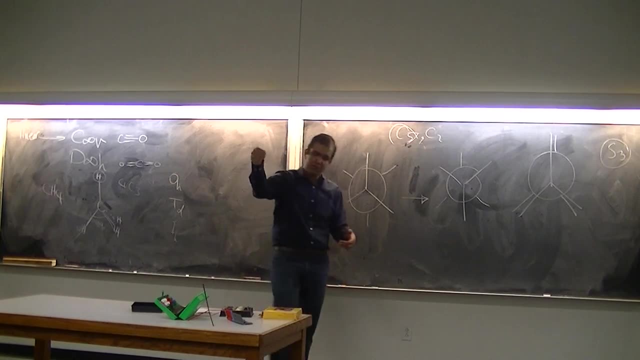 If you have, I, it's either octahedral or hypotahedral And the difference is C5. Octahedral does not have C5. But go through that chart. I guess it's easier to memorize. Right, I'm going to spend most of my time. 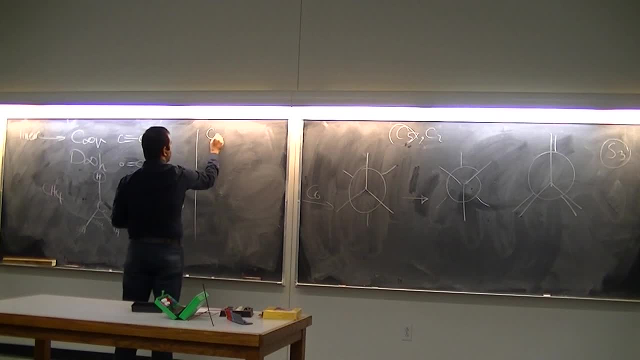 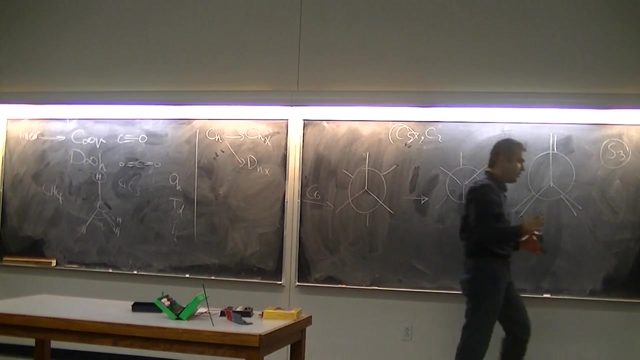 for molecules that only have one Cn: okay. These That only have one highest Cn are either Cn something or Dn something. Okay, And most of the molecules that you will be given are from that time. Okay, Once you figure out the highest. 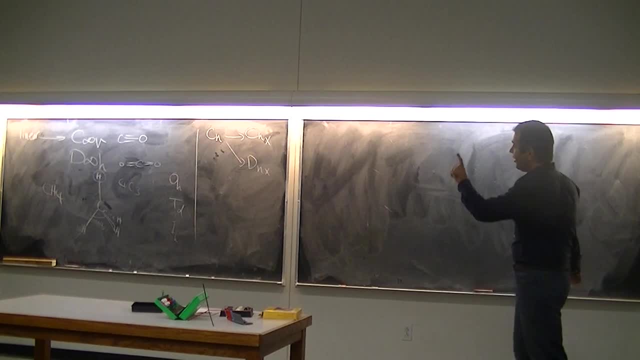 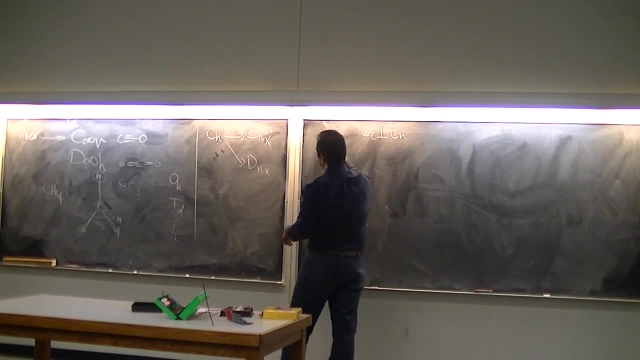 so what do you have to do to get the point group? First, find the highest Cn. And what is the next, The next step? check for C2s that are perpendicular to the Cn that you just identified. Okay, Look for what? 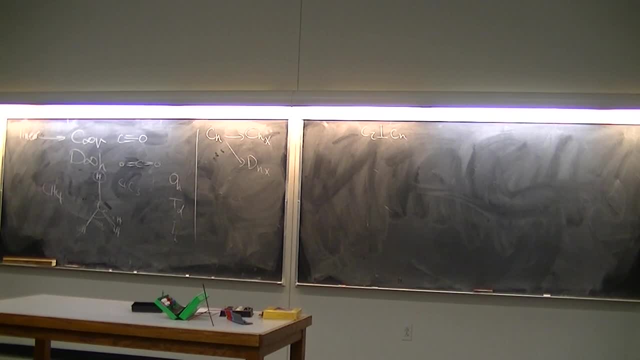 C2. that is perpendicular to the highest Cn that you just identified And remember you are supposed to have only one Cn, So there should be no confusion of which Cn to take. If you have multiple Cn's, you are not here. 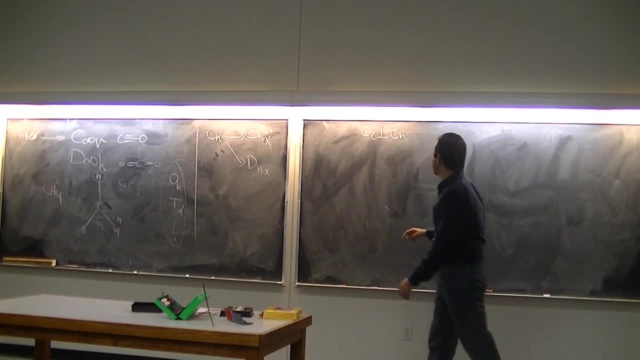 You are here. If you have one Cn, you are here. So you look for C2s that are perpendicular to your Cn. So you look at your Cn and you think of what like axis could be perpendicular to that. 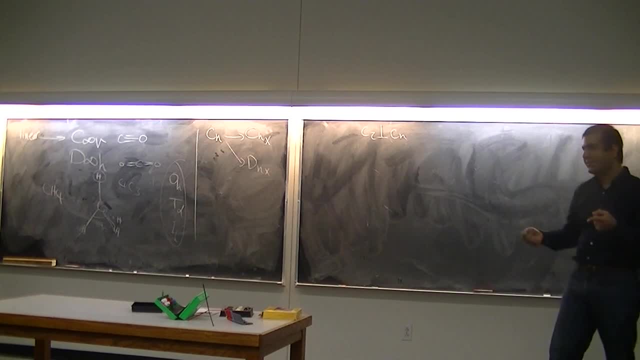 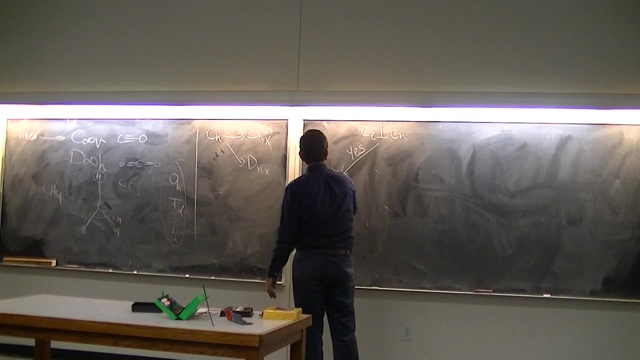 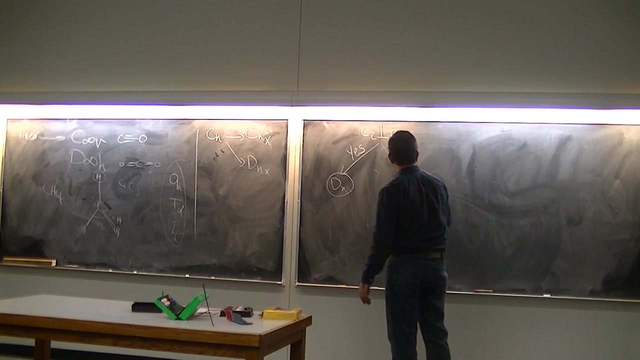 And you look and see whether any of those axes are C2. If you have perpendicular C2, then you are in the Dn family, Okay, Dn. If you don't have, you are in the Cn family, Okay. 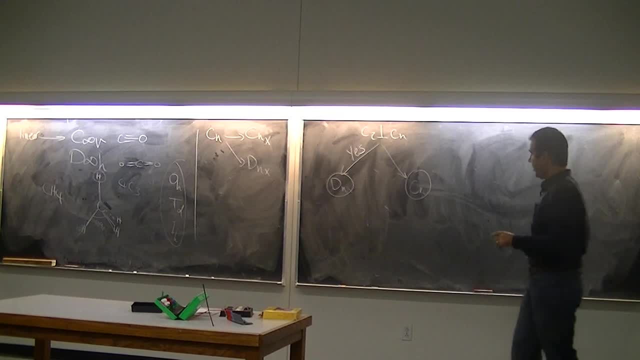 Okay, Let's see E, F3.. What is the highest Cn? C1.. Quite obvious, C3.. Louder, I can't hear you. C3. C3.. So C3, and how many C3s do I have? 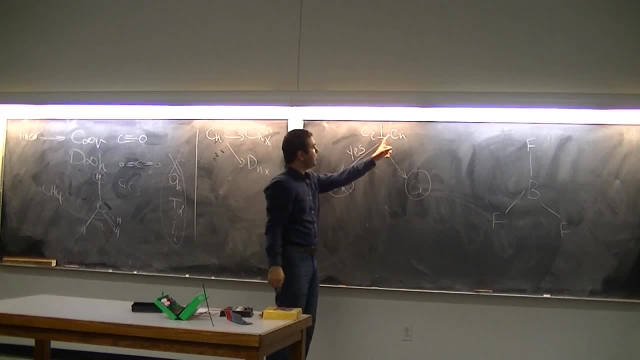 One, Only one. So I'm not here. I'm here. What is the next thing to check? Perpendicular C2s. So my C3 is there, right, Just there, Right, Perpendicular to this board. So the C2s, if they are there, they should be perpendicular to that. 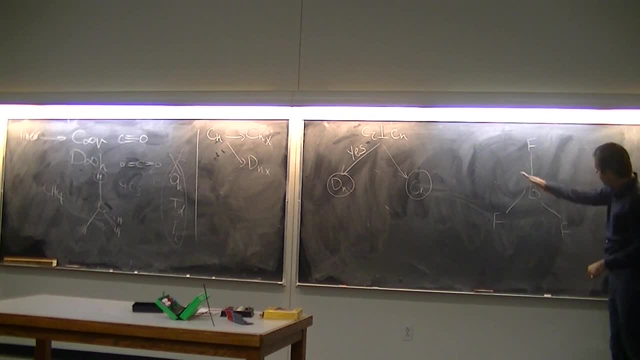 So I should be looking on possible C2s kind of parallel to the plane of the board. Okay, Is there any? Is there any perpendicular C2?? Yes, Yes, This is a perpendicular C2.. This is a perpendicular C2.. 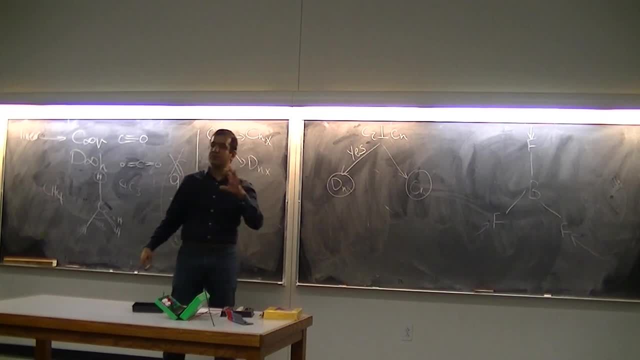 And this is a perpendicular C2.. So that molecule is from the dn family, It's dn something. And how do I know whether it's dn something? The next thing that you have to check here is sigma H. You have to see whether there is a. 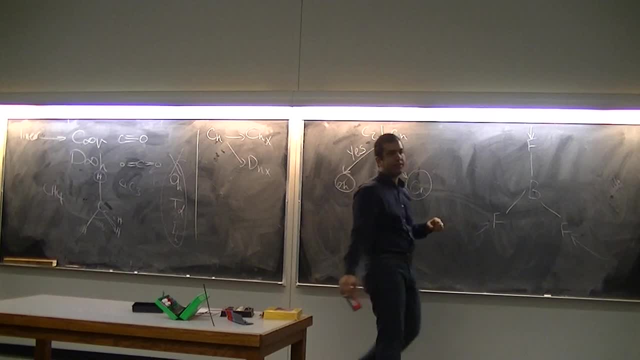 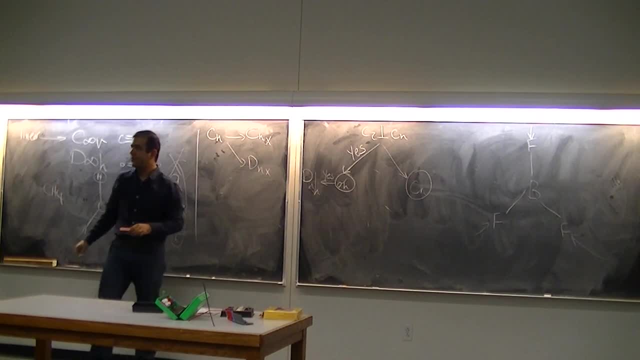 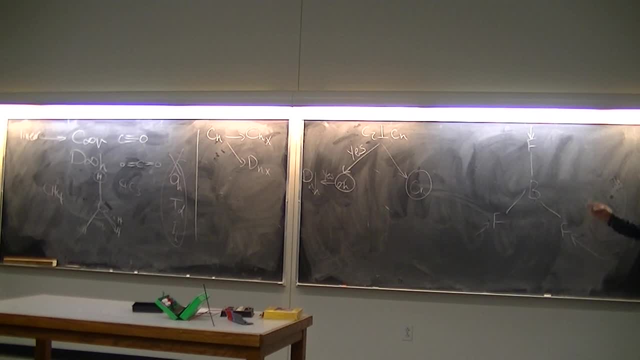 So I'm in the dn family. Is there a sigma that is perpendicular to the Cn? Yes, Yes, It's there. right, It's the plane of the voice. So the answer here is yes. So this molecule is what? 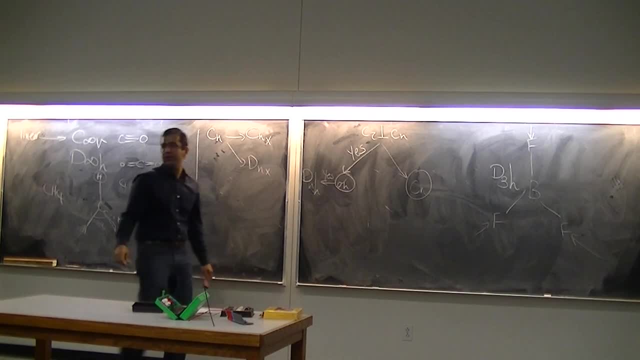 B3H. Okay, Now if I take the same molecule and replace the fluorine by hydrogen, does it still have the C3?? Yes, Yes, The C3 is still there. If I rotate it 120, it's still there. 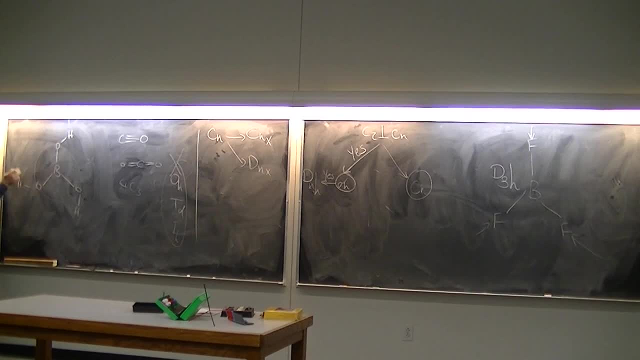 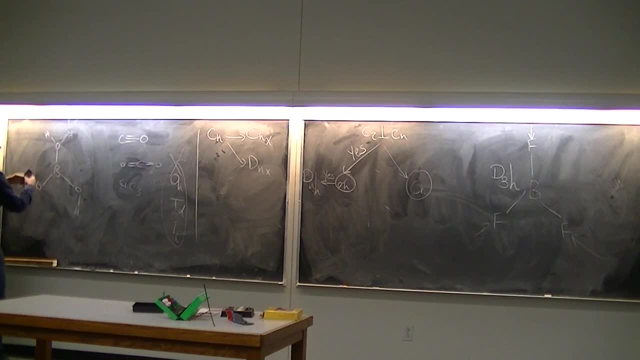 So the angles are also important, But the way I draw it, it still keeps the C3. All right, Okay, Does it keep the perpendicular C2 that it used to have in the case of VF3? No, Yes, No, it doesn't. 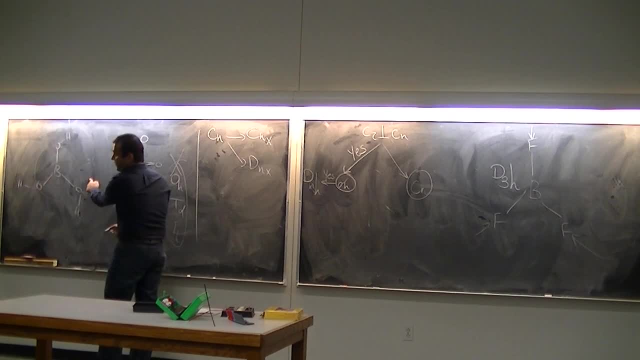 It doesn't. It doesn't Because if you apply the, If you apply the same C2, this hydrogen will flip over here, right where there is nothing. So it keeps the C3, but it kills the C2, okay. 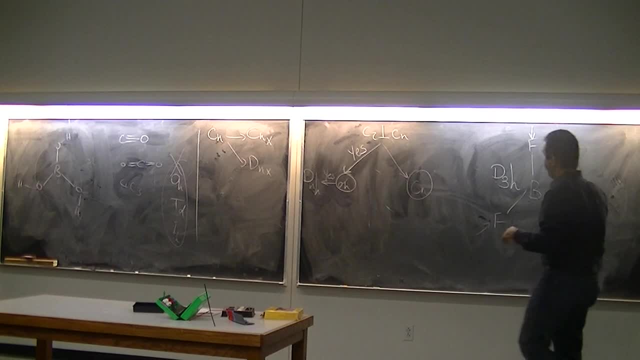 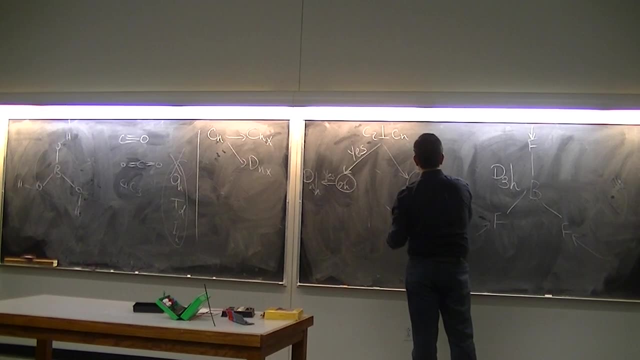 You all see it: The C3 is gone, but the C2 is still there. So you are in the Cn family. and the same thing you have to do here: You have to check for sigmoids. If you have it, then your answer is CnH. 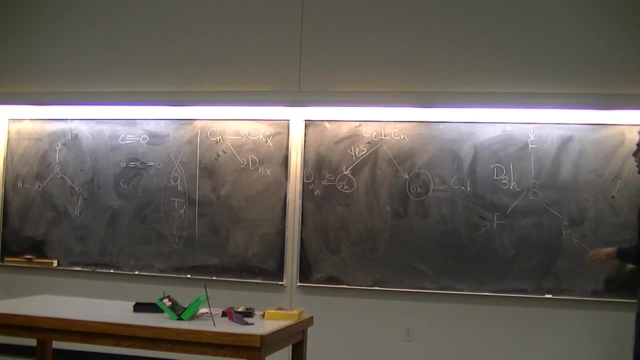 So I'm in the Cn family because of perpendicular C2.. Okay, So the C3 C2 is gone. Do I have a perpendicular plane? Do I have a horizontal plane? That molecule Is it still flat? It is, So it keeps the sigmoids. 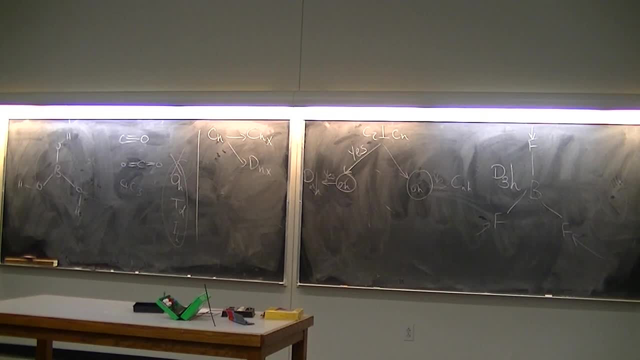 So the answer here is yes. Yes, so here, this molecule is what? C3H. Okay, All right, let me tell you something to make it easy to analyze. What is the point group of this? What is the point group of this? 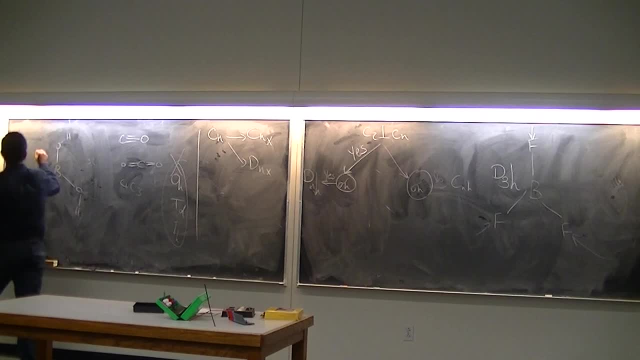 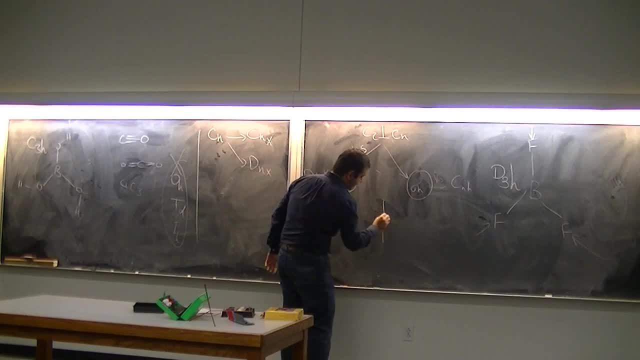 Is it the C3H? Is it the C3H? Is it the C3H? Come on guys, quickly. What is the highest? C5?? Does it have perpendicular C2?? Yes, Does it have the plane horizontal plane? 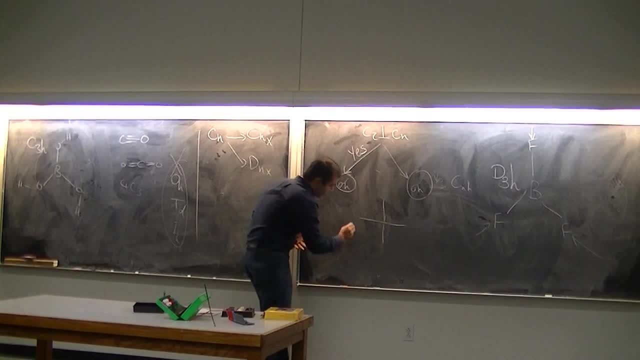 So it's what D4H, D4H. Very good, Does it look familiar, Right? So what do these tails do? You can memorize it this way: Hitler C2, okay, That's why they lost the battle to Russia. There was some perpendicular C2 somewhere. yeah, messed it up, So remember if you have. 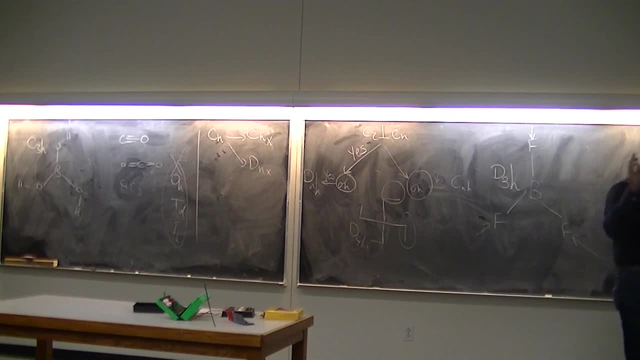 Hitler, there's no perpendicular C2, okay, Tails kill the-. no, really, it makes it simple: Tails kill the perpendicular C2, but if it's still flat, the signal axis is still there. okay, And sometimes you can model your molecule with that shape. 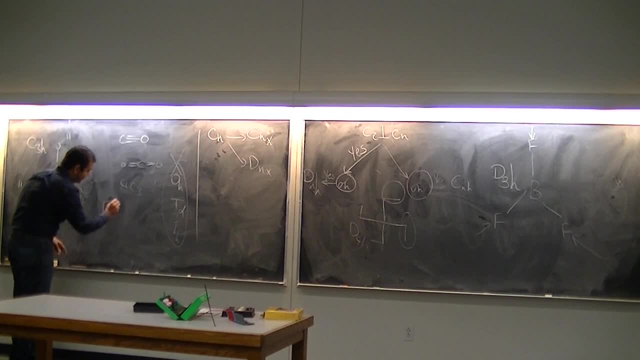 Okay, one of the molecules that people love to give for symmetry is this: right? If I want to simplify this molecule, right? Can I draw it this way? Because of the nitrogens. if you think of nitrogens as some sort of tail, this is C2H. 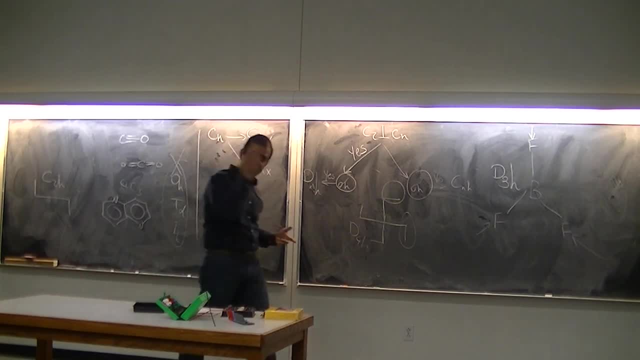 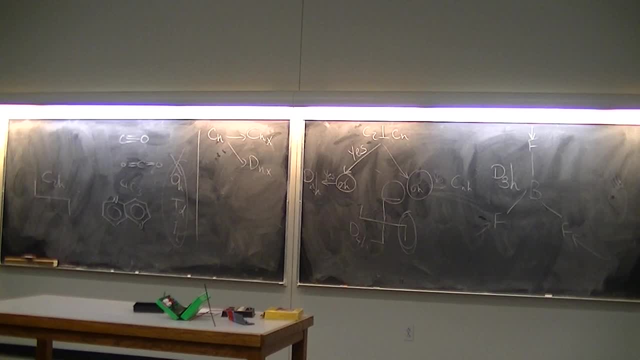 If it's still flat, the signal axis is still there, but if it's not flat, the signal axis is also gone. Alright, any questions about DnH and CnH? Okay, what if the answer is no? What if there's no perpendicular? Then you have to check-. 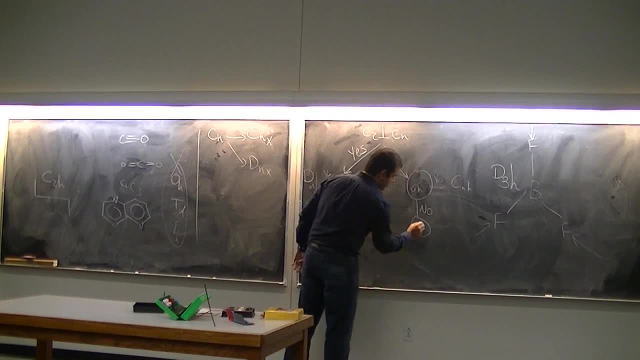 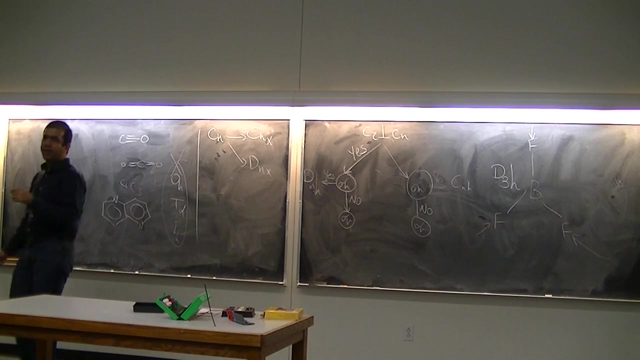 For sigma B, And by sigma B I mean your table might talk about sigma D or sigma B, Assume that they are both the same. By sigma D and B I mean a sigma that is parallel to the CnH. Okay. Now, if there's no sigma H, then you check for what Sigma B? If the answer is yes, what is it called? 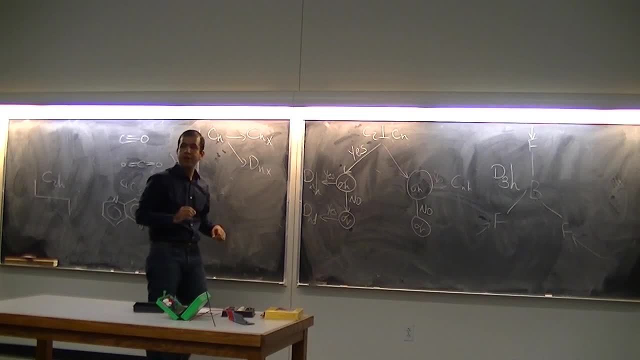 DnD, Right, And if here the answer is yes, it's CnD, Alright, Just guys, quickly, what is this? Okay, wait a minute. So DnD, Okay, Yeah, ZH3ZH3.. What is the highest Cn? 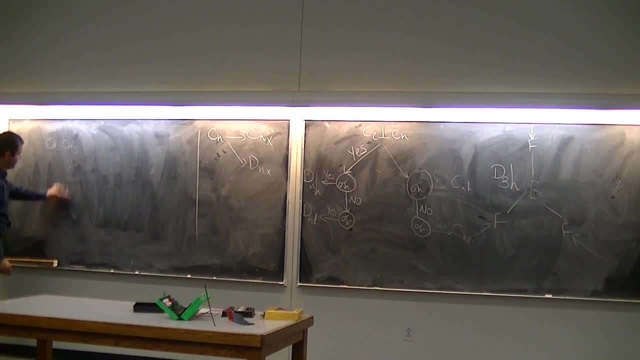 Oh, okay, No, Not this one. So there are two squares on top of each other and they are off Like they are not. it's not eclipsed. What is the highest? Cn? C4. C4. All agree. 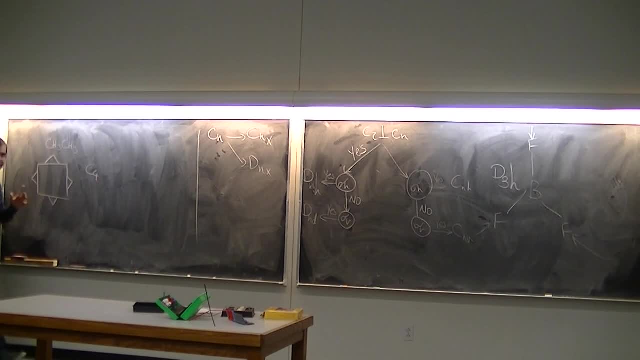 Yeah, This is. it has C4. What is the next? So one thing that you should be careful: Don't try to extract all those symmetry elements from what you see. Look at what the chart is asking at the time. Okay, So don't say to yourself: it has C4, it has C2, it has sigma, it might have I. 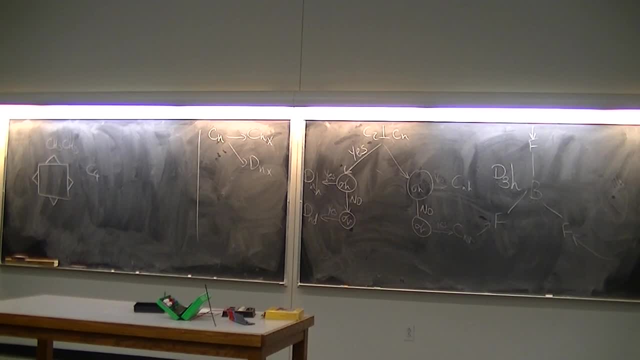 Don't do that, Just follow the chart. Okay, What is the next thing to check? If there is perpendicular C2.. If there is perpendicular C2.. Is there any perpendicular C2 here or no? So since C4 is here, I'm looking for a C2. that looks like that, right. 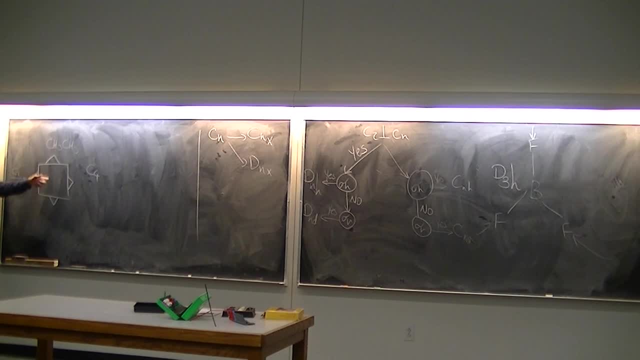 No, No, it's not there, because if you apply, what will happen to this? if you apply this, This will rotate the back. so that, so this one- let me talk about this first- It will rotate it and turn it and send it to the back right. 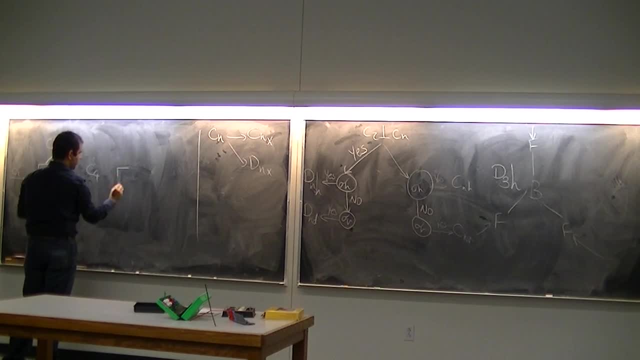 So it will look like. it will look like this, Because this used to be here and just goes to the back, And that one that. so this one used to be in front right With the C2. it just goes to the back, Okay. 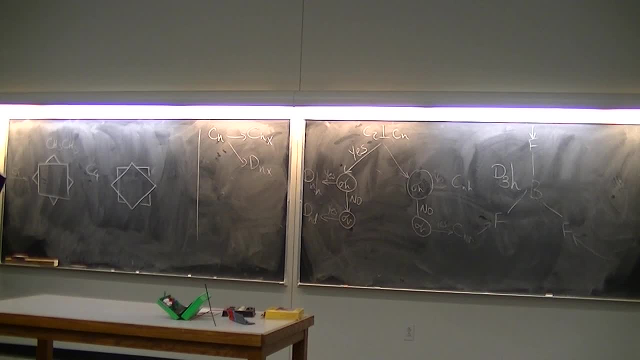 And that one was in the back, but with the C2 it just comes to the front, So you have a like tilted square in front and a vertical square in the back. Is it clear? So it does not have the C2, right? 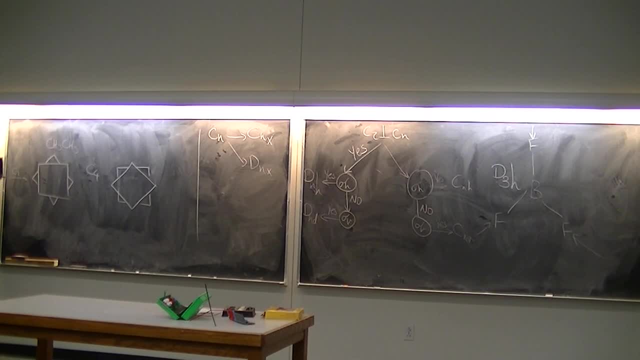 So we are in the Cn family, right, Right? No, it does have perpendicular C2.. Okay, It's difficult to see, but it's there. Alright, guys, Don't try to see it, Just trust me, It's there. 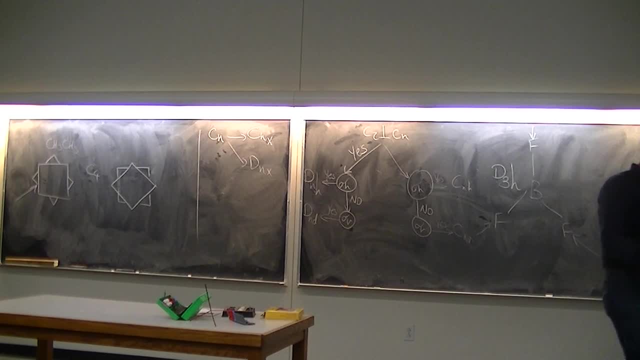 If you have similar shapes on the top and bottom of your molecule with respect to your Cn, Try to digest what I'm saying. It might- you might not get it in the first time- What I mean by top and bottom. I'm talking about it with respect to your Cn. 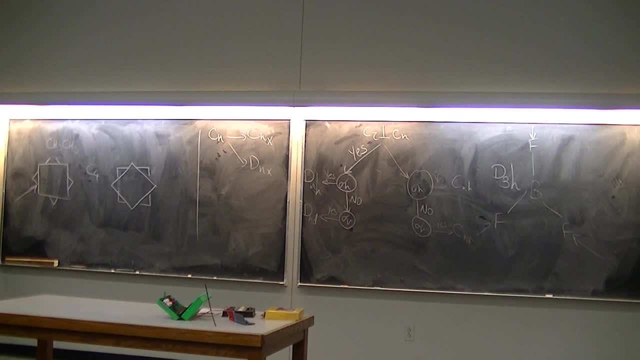 So when I say top and bottom, I'm not talking about here and here With respect to Cn. Your Cn was there, right? So top is the front square, bottom is the back square. Okay, If you have similar shapes from the same size and from the same element on top and bottom. 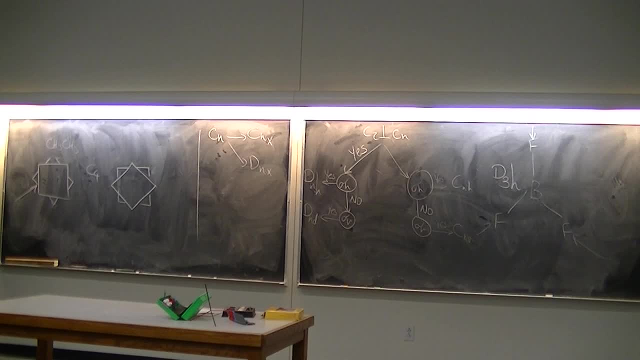 it doesn't matter what angle they have with respect to one another. You always have perpendicular C2.. Okay, Just memorize it, Don't try to see it. Okay, Trust me And decide if it's. this is what I was saying yesterday. 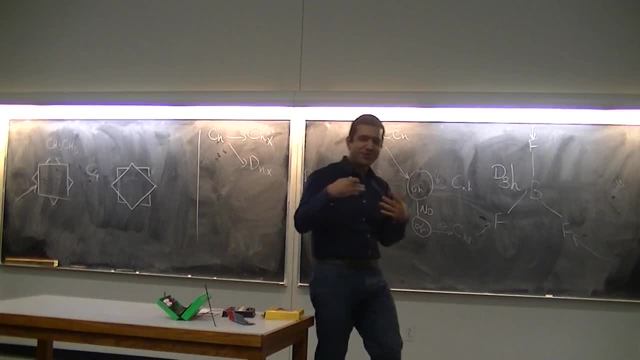 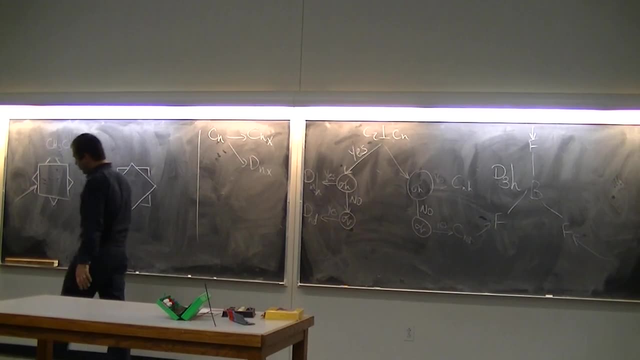 If what I'm saying is wrong, don't worry, I am always going to grade those So you will get full credit anyways. Okay, So trust me, If you have a square at the top, goes to the square. Remember, I'm not talking about a case where you have fluorine here and fluorine in the back. 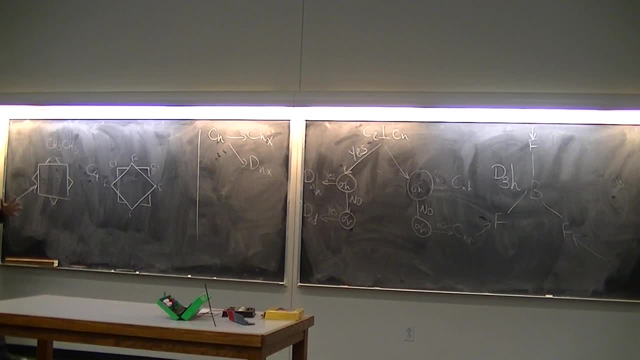 If they are similar, and by similar I mean exactly similar. Same element, same size. Not if you have a square in the front and a triangle in the back, Similar shapes In top and bottom, you always have perpendicular C2.. Okay, 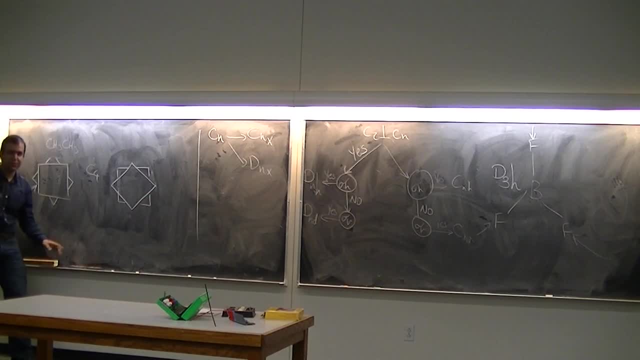 Don't again. don't try to see it, because you won't see it And you will go to the Cn family. Just trust me. These are all the n something. So Do we have perpendicular C2 here? Yes, 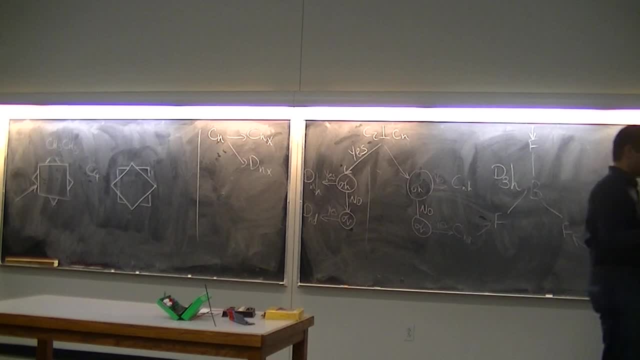 So we are here. Does it have sigma H? Is there any? is the plane of the board a sigma for this molecule? No, No, it's not, because it will send this one. It will actually do the same thing. It will send this one in the back and will bring that around back and front. 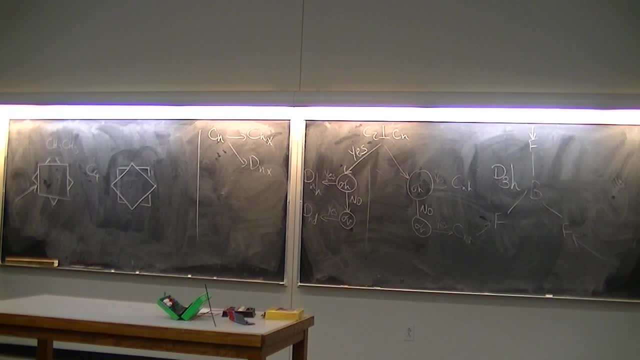 This is where perpendicular C2 and sigma You probably It's easier to see the difference between perpendicular C2 and sigma. Sigma will just bring it from back to front, So this one will just come in front, But perpendicular C2, by rotation, does it. 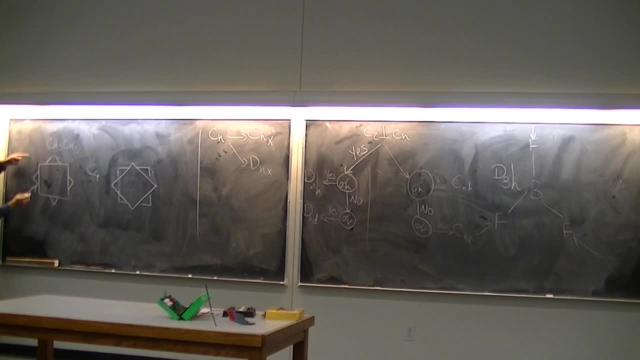 So if you do perpendicular C2,, for example, this one will go in the back. It just, you know, rotates 190. So from top it goes to the bottom, But reflection just does not change top and bottom Just force it to go from back to front and from front to back. 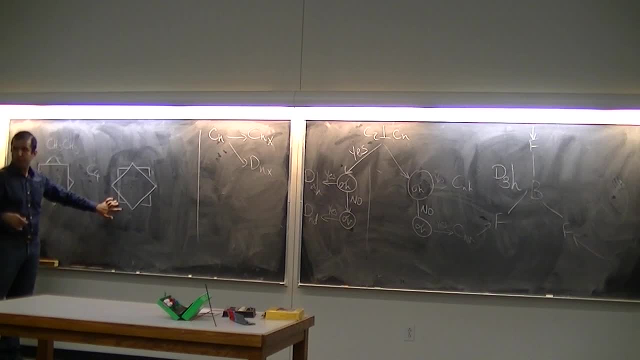 So is there any sigma H? No, right, Because if you apply sigma H, this is square from front, It will go in the back, It will look like that and it is not the same. So the answer here is what? No? 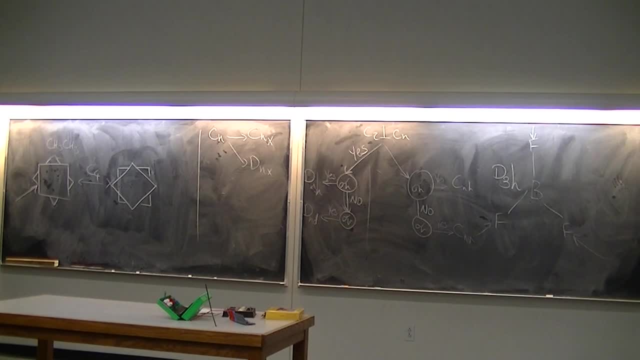 Am I confusing you? Why can't we see the C2?? Why, I'm still trying to figure out the C2.. Oh, okay, It's actually there If you rotate this 180.. Where does it go In the back? 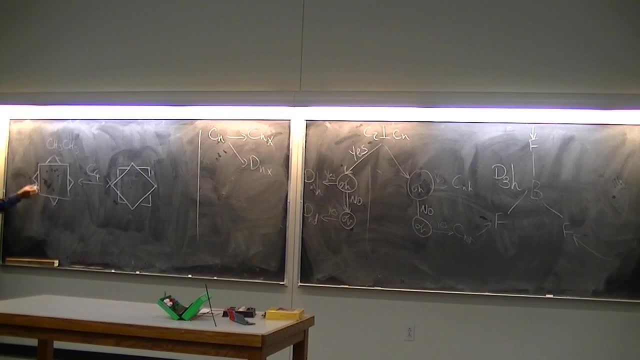 So by applying: this goes there, This goes here, This goes here And this goes here. It is easier if you try to see it. If you see it, it's easier to see it in a triangle. The first C2 that comes to mind is where 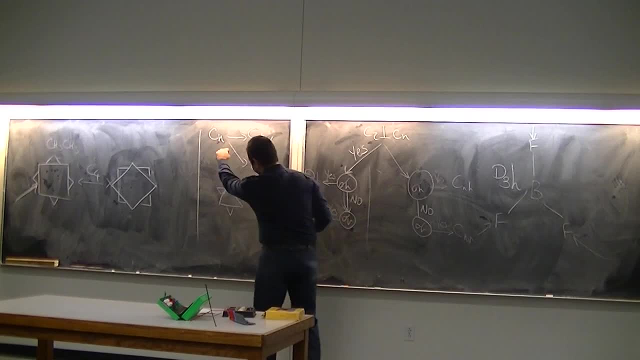 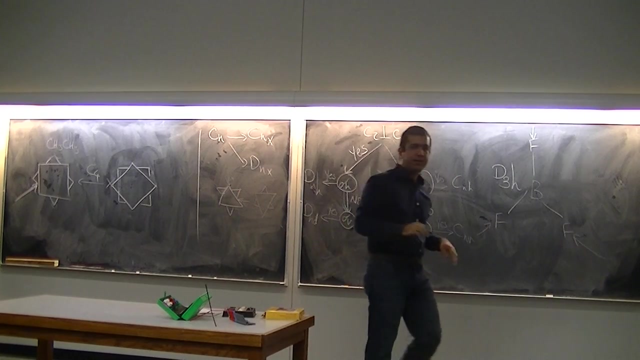 Which is not the case. If you rotate it by 180 through there, this triangle will go in the back, So the one that is pointing up will be in the back. So it's going to look like that, Right, But if you apply it this way, let me see it. 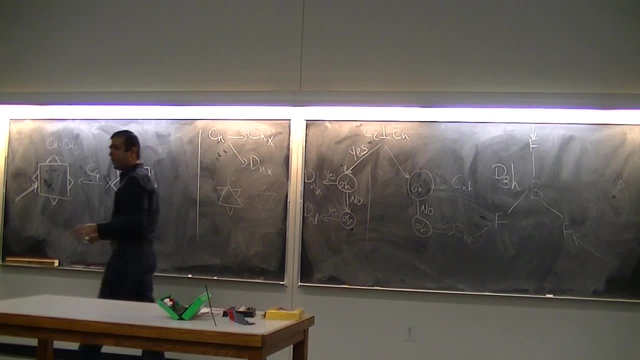 So there is a C2.. Trust me, guys, It's there. Okay, All right. Yeah, So how many C2s are there? Oh, this is the other point. Is it eight? No, you have four. You either don't have any perpendicular C2 or you have n of them, depending on what your. 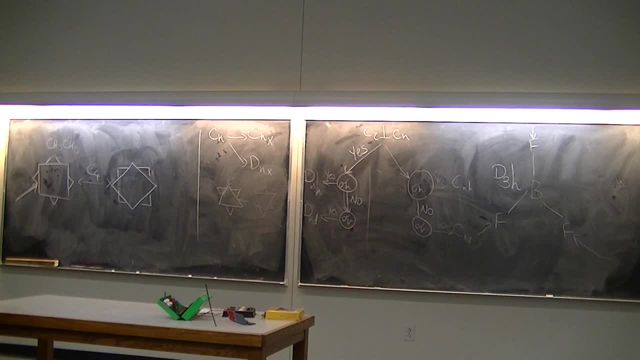 Cn is All right. So I know your chart asks you to check for n perpendicular C2,, but just look for one. You either don't have it or you will have enough. Okay, If you have a C5, you cannot have three C2s. 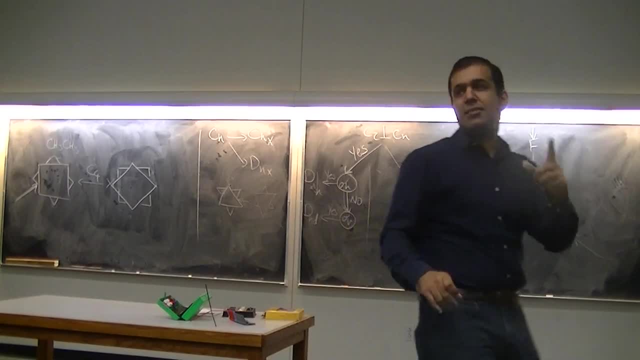 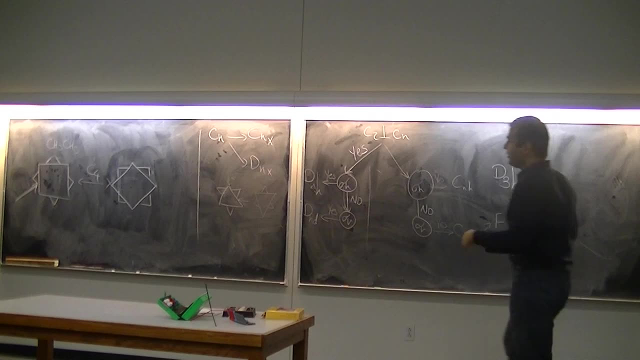 You either have no C2 or five C2s- Okay, So just look for one. The same is true for sigma v. I'll get to that. You either don't have any sigma v or you will have five of them Or n of them. whatever you are having. 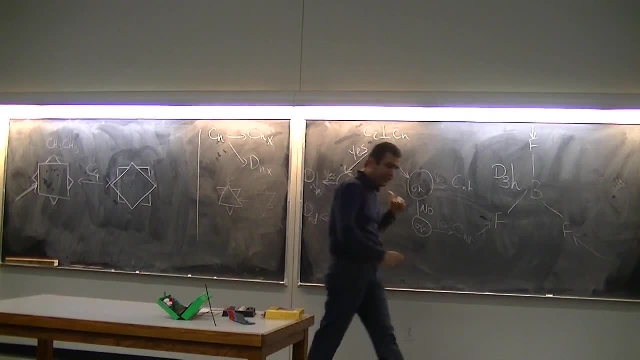 Okay, So we are in the dn family And we said that this molecule does not have sigma right, Right, I don't know what silence means, but right, Yes, Yes, Okay. Does it have sigma v? Is there any sigma that is parallel to your Cn? 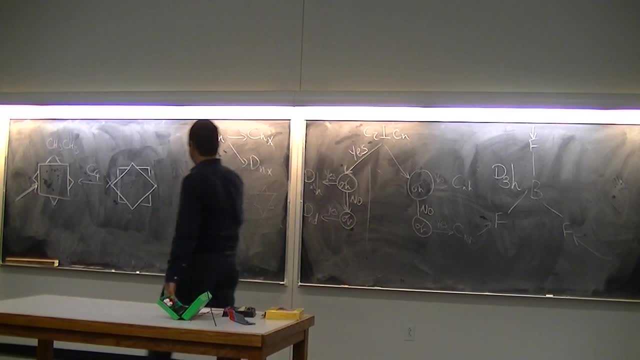 Yes, Yes, It's right there, Which one? If you can think of this Right, You'll reflect that to that. So remember, when you write your molecule in such a way that Cn is perpendicular- you know, is perpendicular- to the plane of the board, sigma h sends back to front and front. 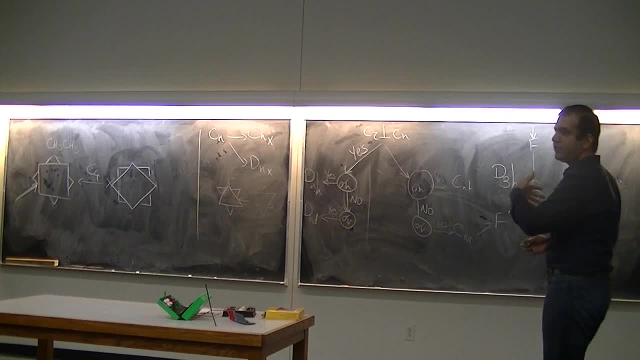 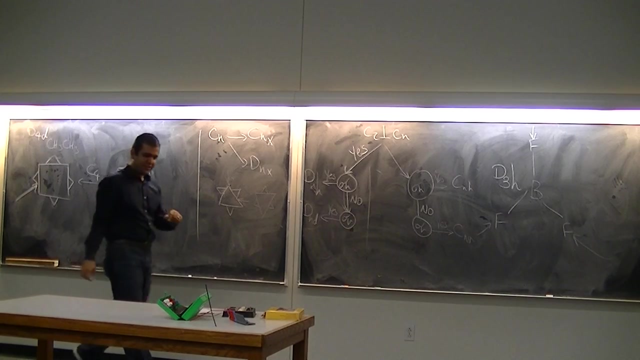 to back, But sigma v usually sends left to right and right to left. Okay, So your molecule is what? DnD? This is Z4D. Okay, So what is ethane? Come on guys. Ethane, Main principal axis, is what? 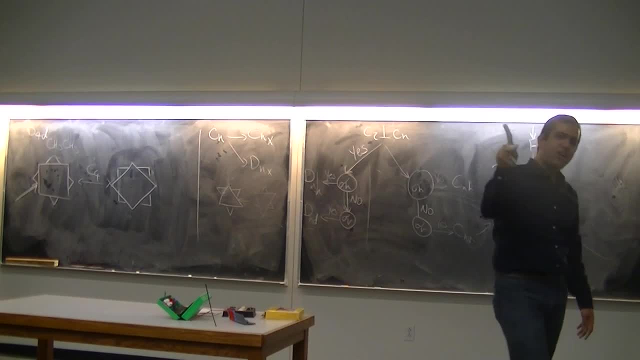 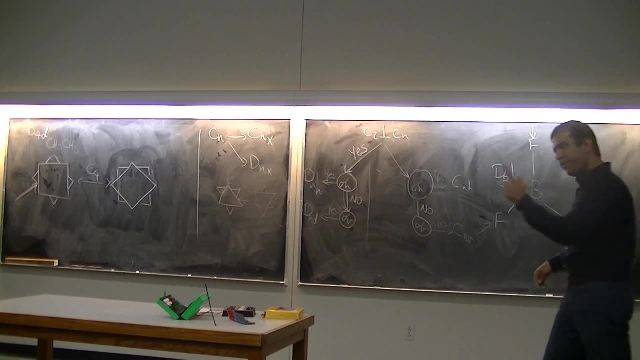 C3, right, The structure, that you have a triangle of hydrogen in front. You have a triangle of hydrogen in the back. Don't worry, There is a perpendicular. Okay, Yeah, D3D, It will be D3D. 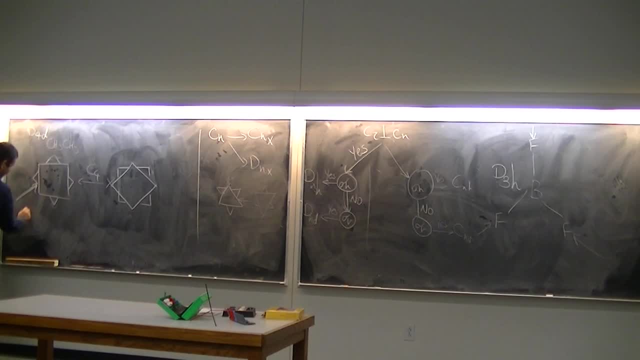 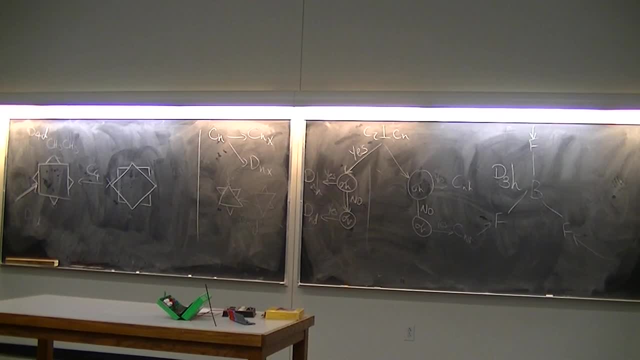 Yeah Well, let's not worry about that. So okay, Guys, quickly Look, Let's do Bn at BnL. Okay, So Cn, Let's go to ammonia. What is the highest order? what is the highest Cn? 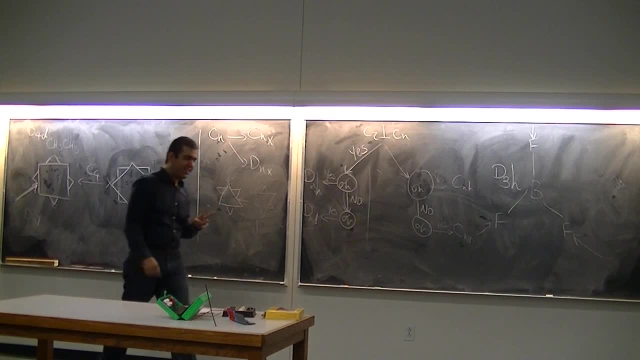 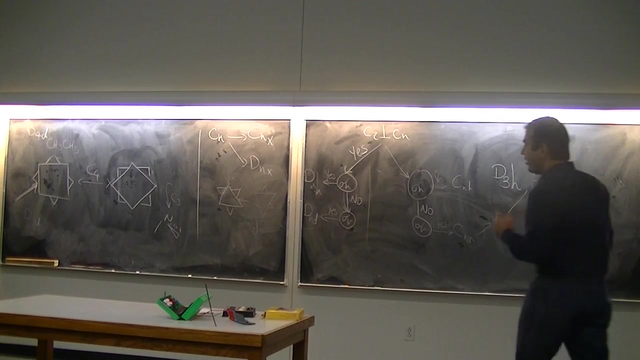 C3. Very good. Does it have perpendicular? Okay, right now. so what is the first thing if you see members with the same size, with the same size for remembering, for remembering similar up and down, you have perpendicular c2, right, you got it. the second thing to write: if up and down of your molecule was completely different, like here you 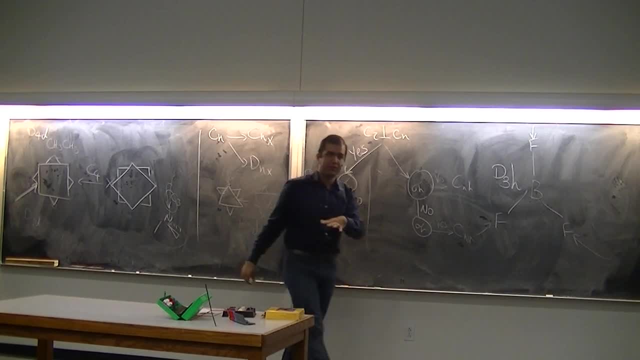 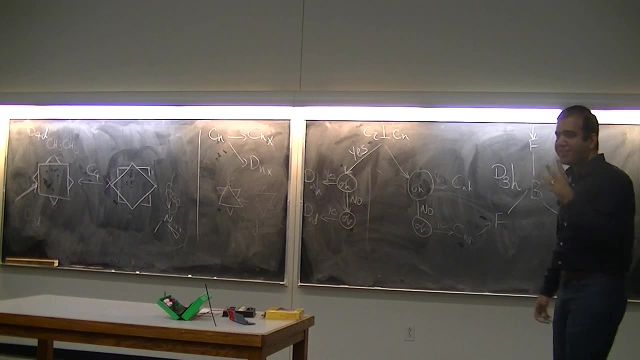 have nothing off, but you have hydrogens in the down, in bottom. okay, you do not have perpendicular c2. you do not have sigma h. okay, because they relate up and down with different mechanisms. your up and down is different. there's no sigma, there's no perpendicular c2. 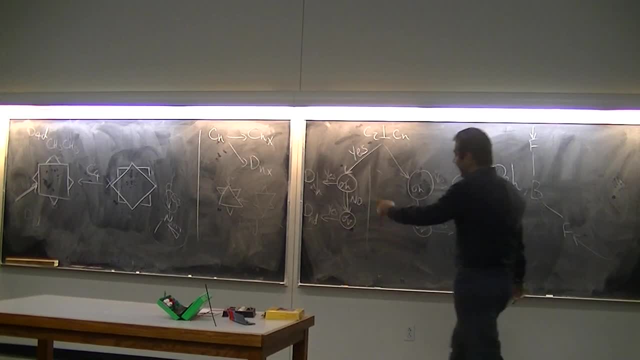 okay, don't try to see it. okay, so it has c3. does it have perpendicular c2? how do you answer that question? you say up and down is different, so there's no perpendicular c2. okay, you go here and there's no sigma. so you kind of jump, you come here, okay. 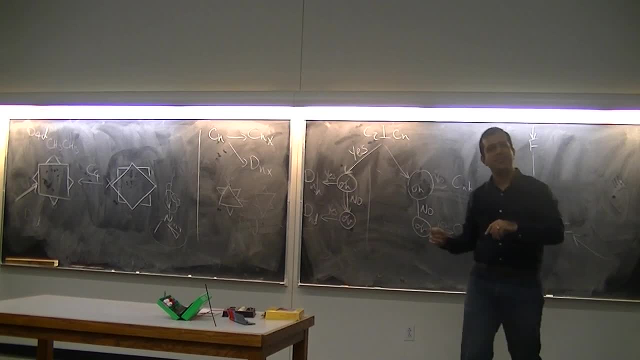 up and down. is there a question? yeah, what is it? oh, you were on your own, doesn't that molecule, the bf3? also not with respect to cn. where is your cn? yeah, up and down is the same nothing, oh, okay. yeah, up and down with respect to cn, if they are. 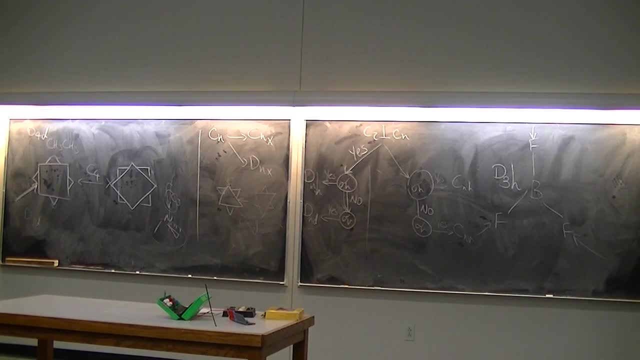 different. there is no perpendicular c2, there is no sigma. okay, so this one- it has a c3 up and down- is different. there's no perpendicular c2, there's no sigma, so you directly jump there. is there a sigma b? is there a sigma that is parallel to cn? yes, yes, it's there. 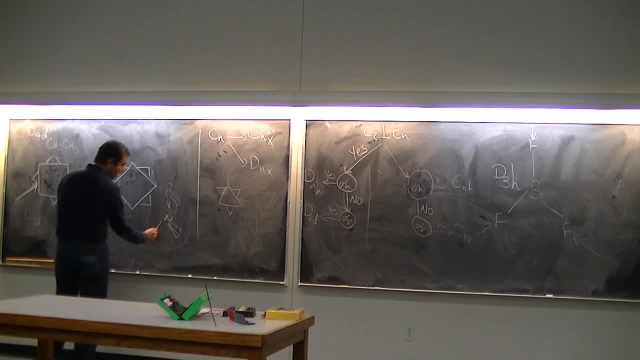 it's plane of the board, so it's a plane that goes through this nitrogen and this hydrogen. so remember, there's not one nitrogen here, one hydrogen here and two other hydrogens here and there, right? so if you have a plane like that, it could reflect, reflect the two hydrogens and go. 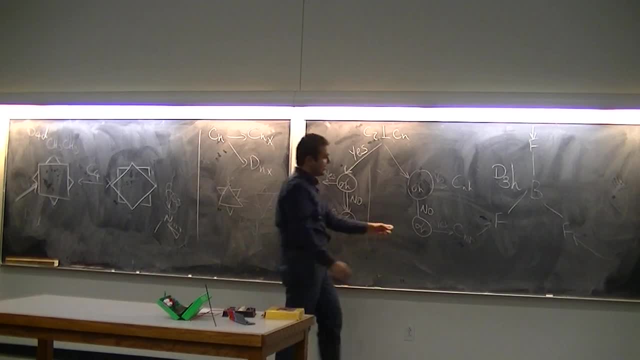 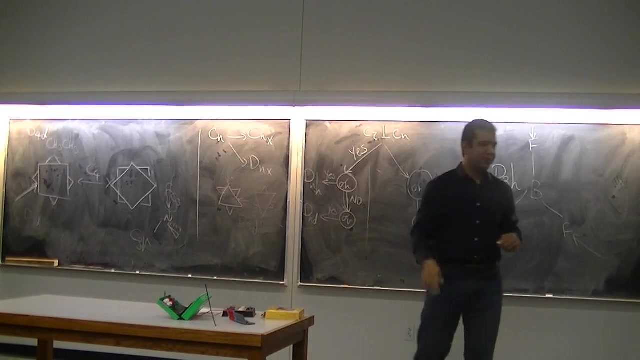 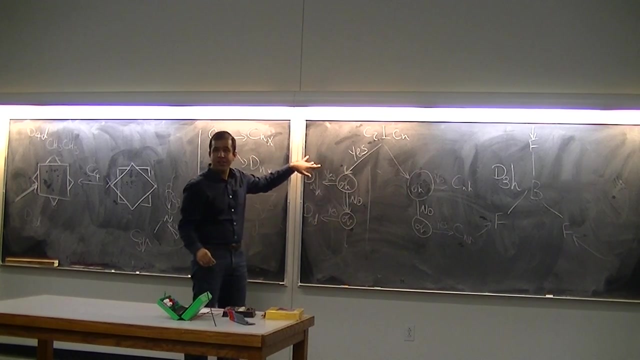 through this hydrogen and this nitrogen. so the answer here is yes. so what is ammonia, c3 v? and guys, don't worry about your attendance, i'll give credit to everyone for this week. yeah, okay, you got that. okay. what the what? if the answer is no? so so far, just a quick review. we did dnh. we. 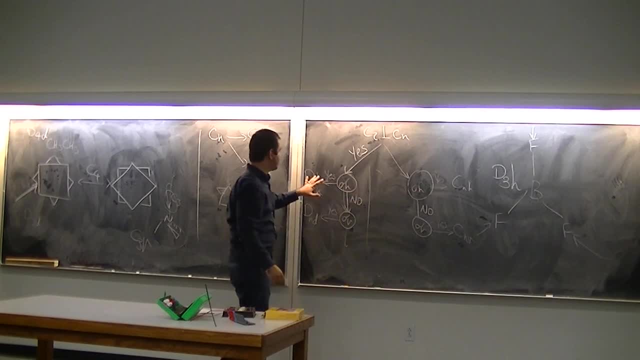 did cnh right. this was like the hitler thing, this was like the symmetrical structure, like that. and then we did dnd and cnb right. if the answer is no here, then this keeps up. okay, on the end all right, but the cn resists one more step. you have to check for one more thing, s2n. 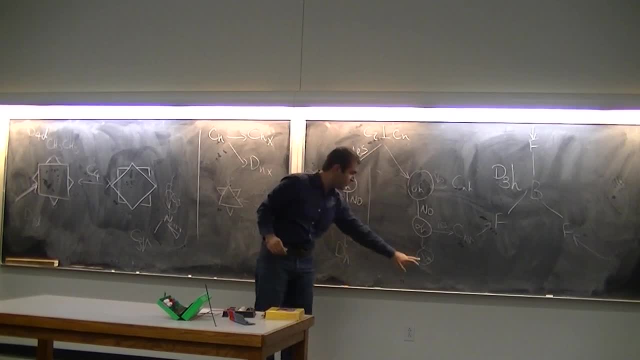 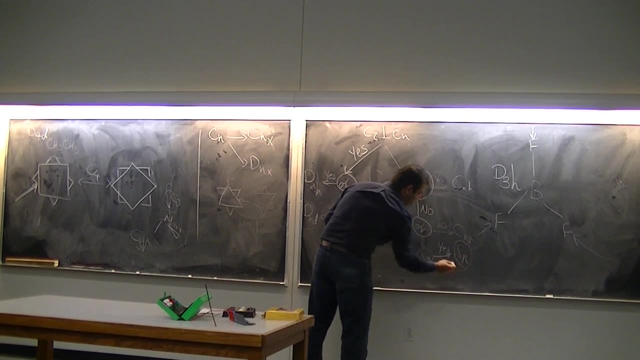 s2n like 2n means like if your main c is c5, it means to check for s10. if you have s2n, then your point group is sn, otherwise it is cn. so remember, if you're in a cn family you might have. 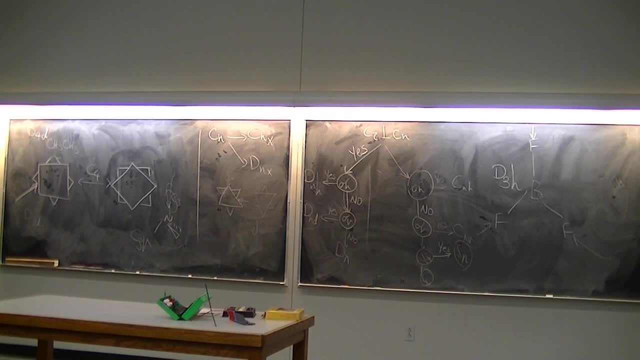 to take one more step. yeah, it says s2n. is that a mistake on the screen? no, no it. i wrote s2n too, so it should be s2n two times, whatever your n was. so if you're you have c5, you have to check for s. 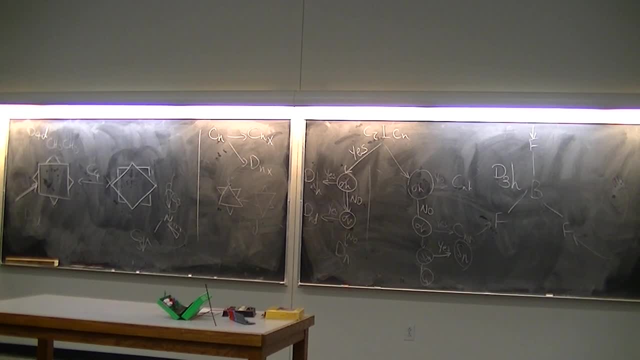 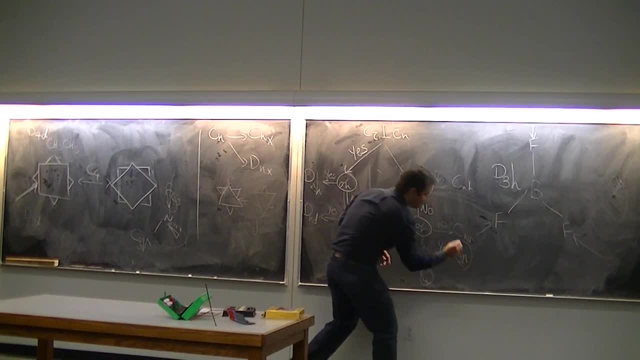 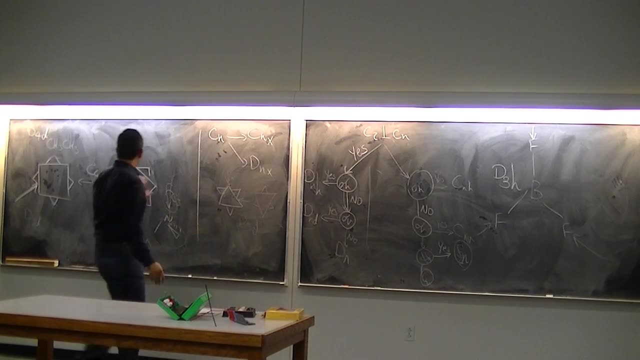 oh my bad. yeah, it should be s2n. yeah, thank you. okay, let's do this first. if you take that right and rotate the top square a little bit, not, not, not 45 degrees, not, i don't know. yeah, not 45 degrees, so it completely becomes a set here, but just a. 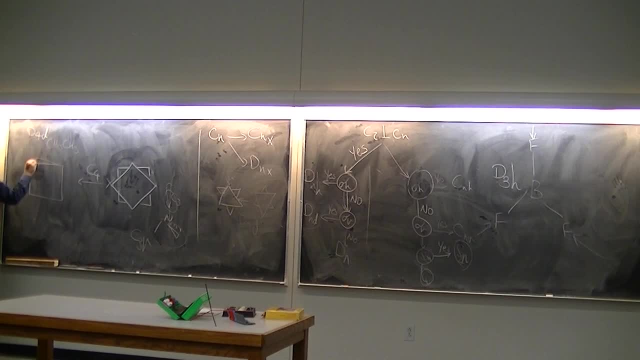 little bit. it will look like that: right, yea, right. so it is not eclipse, it's not a stack. what is the point group? what is the highest cn, c1, c4. right, there's a square on the top. remember, when you're rotating, when you're doing cn. 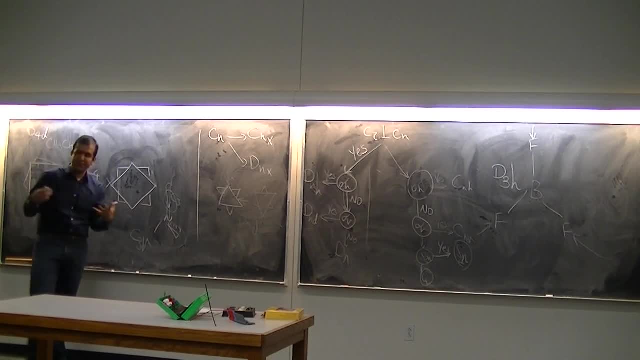 like this one. usually when you're doing cn, up and bottom are not related because you don't cut up. you know you relate anything in the bonn- bottom together and anything in the top together, okay, so what is the highest cm? so don't think like about those angles. this square has c4, the bottom one has c4, so both of them will have c4. 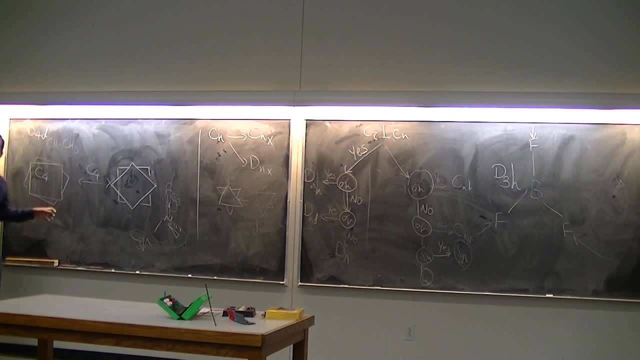 so we have c4 here, right, right. what is the next thing to check? perpendicular c2. do i have it? yes, don't try to see it. the answer is yes, why? because you have a square on the top and score in the bottom, so it has perpendicular c2. so we are in the dn family. does it have perpendicular? 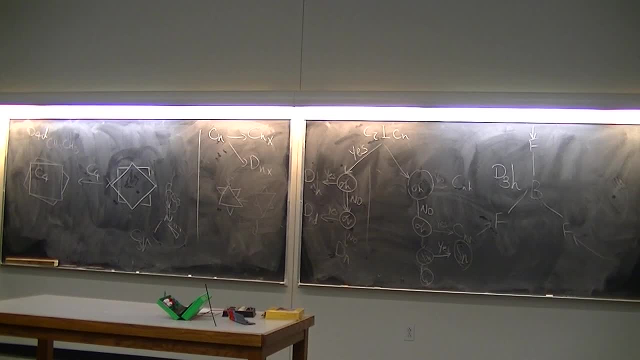 plane. does it have? no? no, if you apply that, the one in the back is going to come from the front and they are not exactly matched right. so we don't have sigma h. do we have sigma b? no, it doesn't have it, because if you want to apply for the top, if you want to apply for the 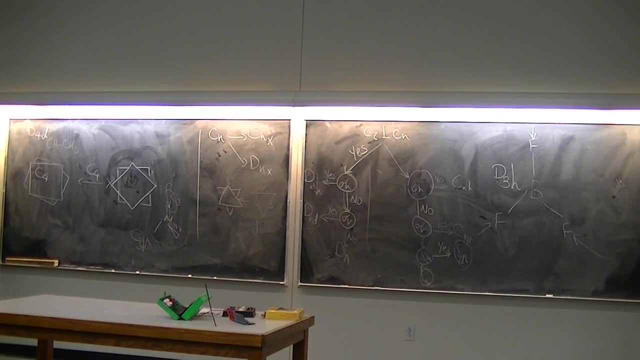 front square, it wouldn't work for the back one, right? if you want to apply this to reflect this on this east, then this one will go here where there is nothing. what about connecting the connection points of the tree? yeah, like that it is still. it still wouldn't work because this goes. 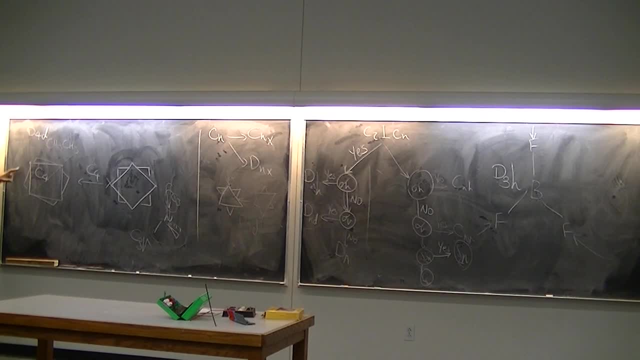 there. whatever you want to try to apply for the top one, it wouldn't work for the bottom one. yeah, actually, in the case where it worked here, the, the planes of the front and back would kind of lay on top of each other. that's why you had sigma be here. but if they are not, 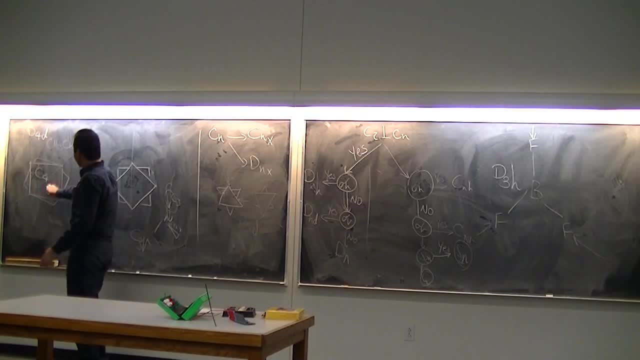 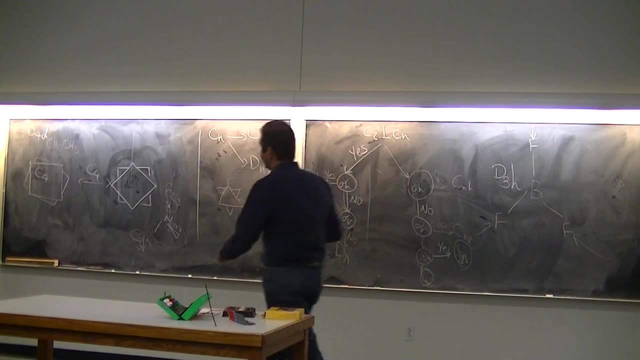 uh, if it's not completely staggered or completely eclipse. you don't have sigma b. what's your question? yeah, how about like this, like right, uh into through this, like, uh, the edges there, you mean like there, like here, i mean like, remember, this angle is not 45 do? 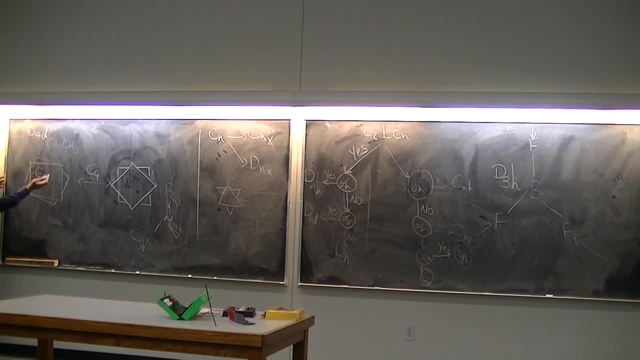 you mean something like i. okay, let's break it down into square by square. if it was just one square, right, this is square per square, right, right, this is going to be a square and it's a square in, i'm right. okay, so between x and 2 is x about 0.7 kilometers. 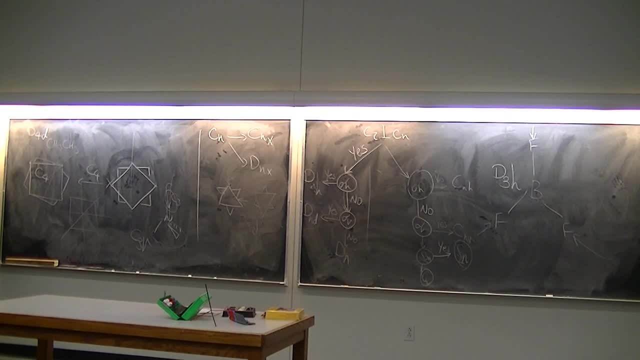 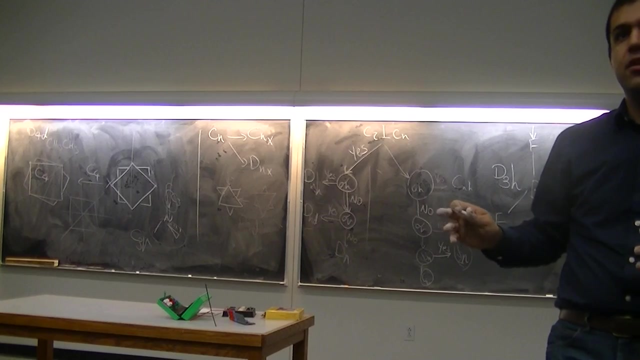 and the total difference in one square is just again, better to me than because this y happened to be a point p by h, right? so exactly what is coming? this wholenothing, because so now i'll teach you what's where the plan is going. i'll teach you everything. 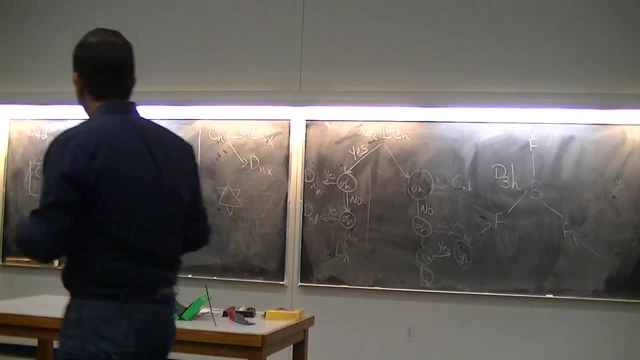 you know i mean where this goes. so i have max square notes for the front of a square which a chena. anything else here. come on, man. do you know where that would be? the top of the like the square on the top. reflect to the back of the like. the square on the back. 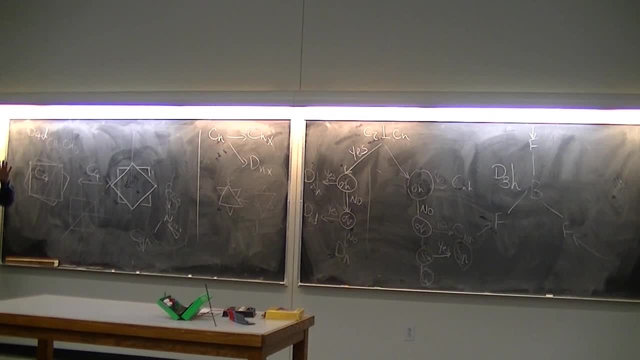 So I mean like Well, sigma B's cannot relate anything from top to back, They just anything that is in the top will be in the top. it just goes from left to right. So these sigmas just don't stand anything. from top to bottom, it just 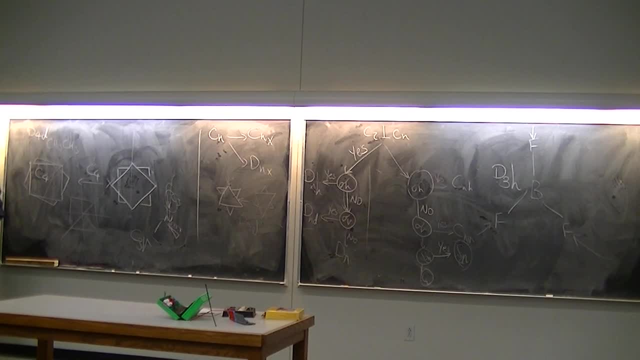 Are you talking about something like this? Oh yeah, that's C, That's C2, good, but that's C2.. Sigma: it does not have the sigma, So we don't have any sigma here, okay, So what is your molecule? 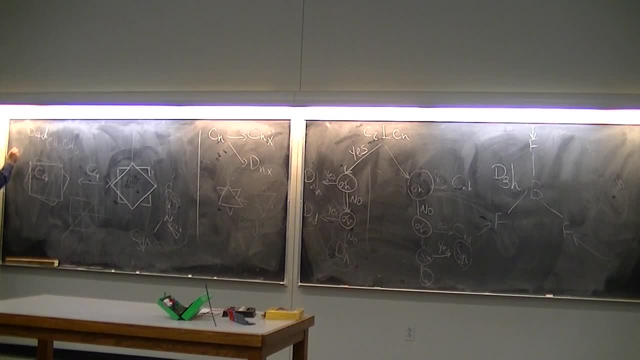 It's Bn, it's B4.. Okay, so it's quite interesting If you start. what is this? What is the staggered structure? Sorry, eclipses structure, If the two squares are exactly eclipsed, what is the highest Cn. 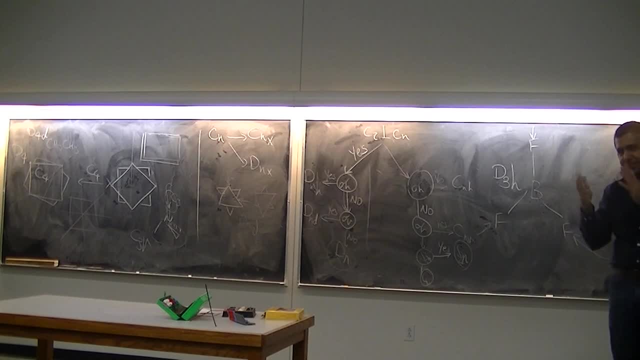 C4.. C4 again. does it have perpendicular C2?? Yes, Yes. does it have sigma H? Yes, Yes. so if they are completely eclipsed, it's D4H. okay, If you rotate it a little bit. 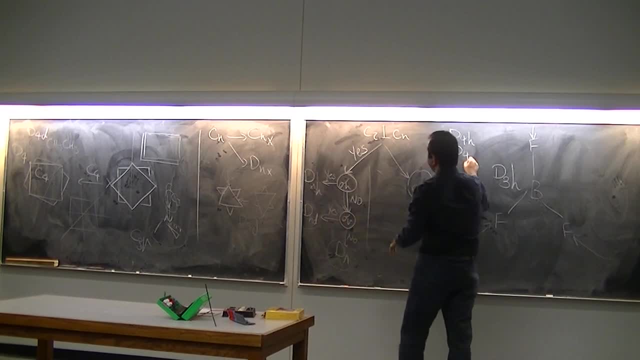 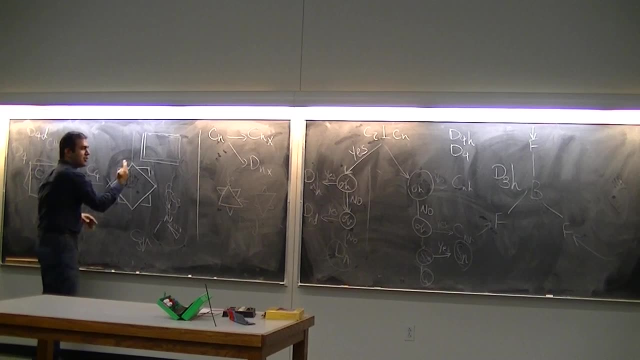 the sigma will disappear. it becomes D4.. If you keep rotating it again, become a perfect, staggered structure. it will regain some sigma. it becomes Dn. You got it, guys. You could say the same thing for Fn. Do you remember about the rotation around the single bond? 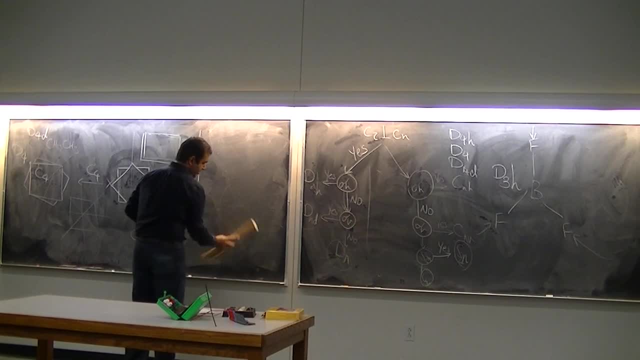 in organic chemistry, in the organic chemistry, When they said that there's, I don't know, three or four kilojoules per mole energy required for this rotation. Do you remember from Orgo? Okay, This is what This is: D3.. 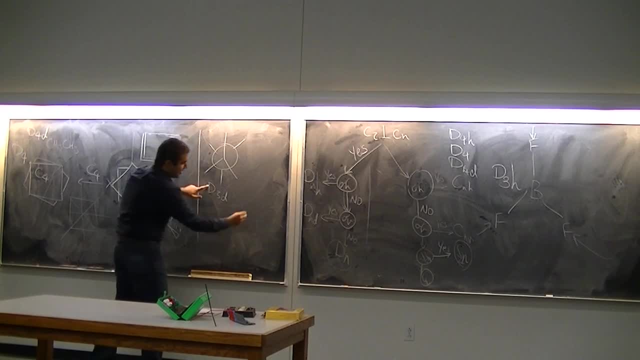 This is D3.. What is this? Come on guys. what is this? D3H, D3H, What is anything in between? Because the sigma V and the sigma H, both of them, so anything in between will be D3.. 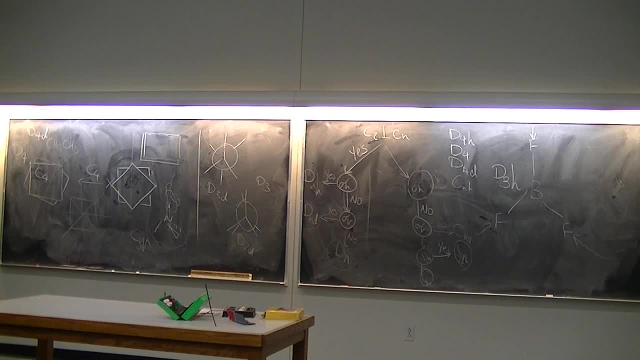 You got it. What is D3?? What is D3H? What is D3D? You got it Okay. Okay, Let's do one here, Okay, So if I make a funny structure, just like the Hitler structure, 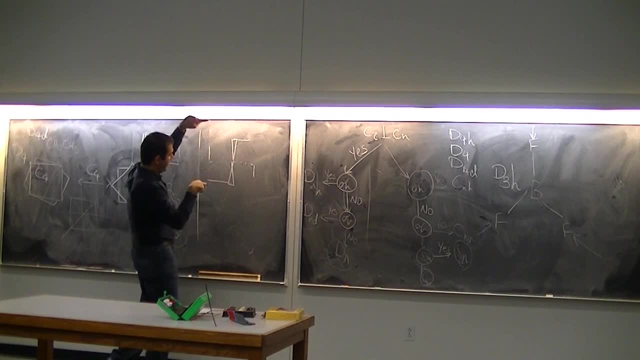 but up and down. So remember, those two are just like there and those two are in the back. What is the highest Cn? It's a weird molecule. it's just a shape. I don't know. I don't think there's a molecule. 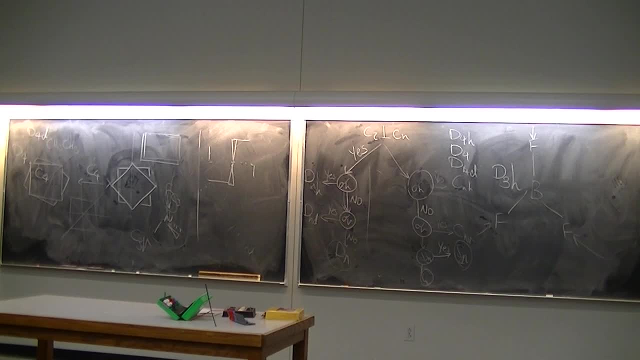 we have such a molecule, No each, no no, there are four arms, but they are. it's like ethane, It's like, yeah, it's like methane. So you have, you have okay. So think of this okay. 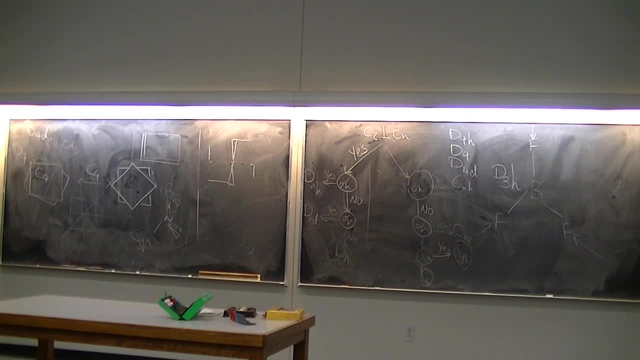 where two of them are pointing toward you and two of them are going, or maybe like that. Okay, So those two are, you know, are pointing toward you and two of them are going in the back, but each one has a tail. 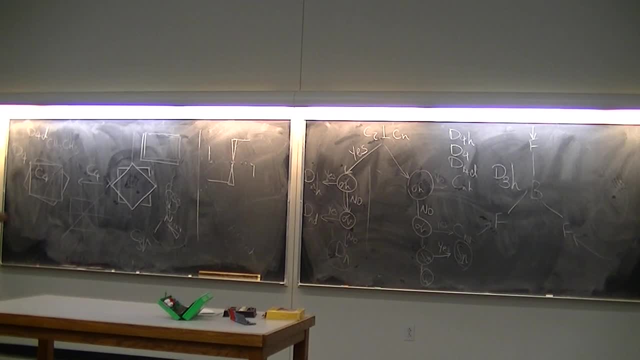 Okay, All right, Let's just figure this out. Let's say someone someday makes a molecule like that. What is the highest? Cn, C2. C4. C? no, it does not have C4, because if you rotate it 90 degrees, yeah. 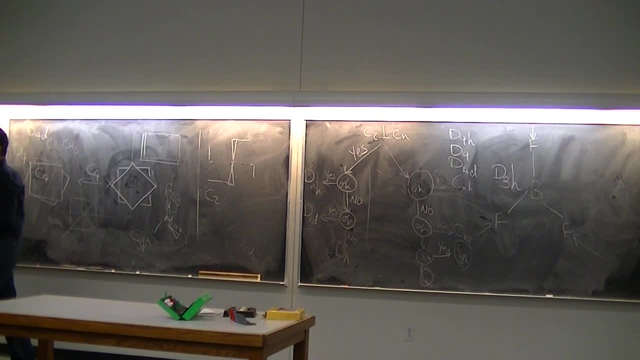 It has C2.. Does it have perpendicular C2?? What did I tell you about Hitler? Hitler hates perpendicular C2, okay. So no perpendicular C2 because of this. Okay, so remember: tails, kill perpendicular C2.. Now right. 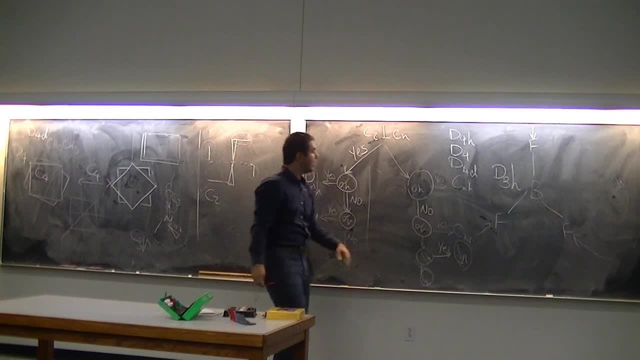 So we are in the Cn family. all right, We are here. Is there any sigma H? There's no sigma H, because if you apply that, those from the front will go in the back, those in the back will come in front, right. 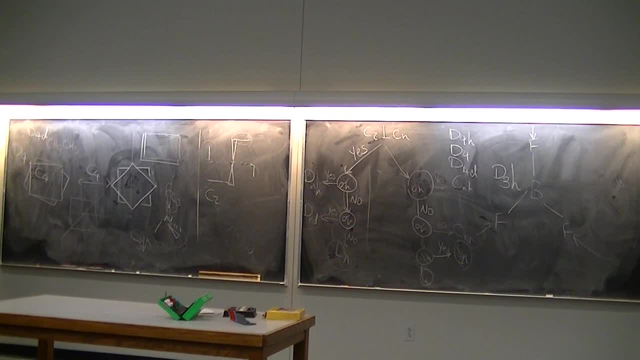 So there's no sigma H. Is there any sigma V? Actually, Hitler hates sigma V, Sigma Vs will, I forgot to tell you. So sigma Vs will be also gone, because if you apply that, this tail will go. there will go here, right. 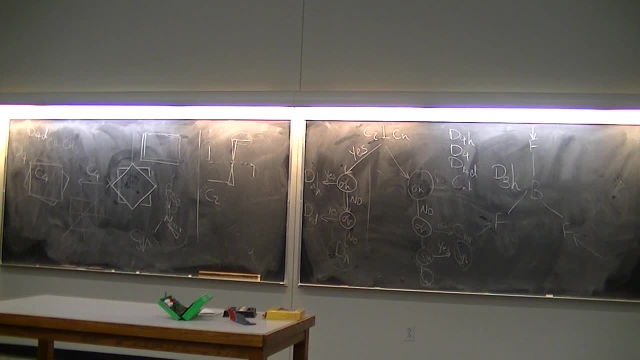 What is the next thing to check? Look at the table. S2.. S4, yeah, Because your C is C2, you have to check for S4.. Does this molecule have S4?? Yeah, even if you didn't know it. 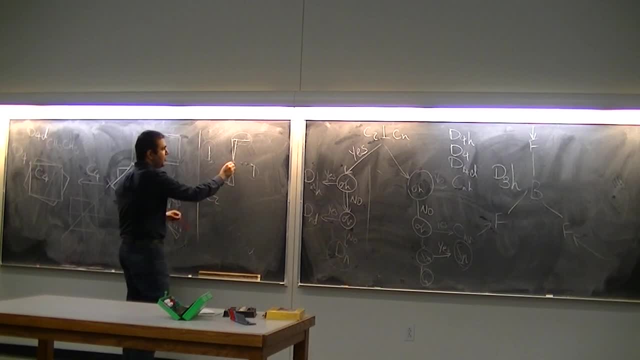 the way I said it, it was quite obvious. It does have S4. If you rotate it by 90 degrees it becomes something like this: And if you apply sigma H now, these from the front will go in the back and these from the back will go in the front right. 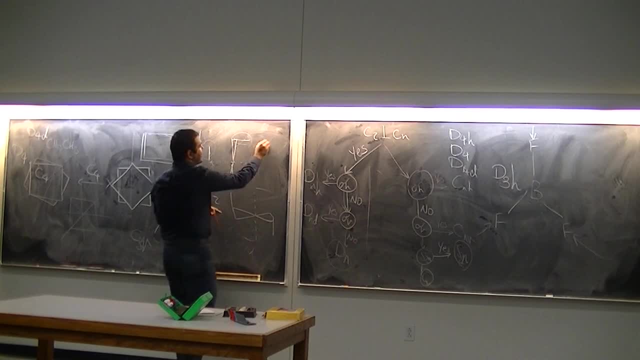 So this molecule has S4. The point group for this molecule is S4.. Okay, you got it. You hardly can find a molecule that is S2, but it's there. Okay, let me give you one example up here and then we'll go to character data. 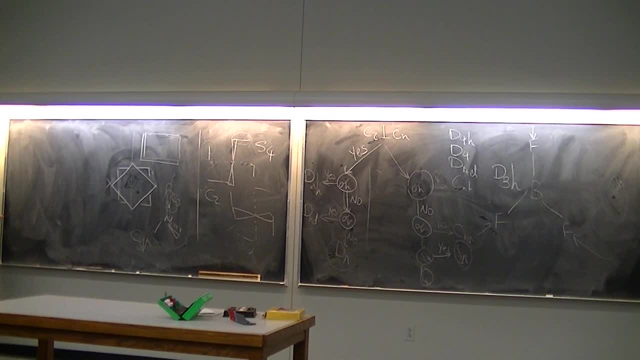 Any questions? All right, any questions? Okay, Yeah, if you have a Hitler structure, let's say, with all of them pointing toward you, something like ammonia. but remember those hydrogens are like Hitler. They have theta. What is the highest Tn? 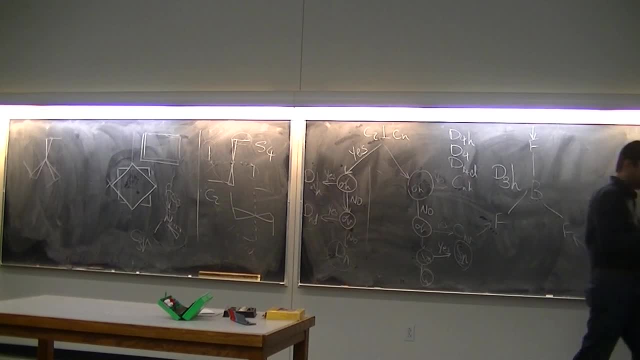 C2.. C2, very good. Does it have perpendicular C2? No, Hitler hates perpendicular C2, and besides, up and down of this molecule is different, right? Remember, it's like a pyramid, Up and down different. no perpendicular C2, no sigma H, right? 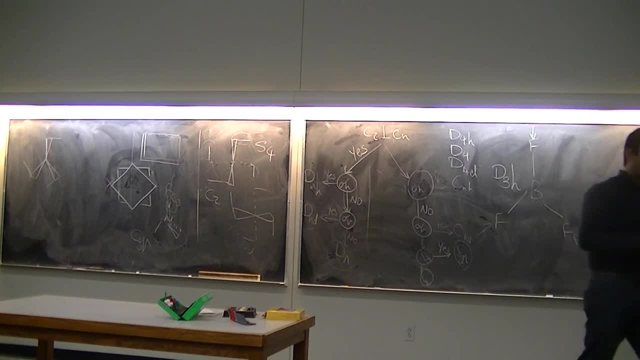 Does it, So we are in C and does it have sigma H? No, I just said you don't have it because up and down are different, So it does not have sigma H, right? If you apply sigma H on this, remember this is your C2.. 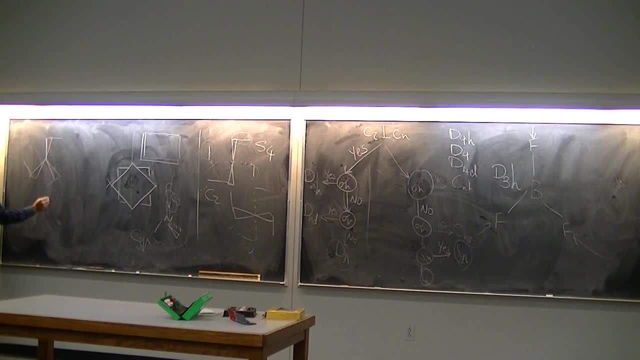 If you apply sigma H, it's gonna look like that: The pyramid actually kind of inverts. Okay, so there's no sigma. Does it have sigma B? No, because if you apply it, the tails will flip and we don't have it. 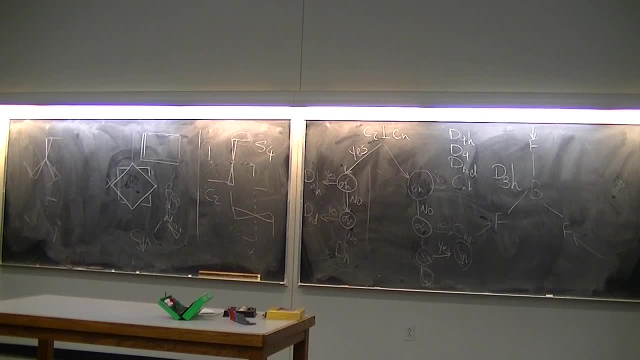 Does it have S6?? No, it doesn't. Those Ss are for are for structure like this: when you have up and down and they are like offset, There's some sort of offset. So this is what C3.. 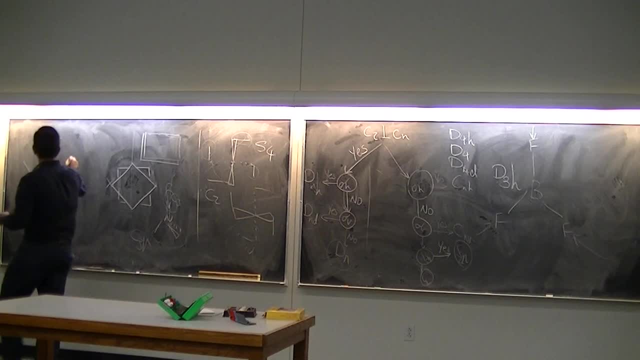 C3,. the point group for that molecule is C3.. Any questions about the character data? What is it? the point group is that it? Yeah, Can we go back to the previous Hitler molecule? So for the S4, so you rotated C4,. 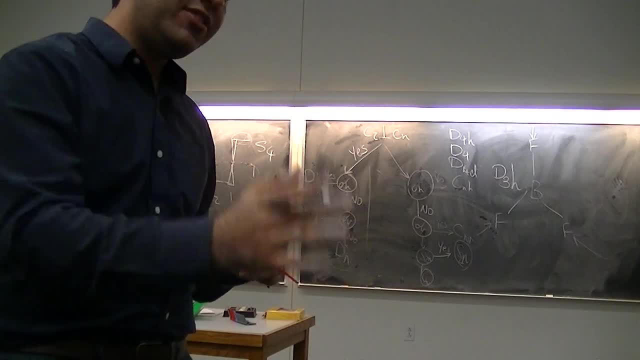 then where's the sigma H after Perpendicular to the C4 that you just to the C4 that you just applied? Yeah, where is it? could you show me? Yeah, yeah, so how did you do the C4?? 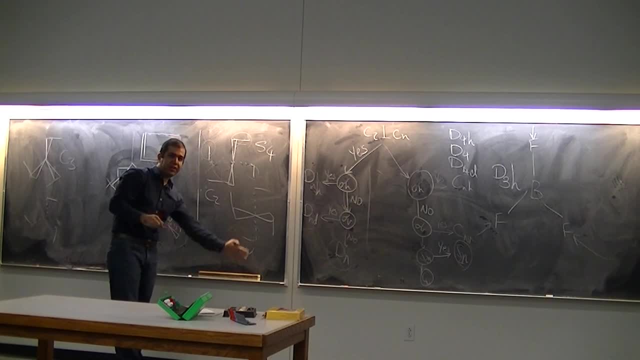 Did you not rotate it like this: Yeah, So we are looking for a sigma that should be like that. Yeah So, where are we? Is it not like that? Yeah, So if you apply sigma, this will go there, Because it becomes. I mean, this is Cn. 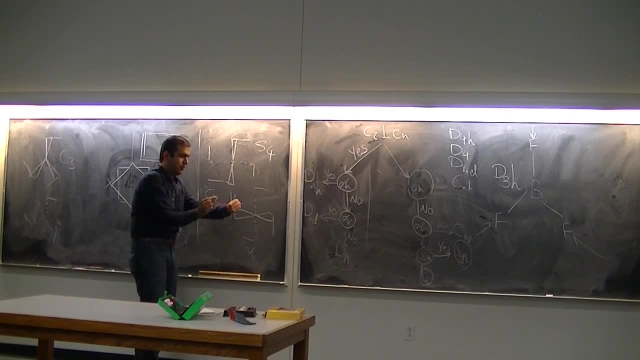 but think that this kind of these two go in the back. I'm not sure Dr Martin will be happy if he sees it. It becomes something like this: right, Okay, The ones in the front will go in the back, the ones in the back will go in the front. right? 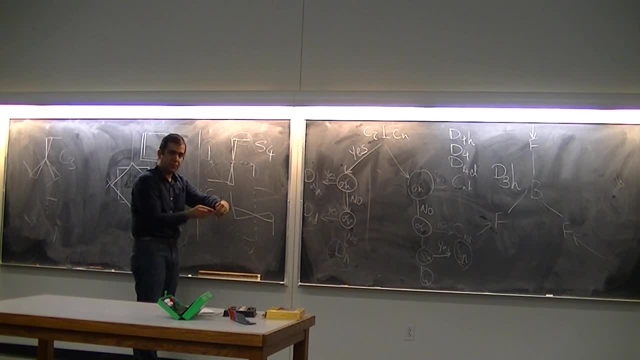 So I have to draw these like solid and draw these like points, because they're already and it's going to look like that. Okay, Is it not? this? These two warning pointing toward you, and this one. 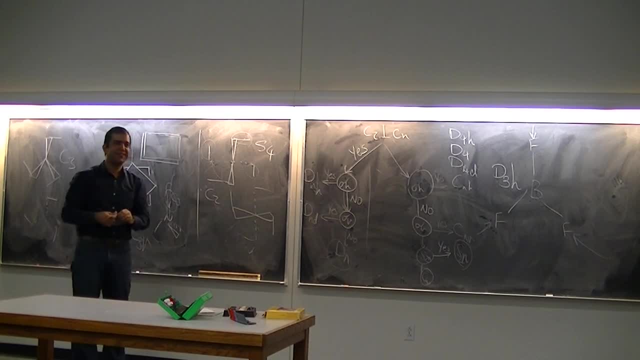 Oh, yeah, yeah, yeah, Oh, okay, I see, Okay, yeah, So for when you do like tests, do you have to take the rotation by the plane or, if you can, by the plane, plane to the rotation axis. 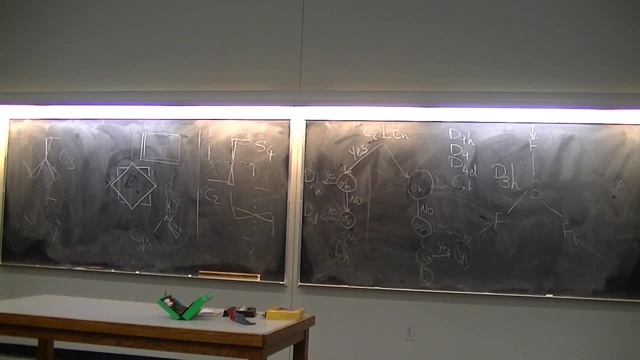 Is it the original axis? Is it the original? Oh, okay, no, no, In 99,. in all cases that I know of, they are the same. Okay, The CN that you are doing is the same as the CN axis of the SN. 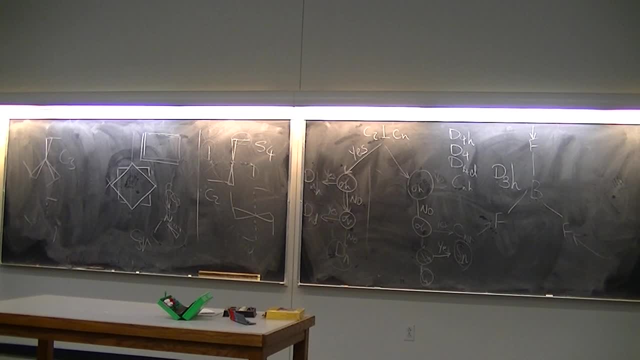 Okay, so they are the same. But even if they were not, the sigma that you apply should be perpendicular to the CN that you just applied to that SN. Okay, So you apply C4.. If your C4 is perpendicular to the plane of the board. 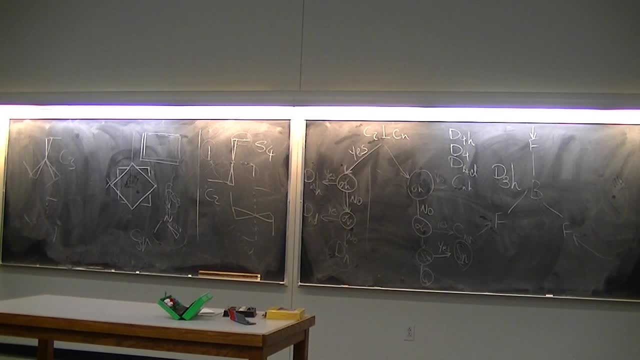 then your sigma will be the plane of the board, which is perpendicular to that Clear. So, guys, I have a couple of things to remember. If you just attended the session, these are the important things that I think I talked about. 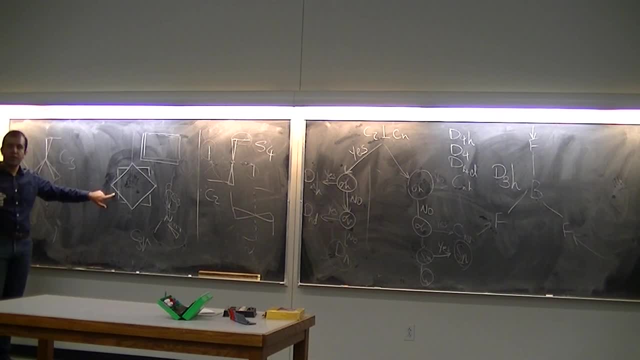 If you have structures that are similar to this, where you have a square in the top and a square in the back, okay, a square in the top with similar elements. not in the case where you have flooring here and flooring in the back. 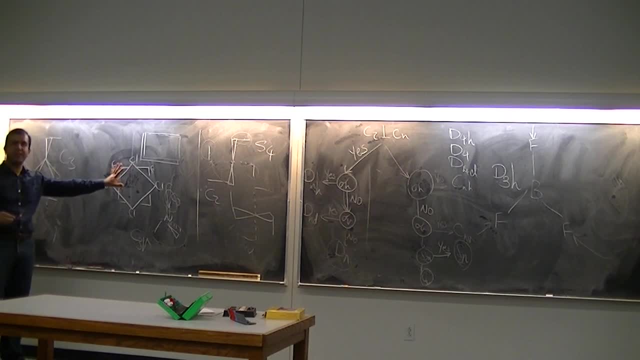 If you have super similar structures in front and in the back, Okay, A triangle in front, a triangle in back, A square in front and a square in the back, Okay, You definitely have perpendicular C2.. Okay, One thing to memorize. 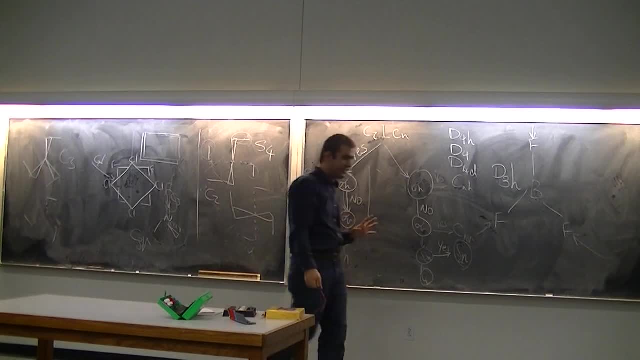 And the second is that if up and down of your molecule with respect to your CN is different, just like ammonia, You have a C3, up of ammonia is nothing and bottom of ammonia is R3 hydrogen. If they are different, there is no perpendicular C2,. 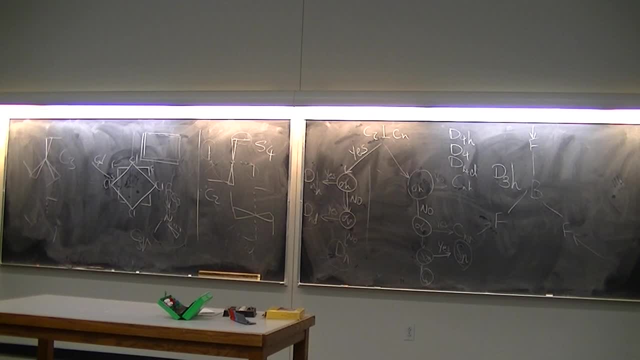 there is no sigma H. Okay, These two are important And you can always All right, guys, Any questions here? Do I move to character table Or do you need more examples on point groups? Let's do a couple of examples on that. 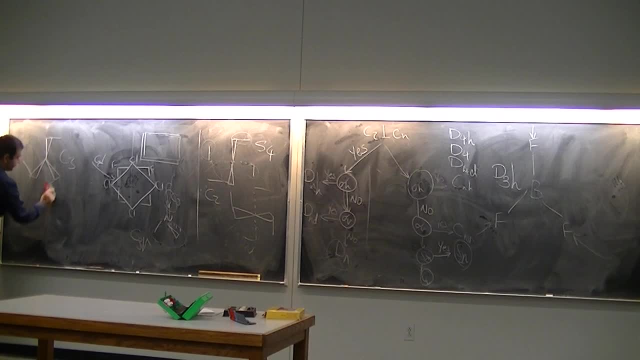 Okay, Let me give you a tricky one. What is this? What is the point group for this? FFH? Okay, FFH. FFH C2H: No, O, O, O, O O O. 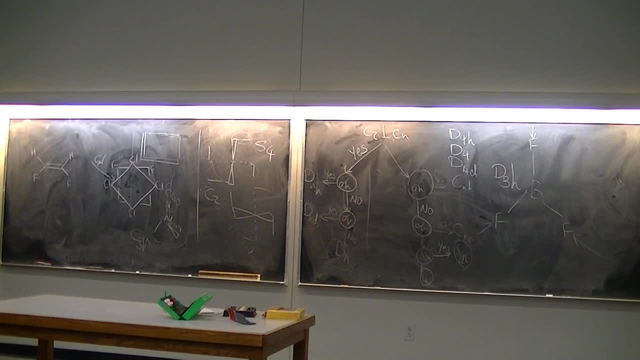 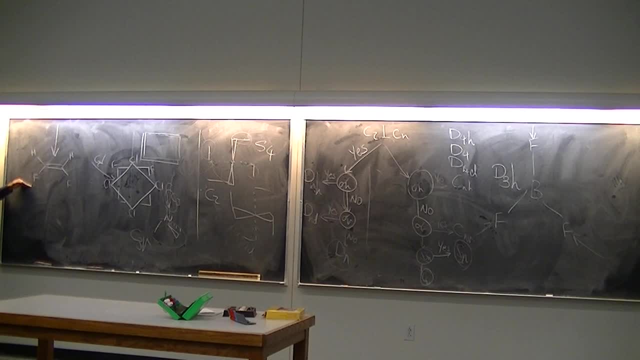 Up and down are what? Different hydrogen fluorine. Okay, up and down. with respect to your CN, it's different, right? So there's no perpendicular C2, there's no sigma. So you quickly jump where Here. So we are here. 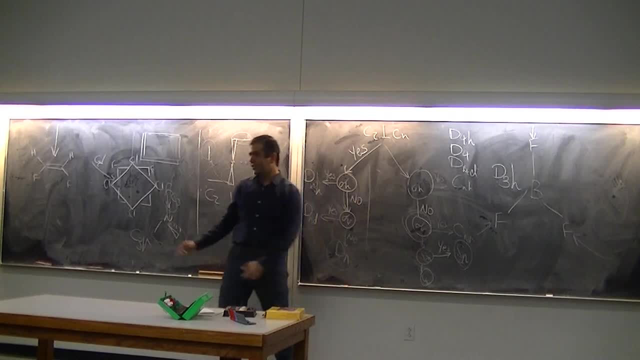 We have to check for what Sigma B Does it have? sigma B, Yes, Yes, so it's C2. B. What about this? Fluorine, fluorine hydrogen hydrogen. What is the highest? CN, CN. 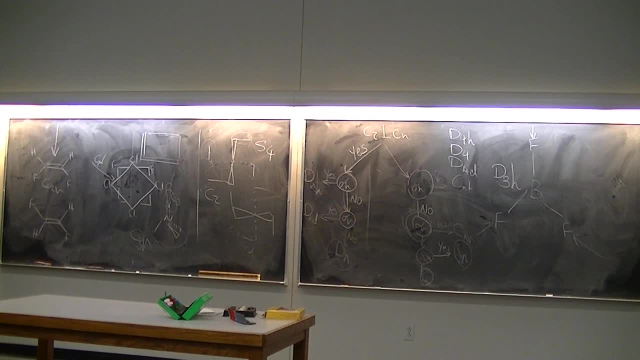 It has a CN, if you want. Yeah, Does it not have a C2 like that? Okay, 180.. 180, right. So what is the next thing to check? Perpendicular C2, right, It has a C2.. 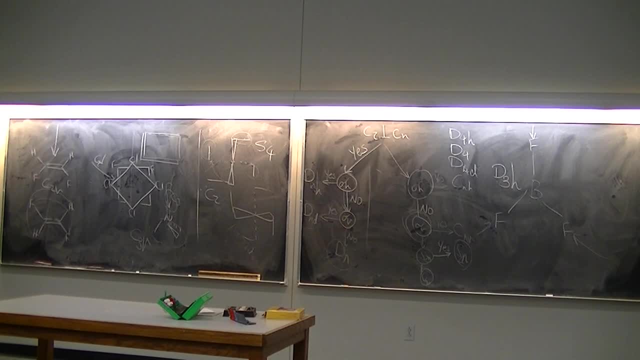 That's, it happens to be your main principal active. Is there any perpendicular C2?? No, Does it not like? look like a Hitler? If you want to simplify this molecule, it looks like this right Similar to Hitler, right. 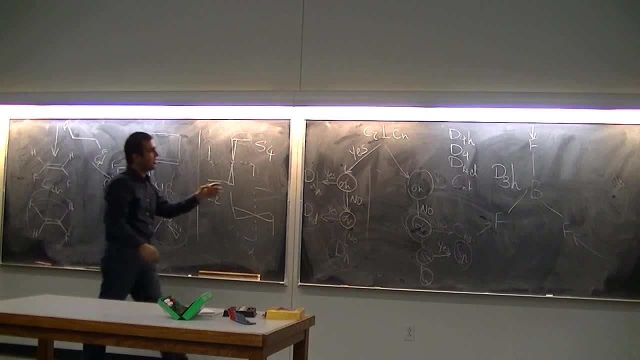 So it does not have perpendicular C2.. Does it not? No, Does it? what is the next thing to check? X, So it does not have perpendicular C2, so we are in the CN family. We have to check for what? 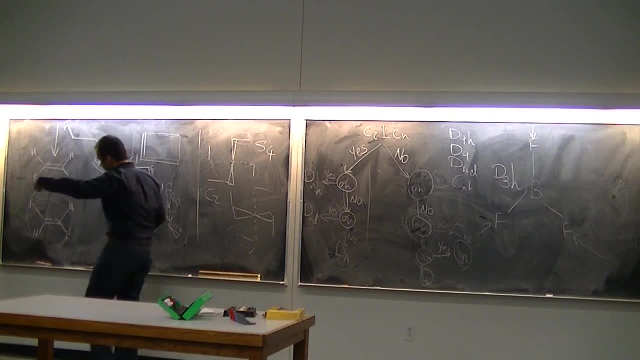 Sigma H, Sigma H. Does it have sigma H? And since my C2 is there, my sigma H is like that. Is it a plane for this molecule? Yes, Yes, So this molecule is what? C2H, C2H? What about FH, if all of them are hydrogen? 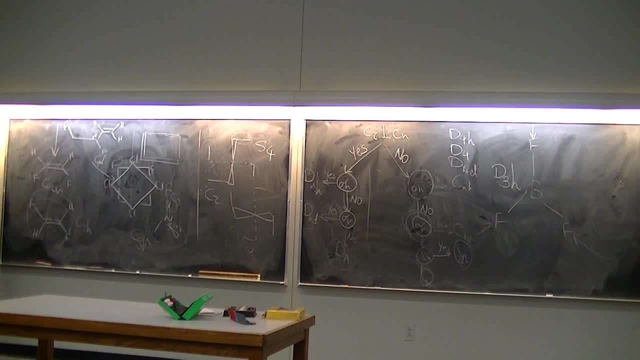 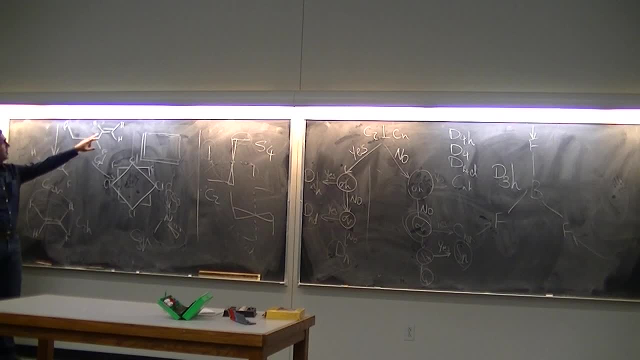 Yes, Very good. What is the highest C2?? Well, it has three C2s right One is in there. If you rotate this molecule, 180, like, let me just drop that. Okay, If I apply a C2 like that, it becomes a cell right. 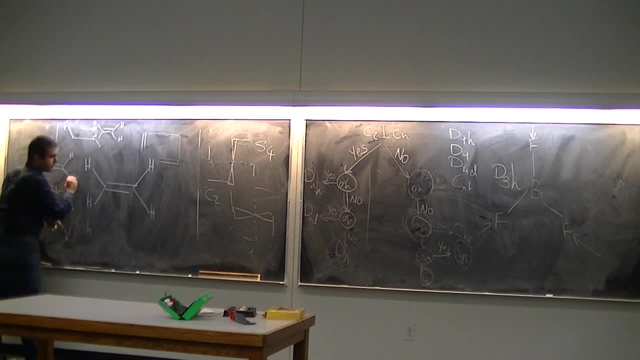 right, This will rotate 180.. This goes there. It goes through the two carbons, so you don't have to worry about it. And this goes there. that goes there, right. Right, This is the C2.. It also has a C2 like that, right Where. this goes there. this goes there 180. Just. 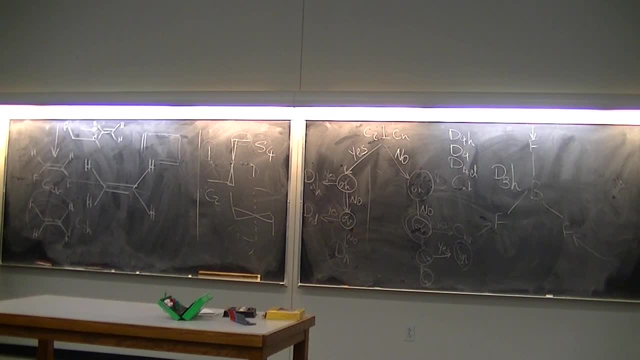 get the molecule and rotate it 180, it becomes itself And it has another C2 like this: If you rotate it like this, those two will just rotate and go back. Right, So it has the C2. and it does have two perpendicular C2s perpendicular to the matrix plexus, right? So we are in. 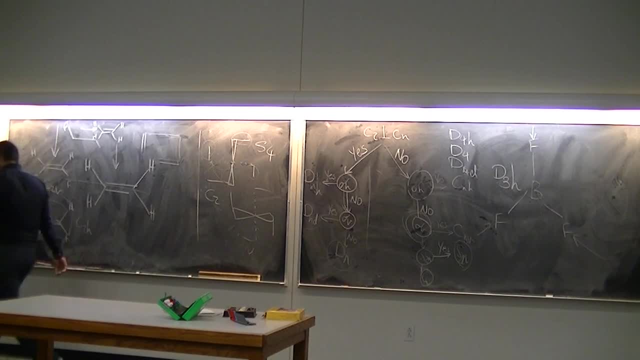 the Dn family. If you think, okay, if you have. I mean, in most cases it doesn't matter. but if you have multiple Cn's, the Cn that goes through the maximum number of elements is your high Cn Right. So if you have multiple Cn's, the Cn that goes through the maximum. 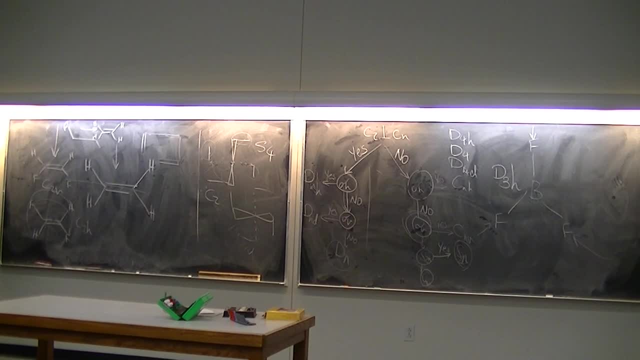 number of elements is your main principal axis? Okay, In this case, I have a C2 like that, I have a C2 like this and I have a C2 like that. That Cn goes through two carbons, right. So that's your Cn. Does it have a perpendicular plane? It does, So this is P2H. 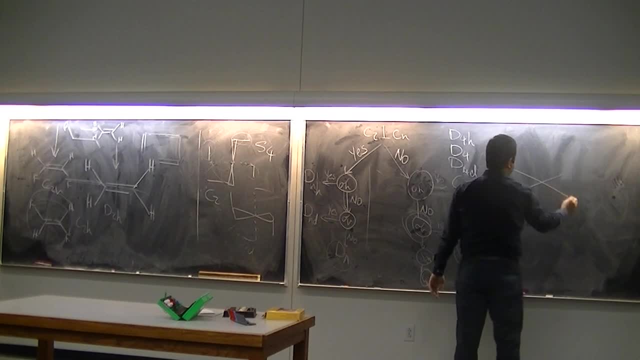 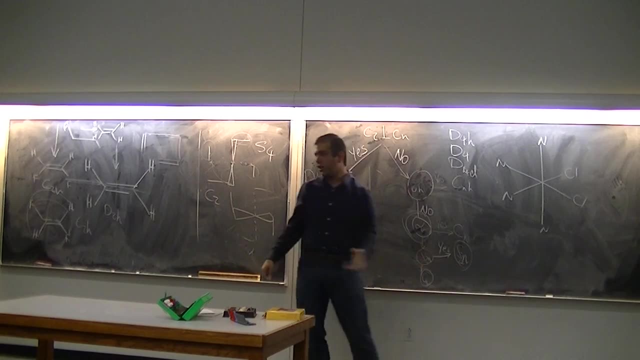 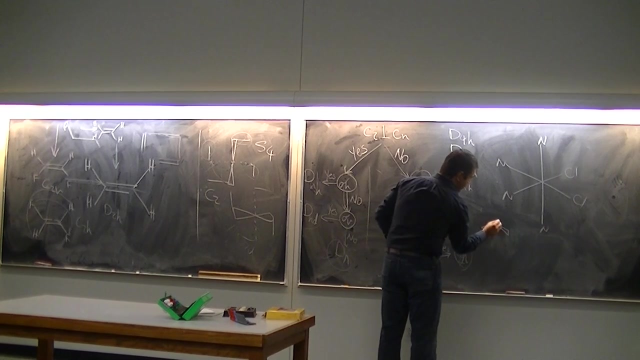 Okay, let me- and this is the last one, then I will character it Chloride, chloride, ammonia. these are ammonia, NH3, but think of them as N And remember this is octahedral, right? So this is structured. those two are. I'll just draw it here then. These two are in the 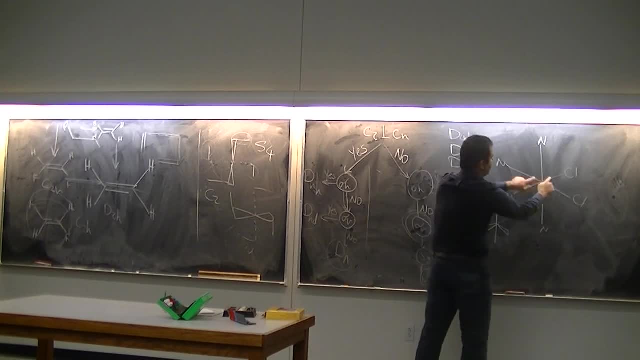 plane of the board. those two are toward you and those two are in the back, So think of it as octahedral. What is the point? What is the highest Cn? C2.. C2, very good, Yeah, there's a C2 through. 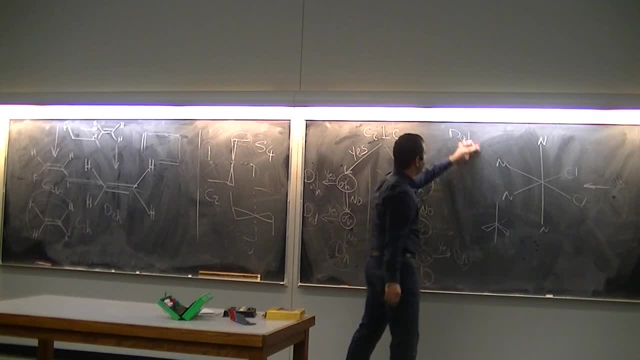 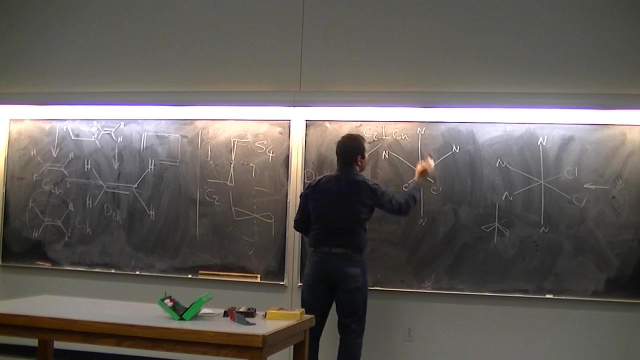 there. Let me help you. if you have a hard time to, if you have a hard time to see those, try to rotate it so that you can see it easier. Is it fair if I draw it this way: Chloride, chloride, chloride, And remember those two are toward you. So if I take those two chlorines, 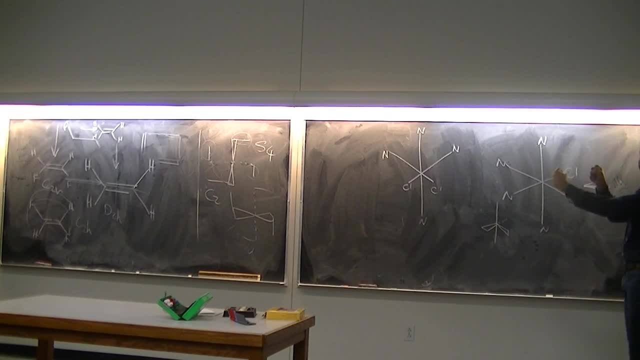 and rotate it 90 degrees so that the two chlorines are in front of the board and those two nitrogen just go in the back Right. It will be easier to see the C2.. C2 is where. Remember, these are not pointing down, these are just there. but since it's a 2D picture, 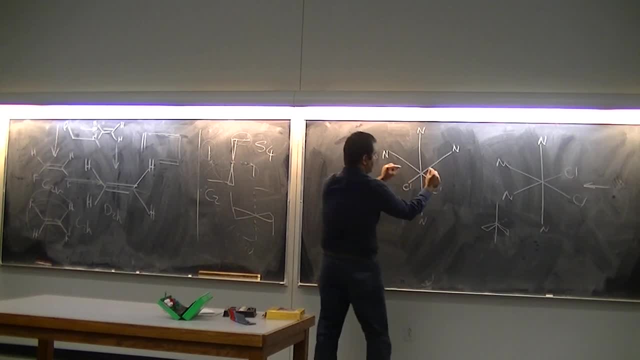 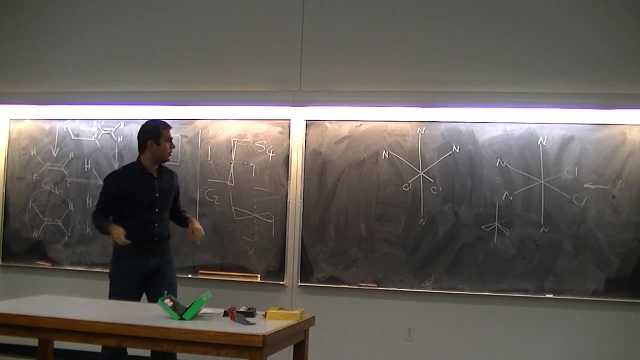 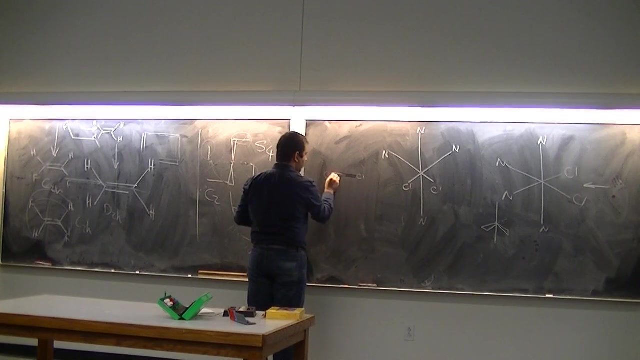 I cannot draw it. I draw them that way, but actually those two chlorines are here and those two nitrogen in the same plane are in the back Right, So maybe I should have drawn it like that. Is it clear, guys, What I meant? 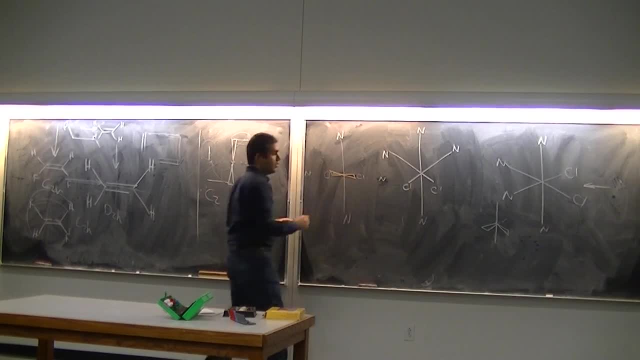 Two chlorines here, two chlorines toward you, two nitrogens in the back, two nitrogens up and down. Does it have a C2?? Yes, it does have. So there's a C2 through there, It's. 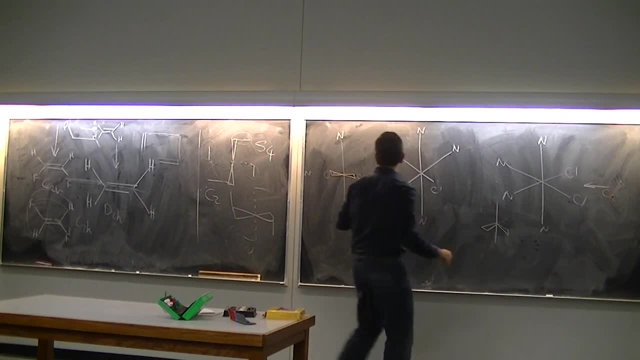 actually this C2.. If you have a hard time seeing it here, try to rotate the molecules, make it look like that and you can see the C2.. Right, Does it have a perpendicular C2? No, Why? Yeah, but you may say more simply, Up and down, What is up of your molecule? with respect, 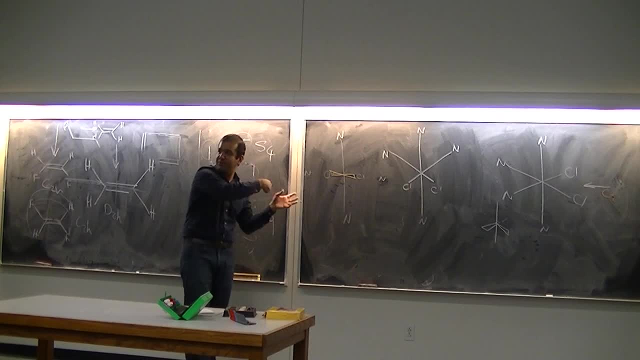 to your Cn: Clorine, Clorine. What is bottom of your molecule? Nitrogen, Up and down, different, No perpendicular C2, no sigma. Okay, So we are in the Cn family and there's no sigma. Is there any sigma V? 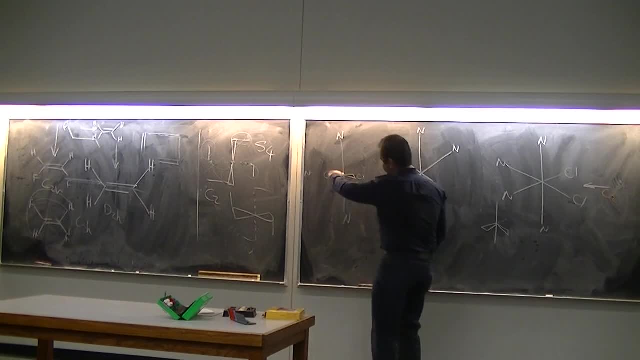 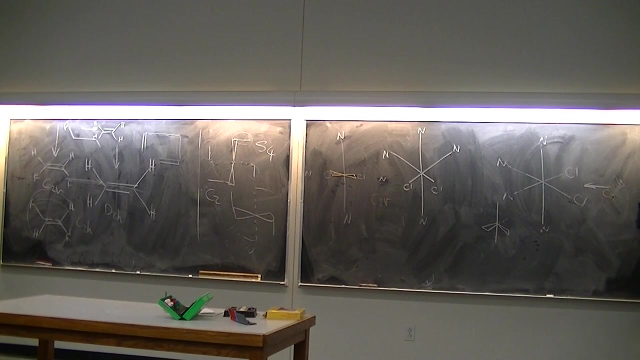 No, Oh yes. Yes, If this is your C2, there's a point like that. So this is C2V. It's actually similar to water, although it's so large, but it's the same as water. If you just ignore all of them, it's like water hiding in nitrogen, Right? 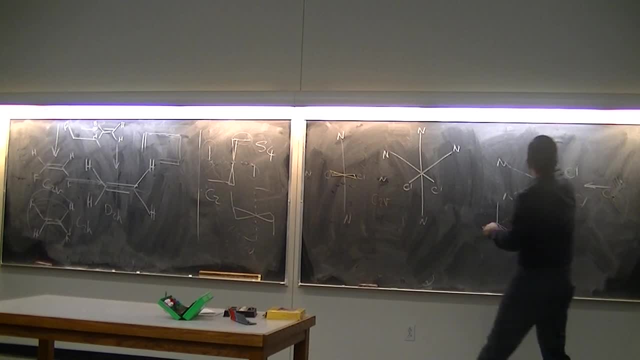 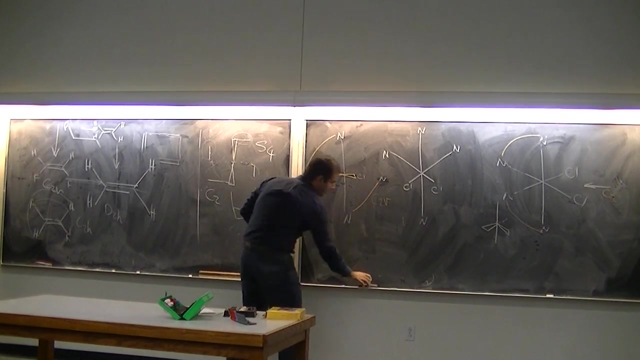 It's C2V. Now if I connect those two nitrogens together with some carbon, what will the point group change into? So remember that nitrogen is connected to that and that is connected to this. Does it keep the C2?? 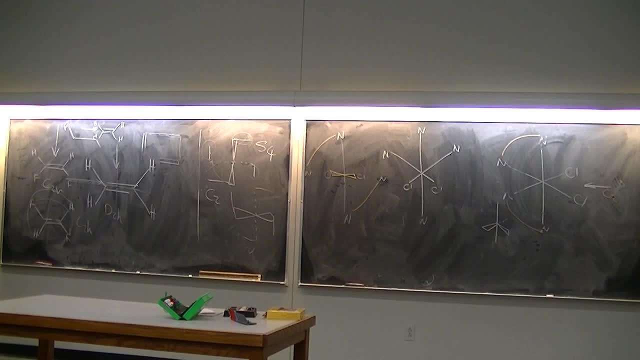 Yeah, why not? If you think of it, if I apply the C2, this will go from there to there. This nitrogen will go here. Let me just number them for you so that you can see: Guys, are you comfortable with this structure? 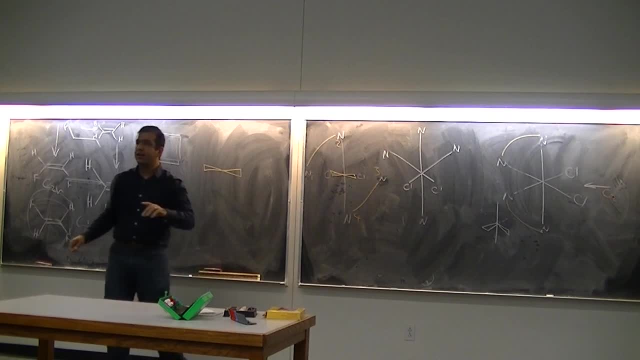 Yeah, Right, Do you understand what it looks like? Yeah, Can you show me the like? what is V, Like what is C2V? Okay, Do you see? Okay, So you were talking about these were not here, right. 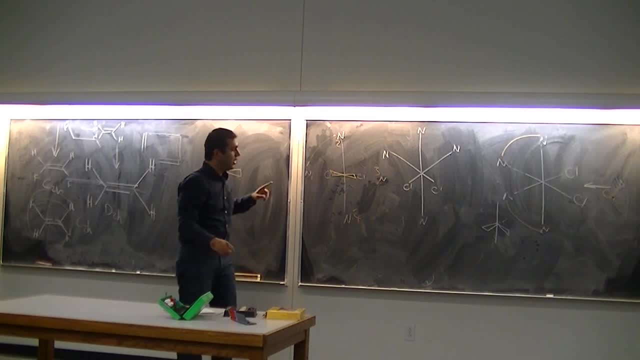 Yeah, Yeah. So do you see the C2? Mm-hmm. Okay, If so, your C2 is here, right? Do you understand that? those two chlorines are toward you? Yeah, Yeah, And those two nitrogens are in the back, One of the things that I just said in the. 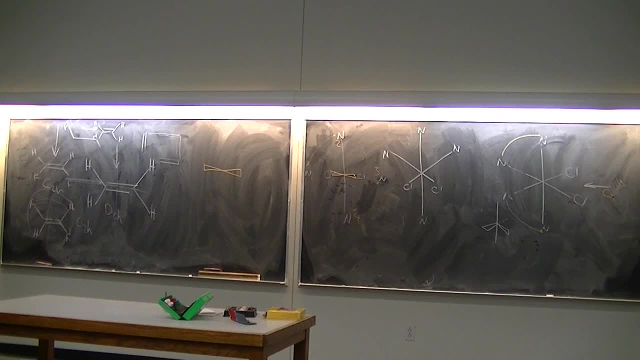 last session is that if top and bottom of your molecule with respect to your CN. so when I say up and bottom I don't mean those two. Yeah, Look at your CN up and down with respect to that. If they are different, are they different? 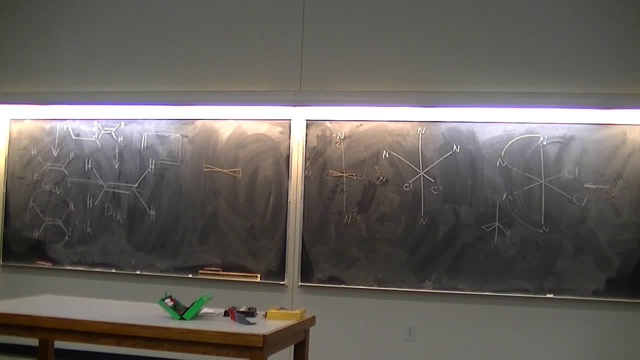 here. Yeah, You have chlorine and nitrogen. They are different. If they are different, you don't have perpendicular C2 and you don't have signal nitrogen. Okay, You can just memorize it, Okay. Okay, So you have a C2 and you don't have a perpendicular C2, so you're in the CN family. 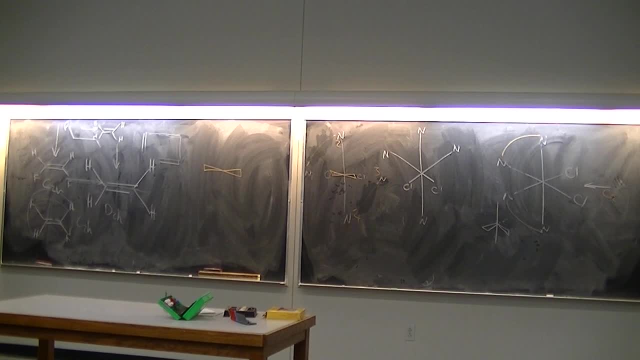 in that chart and you don't have sigmoid. So you have to check for sigmoid, which is a and sigmoid. it does have a sigmoid. If you apply, this is your C2, and if you apply a plane like that, you see it goes through carbon. the chlorines are reflected under 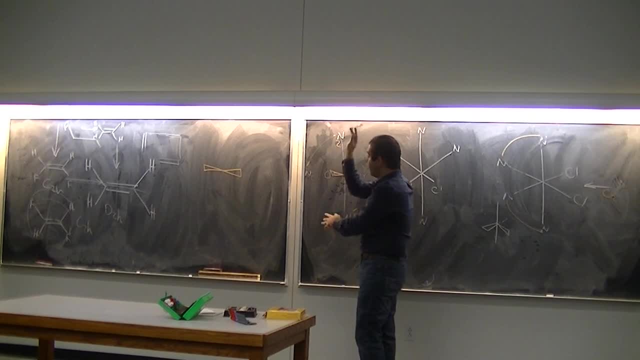 each other. those are nitrogen and it goes through those two. And what is the sigmoid? It's parallel to your C2.. So it is a sigmoid. So if you look at your chart, if the answer to the sigmoid is yes, then your point is correct. 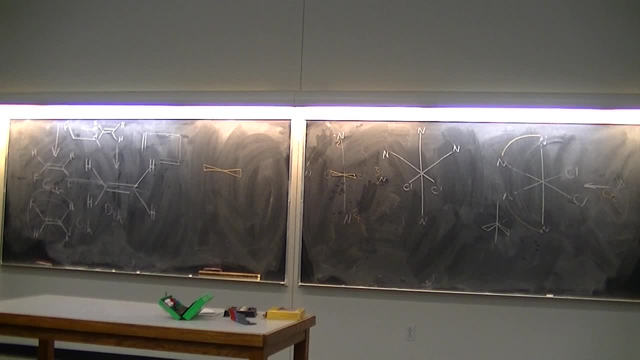 If the answer is yes, then your point group is CN. Okay, And since N was 2, it will be C2.. Okay, Now assume that those nitrogens are connected to each other. So if I apply the C2, where does Cl1 go? 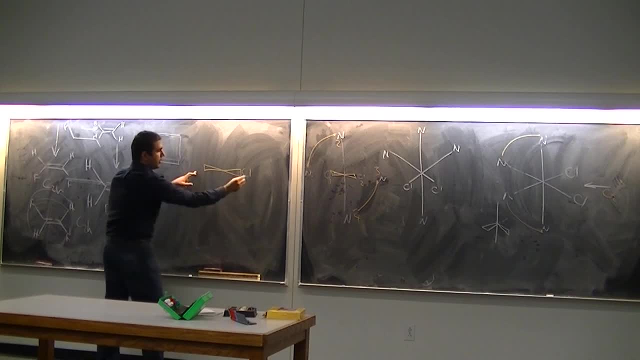 Cl2.. Yeah, So Cl1 will go here and Cl2 will go here. Agree. What about N4?? N2.. N2.. Yeah, N4 will go there and N2 will go here. Right, And remember, these are connected to. 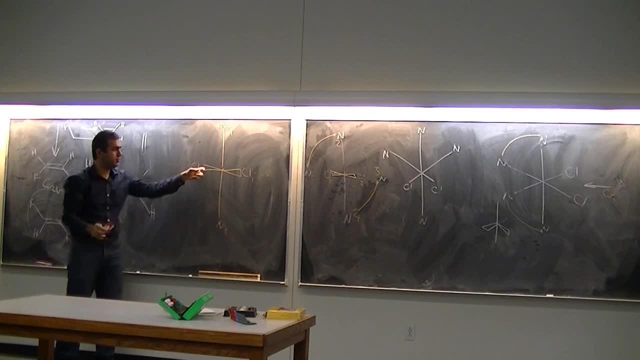 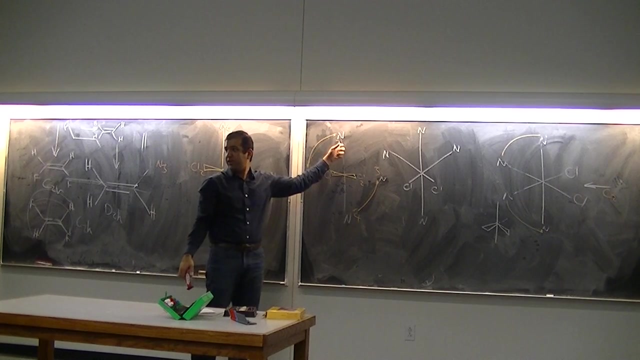 the center ion. here They are just hiding behind those chlorines. Okay, These two. So what about N3?? N1.. N1 and N2.. So what? two nitrogens were connected to each other. N1 and N2 were connected to. 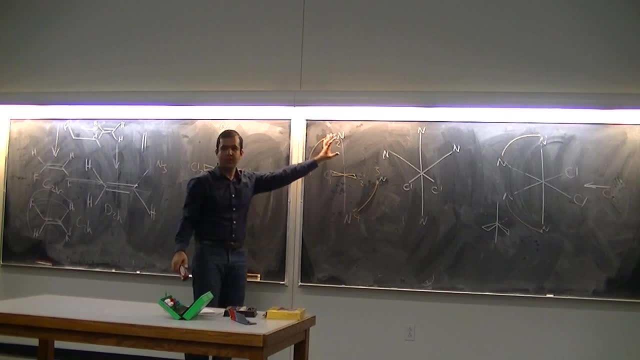 each other. So they- because I don't touch those bonds- Okay, So if N1 and N2 were connected before, they should be connected now N1.. So where is N1?? Oh, okay, Yeah, So N1 and N2.. Yeah, N1 and N2 were connected to each other before They. 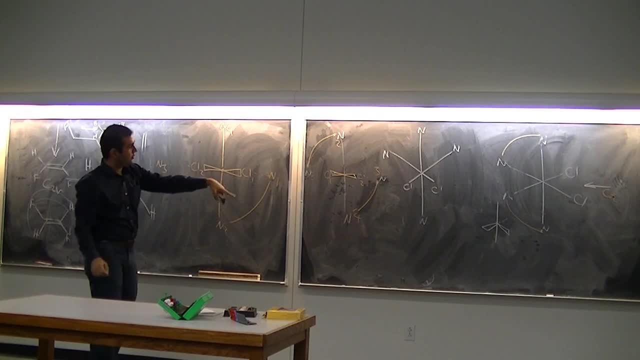 should be connected to each other. now. N3 and N4 were connected before, Is it not the same? No, It is the same, So it keeps the C2.. Okay, Yeah, If you will be given molecules like this, where it is an inorganic complex, where the 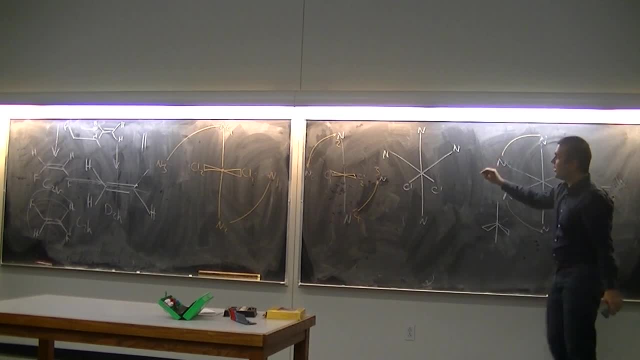 ligands are kind of connected to each other This way. so forget about all those lines that connect the ligands, Number them and apply the CNN and then reconnect them together and see whether it is the same molecule or not. Okay, 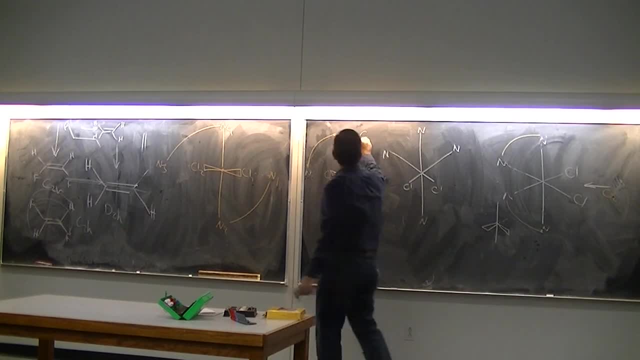 So it does have C2.. Right, Does it have perpendicular C2?? No, No. Up and down are different. Up you have chlorine and the back you have nitrogen. There is no perpendicular C2.. There is no sigma. You have to check for Sigma-B. Does. 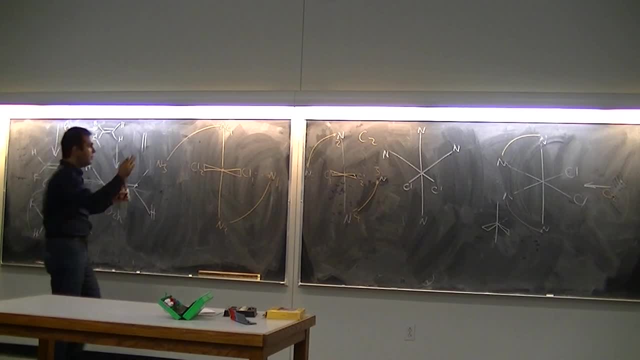 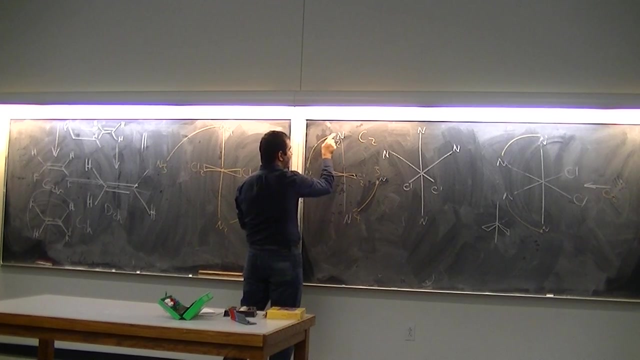 it have Sigma-B. No, No, If you apply the Sigma-B this – if you apply the Sigma-B here, this nitrogen two stays there. N1 goes there Right. So simply N1 and N2 – so that simply this. 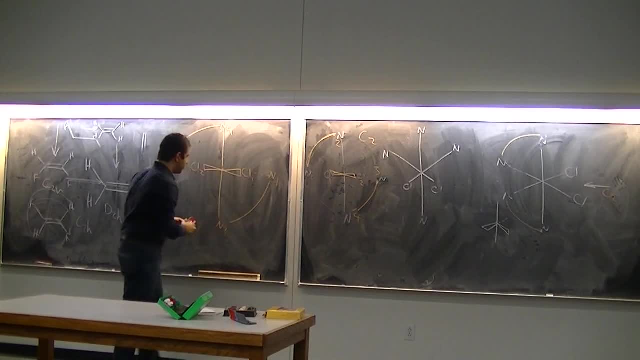 bond goes there and that one is going to be here, So the structure that you will get won't be this, If you okay, let me describe real quick. If you apply sigma v, n2 and n4 won't move right. 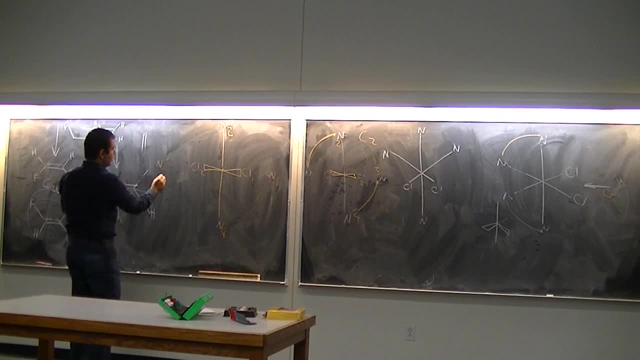 But n1 will go there and n3 will go here, right? So n1 and n2 are connected before. so this is what you get. This is not that Okay. What is the next thing to check? S, S4,, S2n, yeah, S2n. 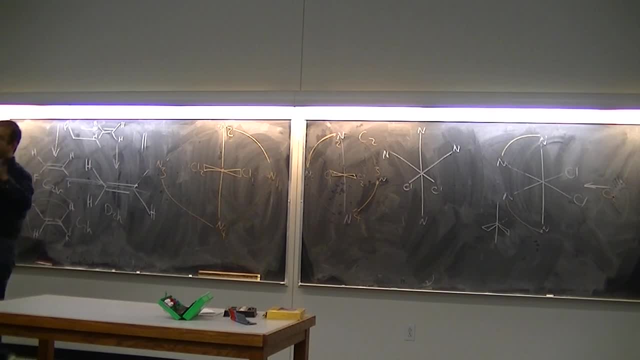 So, since our Cn is two, we have to check for S4. And, trust me, this does not have S4. So this is why the point group is C- It only has ones- and e- All right guys, Do you have any questions about these? 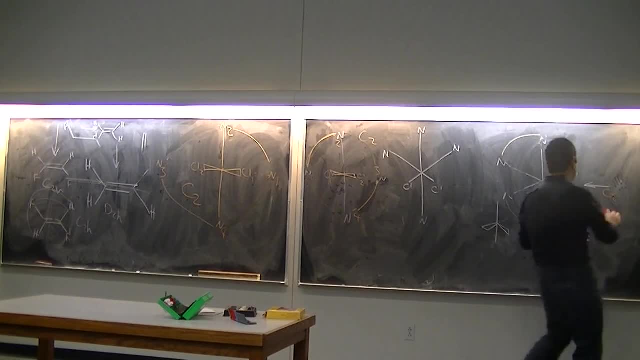 Now let's go to character table. What the hell is that character table with all those negative ones, zeros and stuff? Okay, Water: What is the symmetry element in water? E, C2, sigma v. sigma v- prime right. 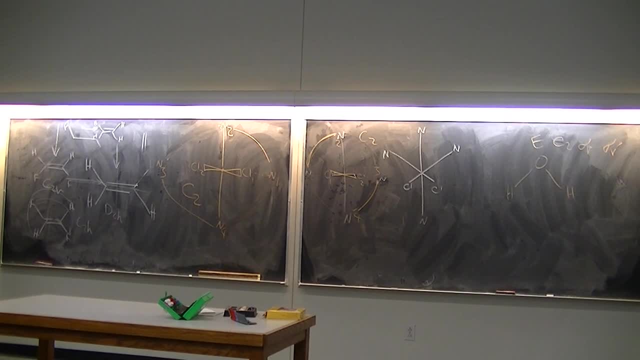 Is it not all that this molecule has, Right? do you all see all of those elements? What is the point group quickly: C2v, C2v right, C2. C2. Up and down or different Right. 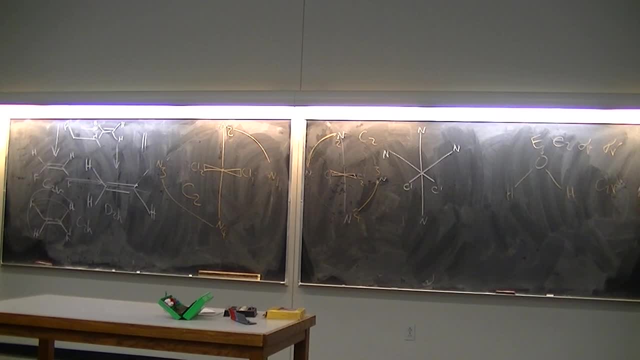 No spermic, no sigma. You have to check for sigma v and it does have sigma v, So it's C2v, All right, Okay. so what do we mean when we say that this molecule has all of those four operations? 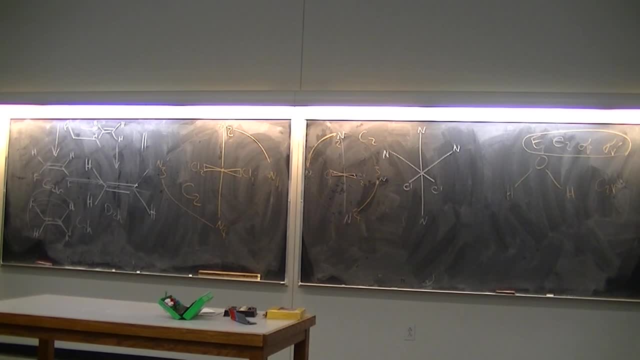 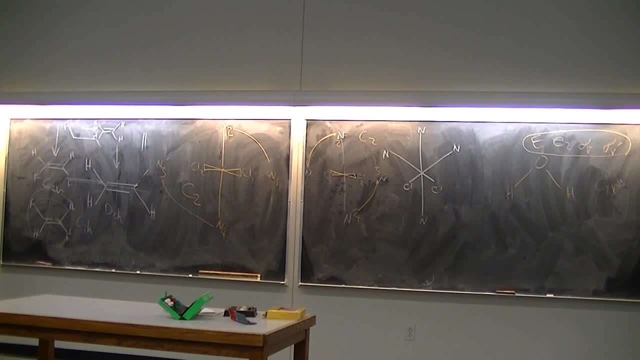 the starting point. Is it not what it means Now, if I kinda zoom in and go, so this is true for the whole molecule as we draw it, Okay, But if I kinda zoom in and go inside this structure, right. 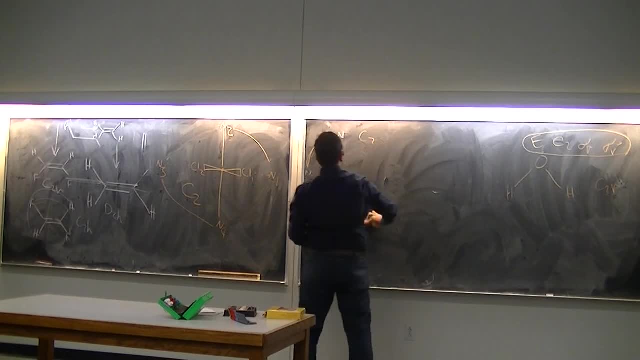 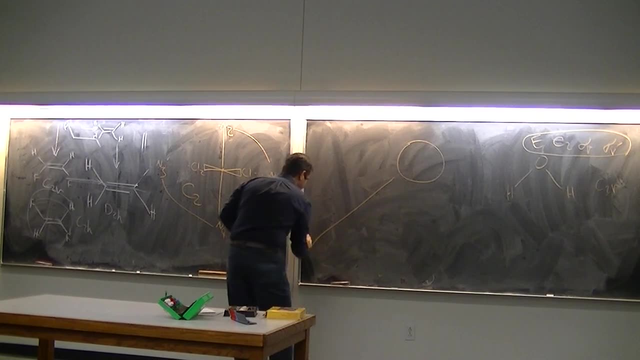 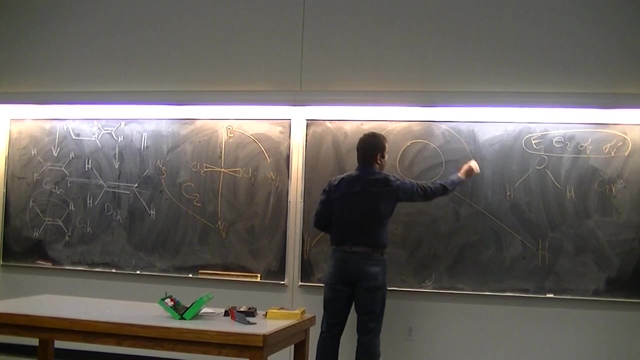 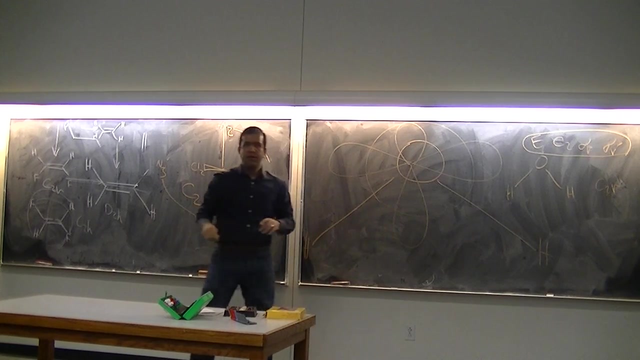 Let me just draw it right down. So if we zoom into that structure, there's this big hydrogen here, oxygen there, and there's this big hydrogen here. If I go inside, I can see some other stuff. I can see an s-orbital, a p-orbital here, another p-orbital down there right. 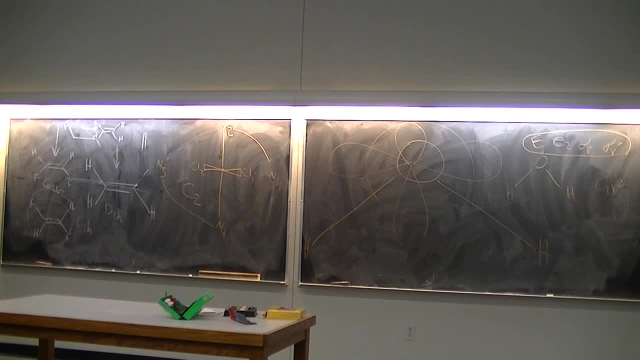 All of them are always there, although I don't see them right. So when I say this molecule has all those operations, it means that if I apply those operations it becomes itself. But if you look kind of inside it is not true for everything inside the molecule. 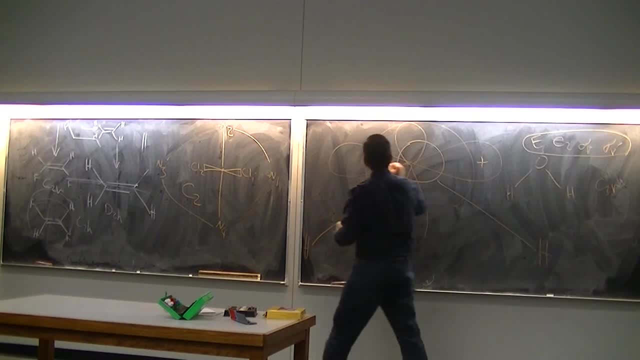 But if you think of this p-orbital, if you apply the C2, does it become something indistinguishable from itself? No, So although we say this molecule has C2, it becomes indistinguishable from itself, But it is not correct for everything inside the molecule, right? 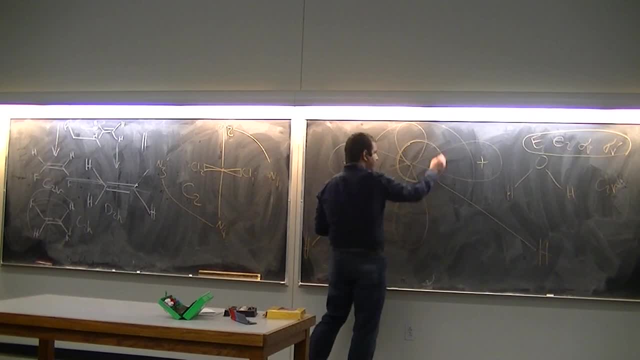 But if you look at s-orbital it's a different story. It has all of those operations. So it seems that like if you zoom in, you're going to go into a different world where there are different responses to each one of those operations. 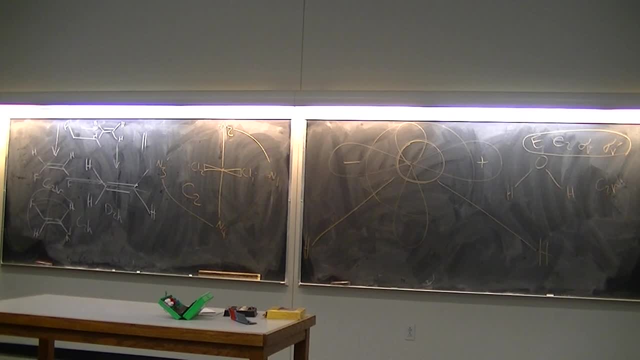 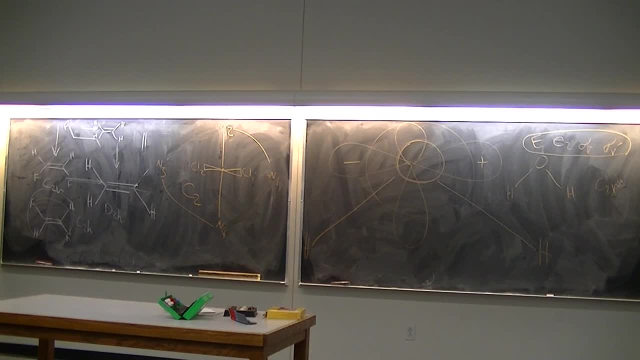 It has E It has everything. But if you zoom in you see different animals in there. If you think of s as one animal, it has all those operations. If you look at one of the p-orbitals, it does not have. If you look at another one, it does have. 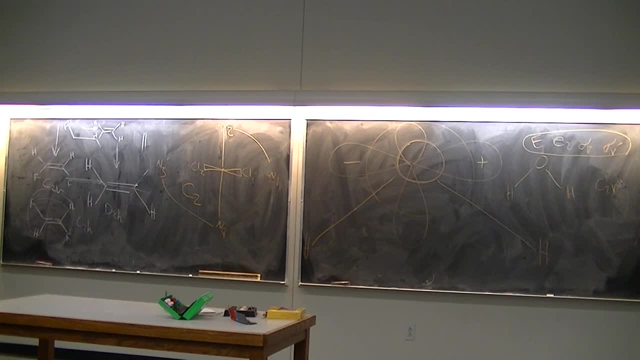 So if you zoom in, you see different behaviors, right. So we need to make a table in which we report all possible responses to these operations, That is, character table. Does that make sense, guys? So if you think of C2v as a function that you apply to a molecule, 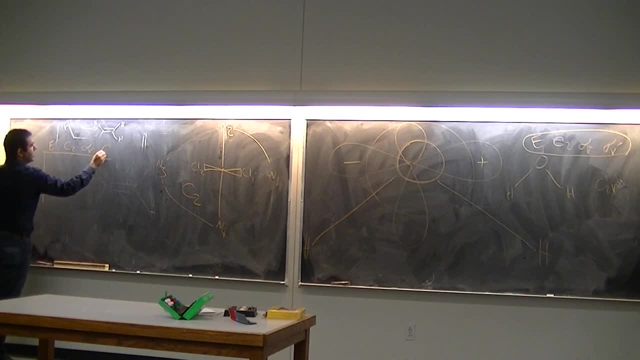 E, C2, sigma v, sigma v prime, you could get different responses. as you apply those operations to the stuff inside the molecule, right, Your molecule might be happy. The animal inside could be itself as you apply any of those, any of those operations, which is s orbital. 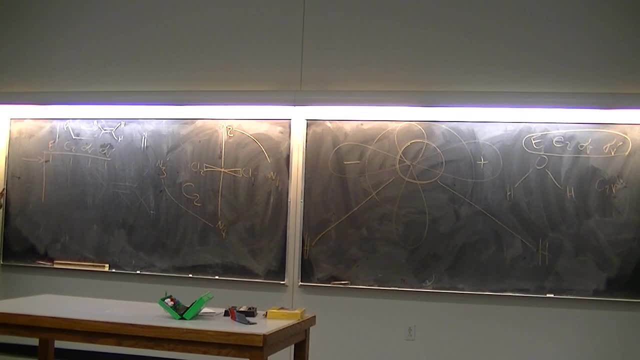 That is one response to the C2v operation if you think of the whole C2v as one operation. But there are some other stuff inside right that respond differently. They might give you something like this: There are other stuff that might respond like this: 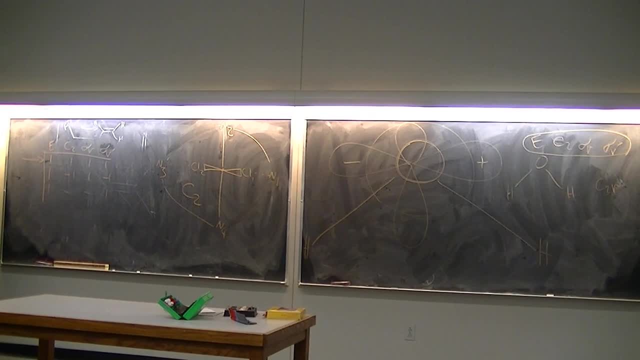 I don't know. I have to look into C2v to see what is in there. But it is actually important in the first place to understand what that character table is. Character table is the list of different responses that all the stuff inside the molecule could give as you apply those operations. 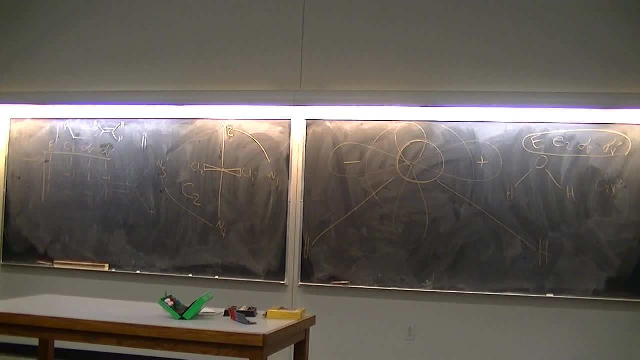 And since they behave differently- like s orbitals behave differently as you apply C2 when you compare it to p orbital. So we need a list of all different possible responses that you get as you apply those. That is character table. It is quite obvious that if you have more operations here, the number of responses that you could get is different. 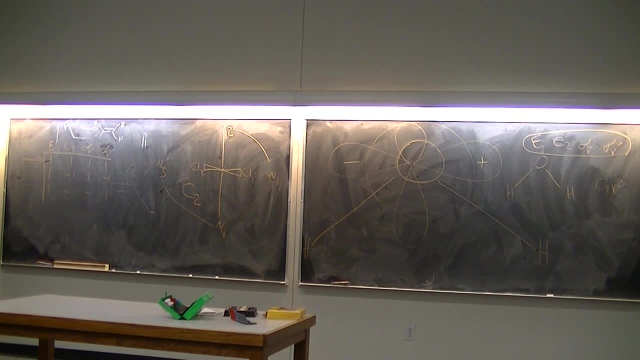 And that is why when you go, for example, to C4v, there are more responses here. Does that make sense, guys? Do you understand what the character table is? now, It is all different ways that stuff inside the molecule could respond when you apply those operations. 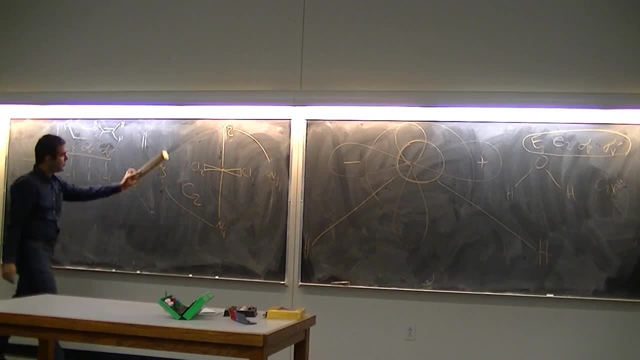 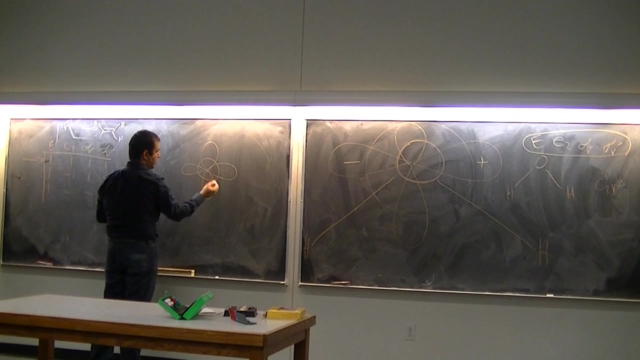 So if Now, if you think of water again, the oxygen of water, where it has like s orbital and three p orbitals, right, Negative, positive, negative, and there is another. So if you think of, Okay, Okay, 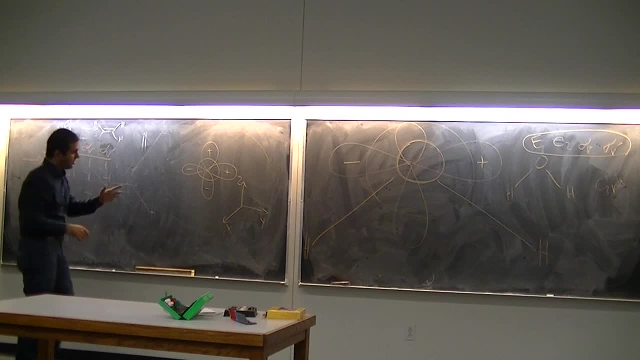 X and Y and Z. Yeah, If you think of X and Y and Z. So if you apply, Let's say we have gone to this world and we come across an s orbital. right, If we see the s orbital, if I apply D, what happens to that s orbital? 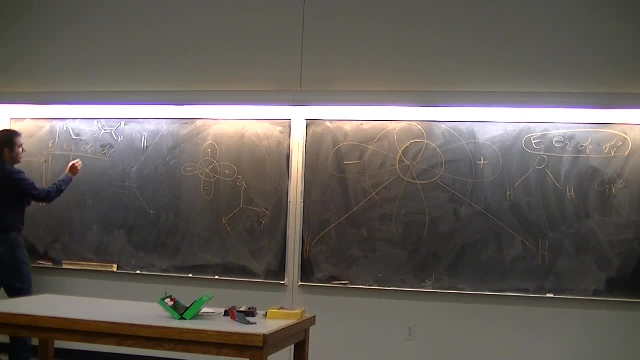 It becomes itself. If I apply C2, it becomes itself. If I apply any of the sigmas, it becomes itself. That is one way to respond to that. That is one way to respond to those operations. Okay, If you take PZ, for example, if you apply E, it becomes itself. 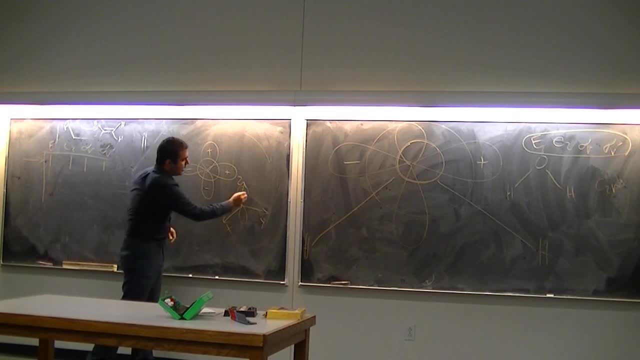 If you apply C2, rotate it by 180 degrees, it becomes itself. If you apply sigma B, it becomes itself. If you apply sigma B prime, it becomes itself. So the PZ orbital gives you the same response. Okay. 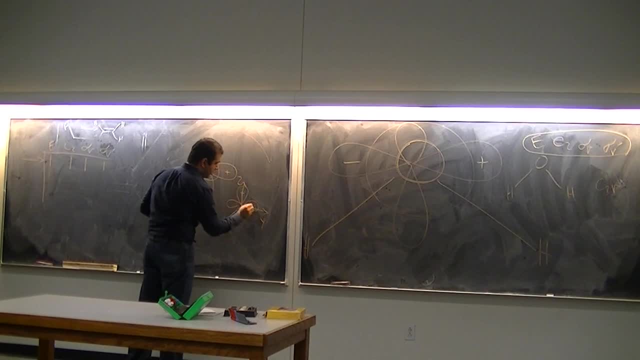 But if you look at PY, for example, If you apply E, it becomes itself, But if you apply C2, it becomes negative of itself, Because the positive and negative flows will match up. So it becomes negative of itself. It does not have C2.. 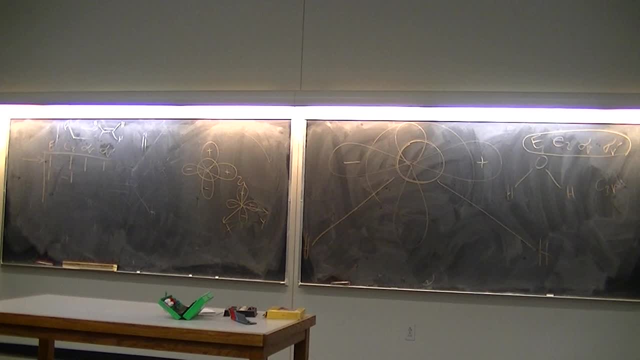 Although the molecule, when you think of it from outside, it does have the C2. But the PX inside of it doesn't have the C2. Okay, It becomes opposite of itself. So if you apply sigma B, Let's say sigma B is the one that goes through the Y-axis. 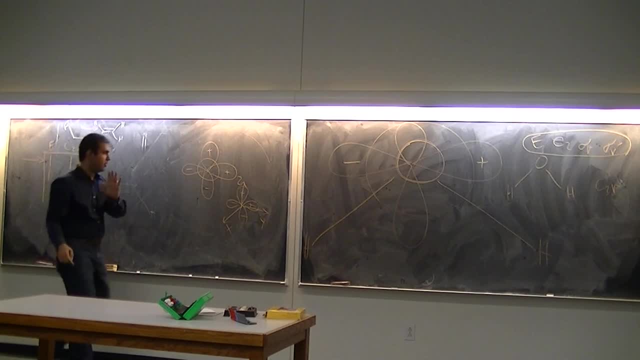 It does have it, But if you apply the other sigma, which is the PX, it reflects negative to positive, It becomes negative. That's another way. There are some animals inside that world that behave like this as we apply the operations. Okay. 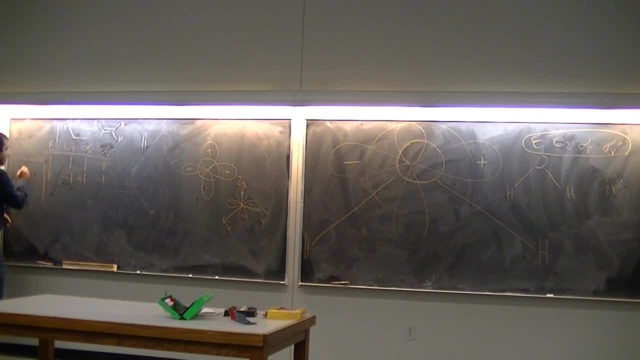 And two other responses. It's interesting that the number of responses that you can get, the number of different behaviors that you could have, is equal to the number of operations that you have in there. So if you see four operations up there, there are four symmetries. 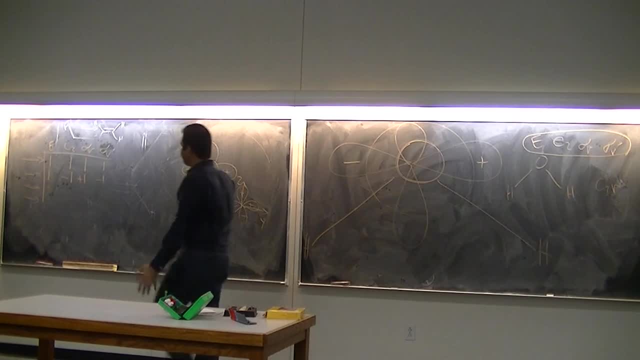 So you can think of these And they call them differently. So this is A1,, for example, Right, So A1, B1, I don't know what the other ones are. So you can think of this, You can think of these as different symmetries inside C2V. 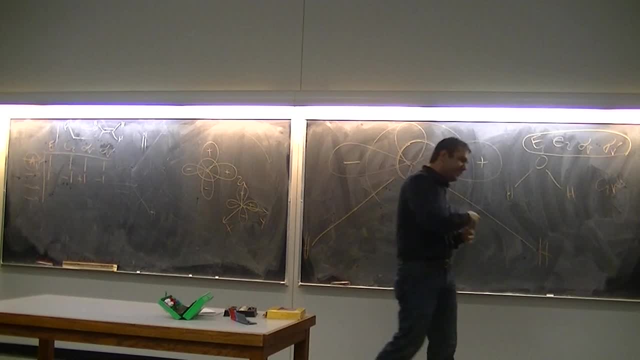 So if your molecule is C2V like water, the stuff inside of it can have may belong to one of those four responses And the terminology that we use. we say that, for example, S-orbital has A1 symmetry in C2V. 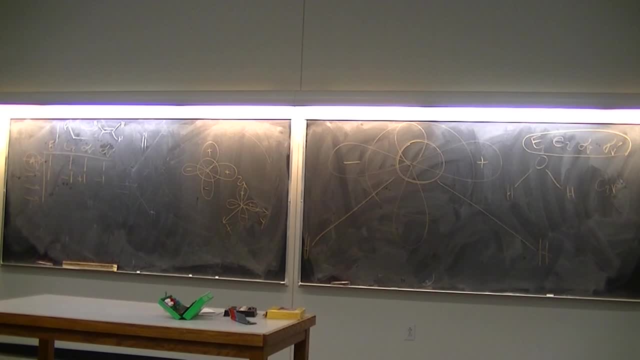 It means that its response to C2V is A1.. Okay, Does it make sense, guys? Yeah, So the Z for the Pz. is that a minus and a minus, or a plus and a minus? For Z, it's a plus and a minus. 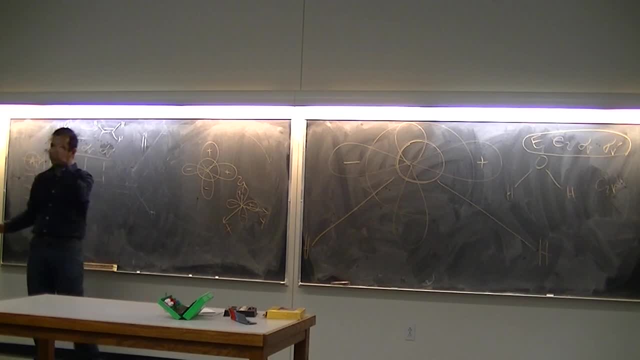 P-orbitals are not symmetrical. so Okay, and so What's the difference, like why? What's the difference between the Pz and the Py, then, In terms of Px, Py and Pz? 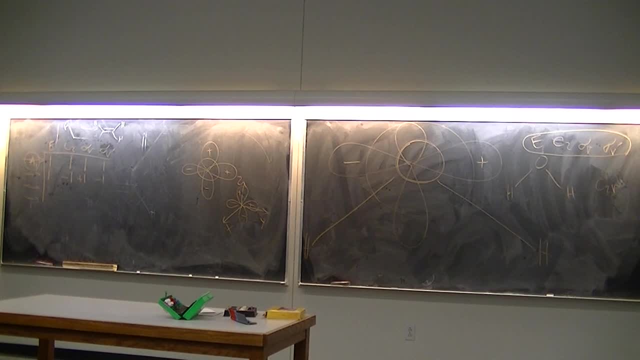 all of them have like two loops Right. One side is negative, positive and the other side is negative. Pz is elongated toward the z-axis, Px is elongated toward x-axis. Yeah, So when you apply to C2, it goes. 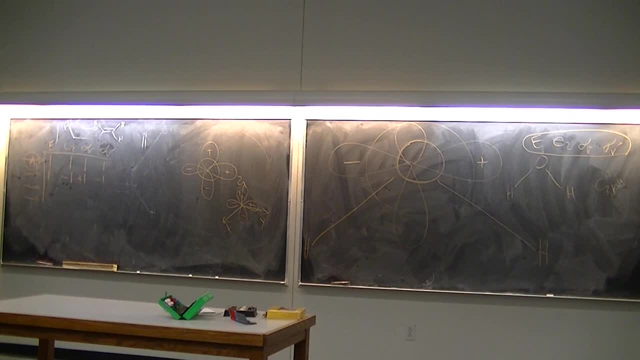 So the Pz and C2 are on the same axis, So it doesn't change it Right. But if you think of Px, it just does change it. So they So that C2 doesn't touch Pz, That Pz is the same. 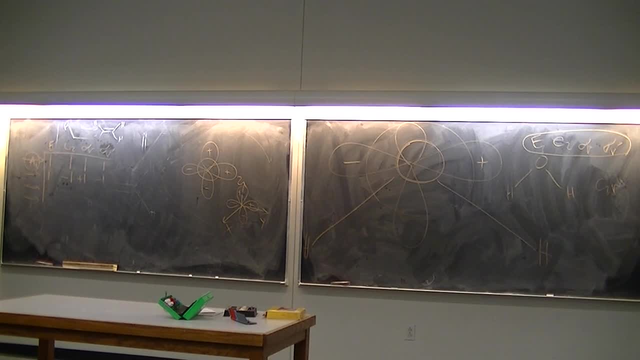 It doesn't feel that way. You apply C2, it says: okay, I'm fine, I'm myself, But the Px, It does change. You know, when you apply the C2, it becomes something else, It becomes negative of itself. 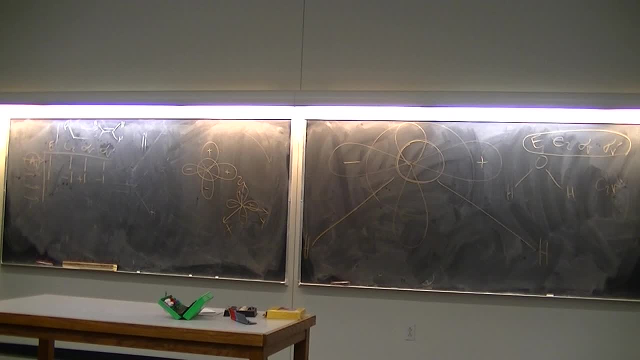 So it does feel the C2.. So they have different behavior. If you zoom out and look at water, in all cases you see. You say that it becomes itself If you apply C2, C2.. Yeah, it's the same water. 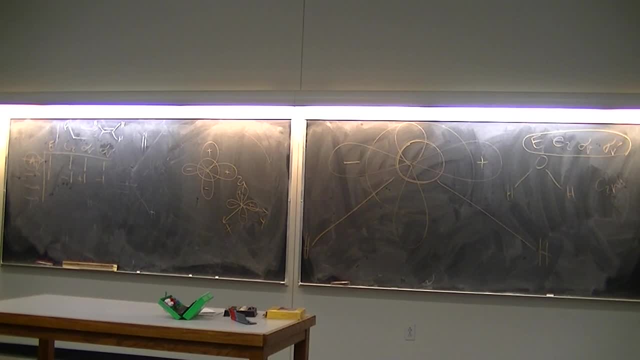 But when you go inside, you have different behavior. And that's what character table is. It lists for you all different possibilities that you could have as you apply those operations. Now you So remember. each one of them is what, Guys? it's important to understand the concept that means. 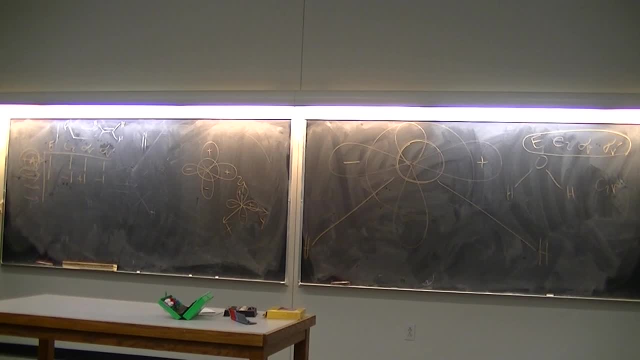 Each one of them is one response to C2b symmetry. Okay, And the terminology is that each one of them is the symmetry of, let's say, s-orbitol or p-orbitol under C2.. So if, for example, s-orbitol has A1, which is the case, 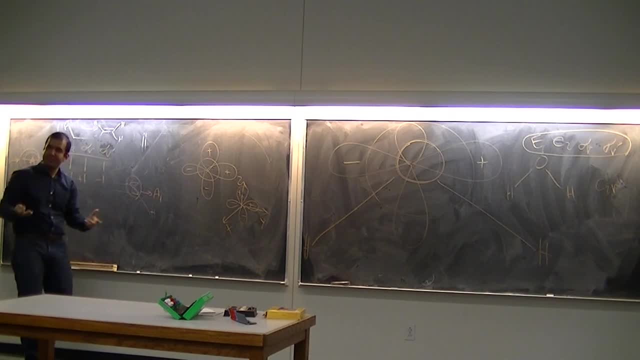 the terminology is this: S has A1. S has A1 symmetry. It means that its response to C2b is A1. It's 1, 1,, 1, 1.. Okay, So each one of them is the symmetry of one orbital. 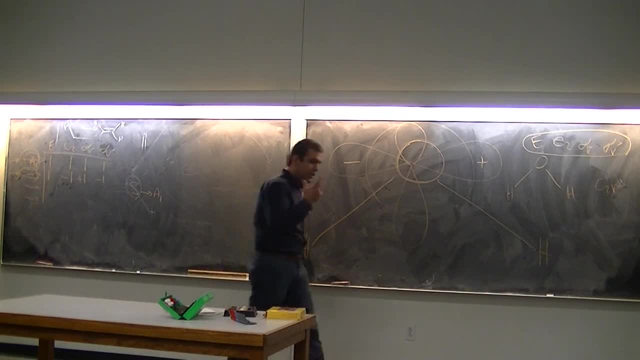 So it's interesting that for two orbitals which are going to interact with one another under a symmetry, they must have the same symmetry, They must belong to the same, They must have the same response as you apply C2, sigma and everything. 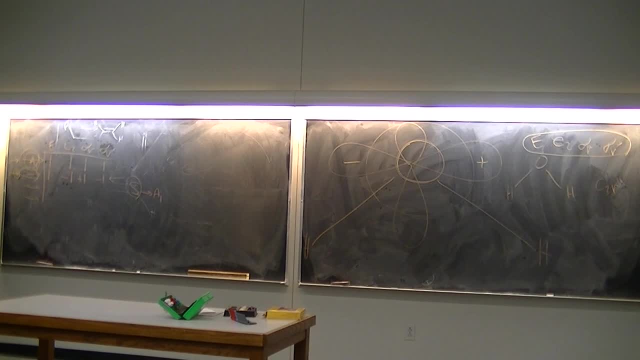 If they have the same response they can interact with one another. Otherwise they cannot. Okay, And we take advantage of this fact to draw the molecular orbital diagram. So let's say they ask you to draw the molecular orbital diagram of water. 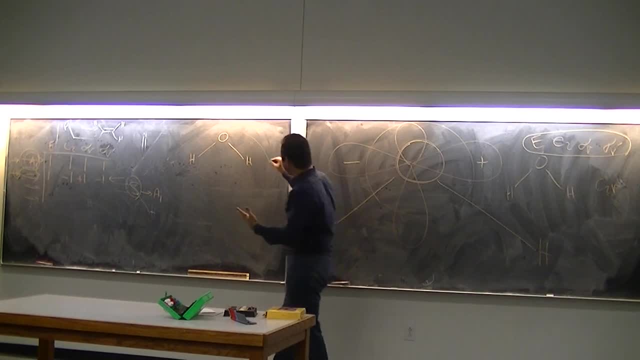 So, if I want to translate what I just said, I have two s-orbitols of hydrogen and I have a bunch of orbitals on oxygen, Right, Is it fair? Now they want to interact. The two s-orbitols want to interact with the orbitals of oxygen. 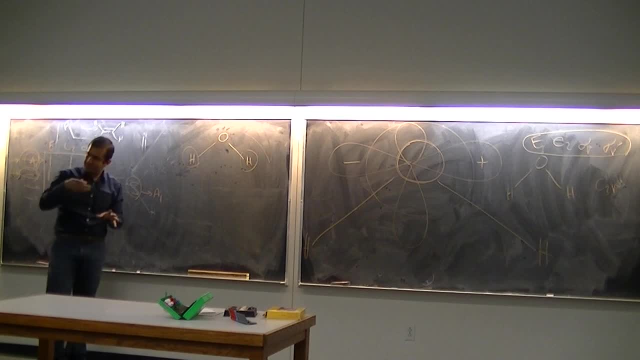 What is the condition for them to be able to interact with one another? They must have the same symmetry. If these two s-orbitols can find orbitals on oxygen that have the same response, they can react with one another. If they cannot find those, orbitals cannot react. 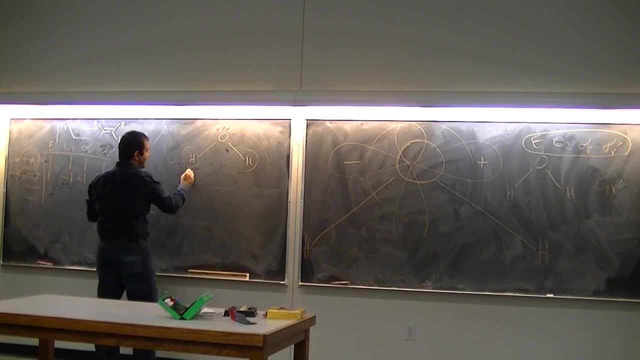 So let's say: Let's say the symmetry of those two is A1 plus B1.. Let's say: Right, But the symmetry of the orbitals on the oxygen is A1 plus B1 plus 2B2.. Let's say: 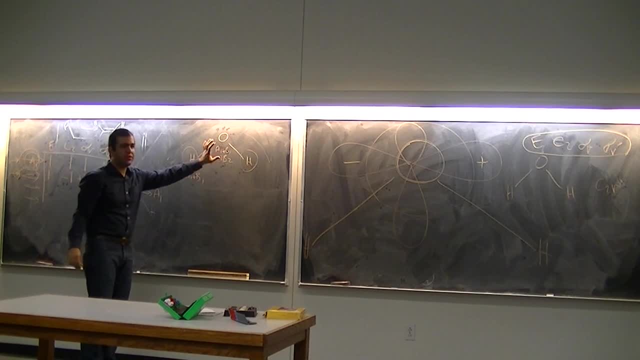 Okay, And remember, these are the symmetry of orbitals under C2B. Is it clear guys? This is the symmetry of orbitals on oxygen. This is the symmetry of the two s-orbitols of two hydrogens. This A1 and B1 from these two can interact with this A1 and B1.. 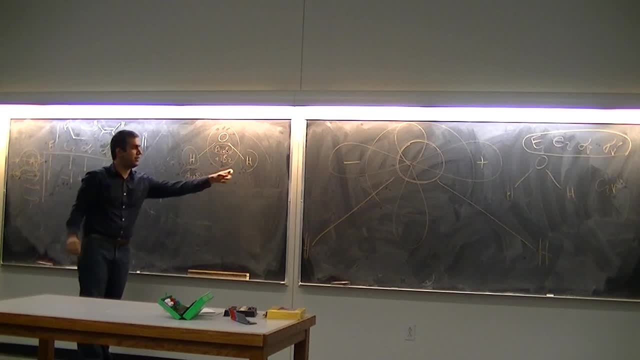 But that B2 that has a symmetry that does not match that of these two hydrogens, it just remains non-bonding, It just does not react. So in order to draw the molecular orbital, all you have to do is to find the symmetry of the two hydrogens. 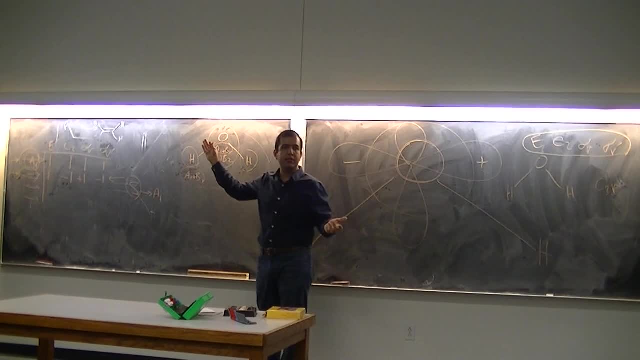 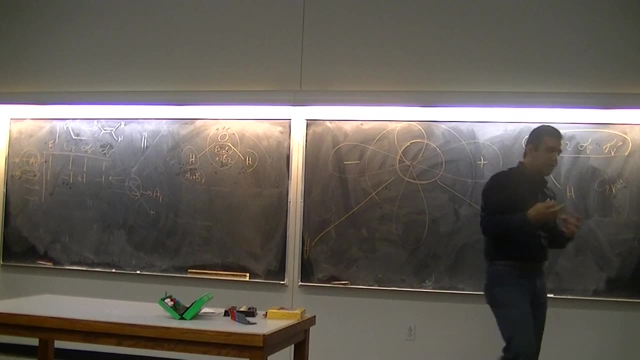 and the symmetry of oxygen and see if each one matches. That way you can draw a molecular orbital diagram. Is it clear? So it all comes to the conditions for two orbitals to interact. The conditions for two orbitals to interact is to have the same symmetry. 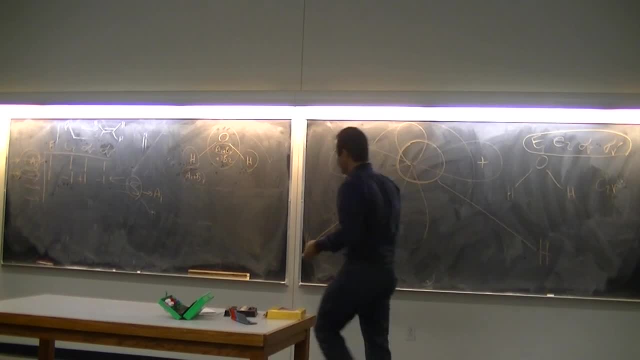 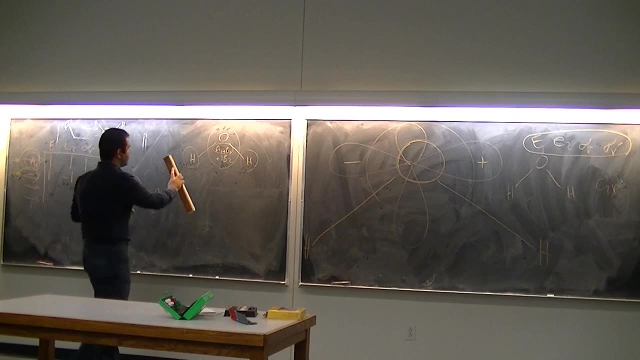 Okay, So all you have to do is to figure out what the symmetry means. Okay, Let's. I know Dr Aramarti did this in class, but Let's do another one. Guys, do you have the character figure? 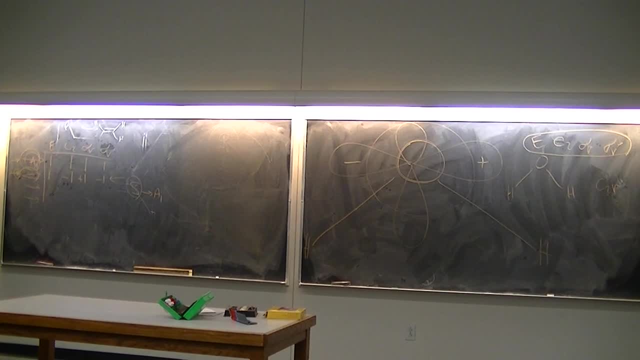 The one with all the numbers and stuff in it. Can you figure out what that means? I just want to see something that is E4H. Okay, we don't have that crazy stuff. Okay, E4H is good, Okay. 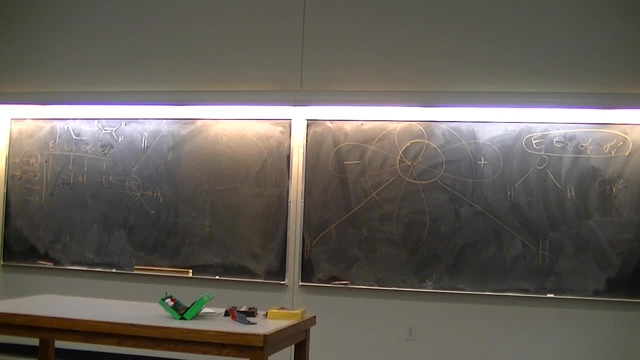 Can I borrow this? All right, guys, Let me draw the character table of. Let's say we want to draw the. Let's see here, It's not fun. 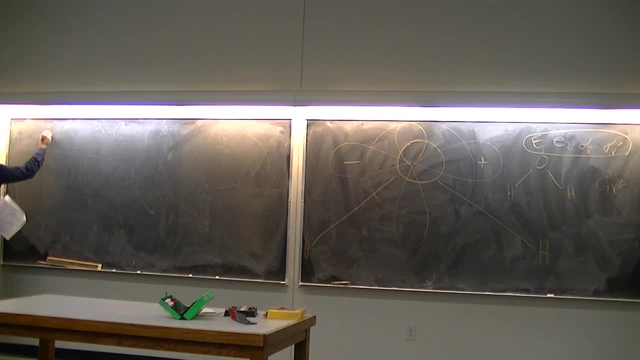 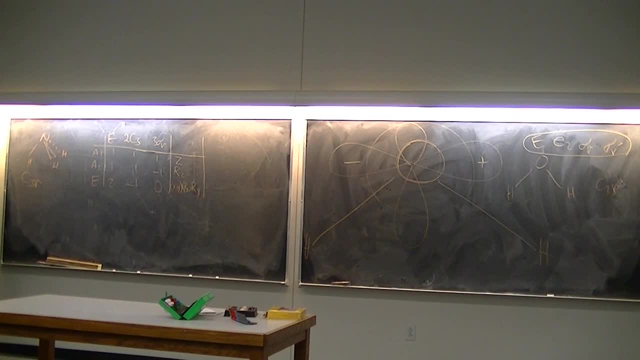 Okay, So you have to figure out the symmetry of orbitals on nitrogen, because your point group is C3D. you have to see the symmetry of orbitals on nitrogen under this point. This is nitrogen. nitrogen has 2sc's. 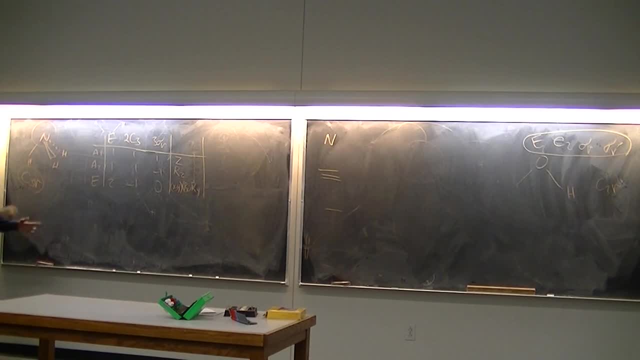 and 2p right. What is the symmetry of the s-orbital under c3d? It's always 1, 1, 1,. whatever that 1, 1, 1 is all 1, because it's so symmetrical, it responds 1, 2, and. 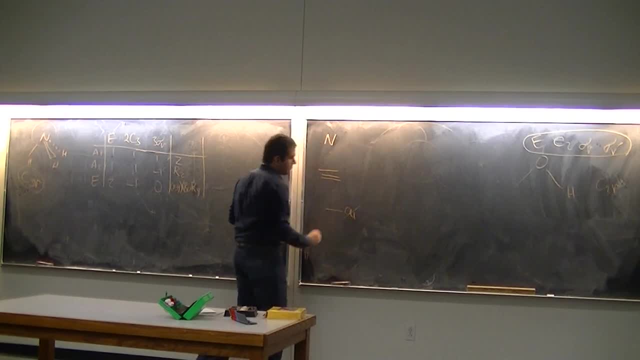 8.. So this is a1, all right. What is the symmetry of the p-orbitals? Well, in the second column, if you look at x and y and z, those are the symmetry of px, py and gz. 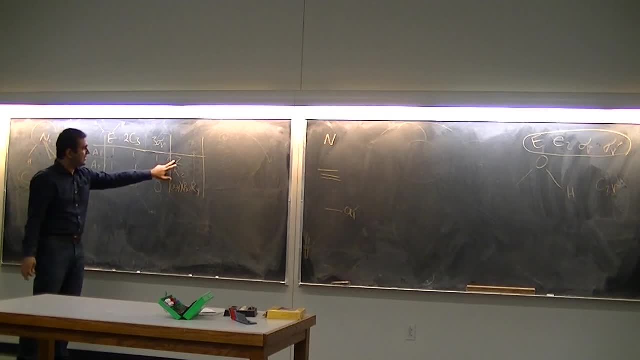 So the pz belongs to a1, but x and y together belong to e. Do you know why? what e is with that? two levels, level two there. If you rotate this molecule by 120 degrees, what happens to x and px and py? 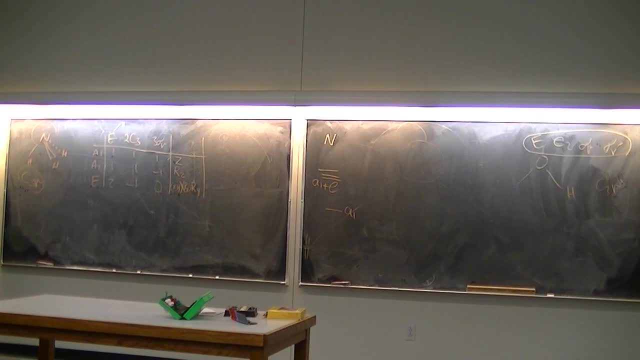 They will be related to one another, Right? X does not completely become opposite of itself. X will have some distribution in the y-axis and y will have some contribution in the x-axis, because you're rotating it by 120, right? If you think of px and y are 90 degrees. 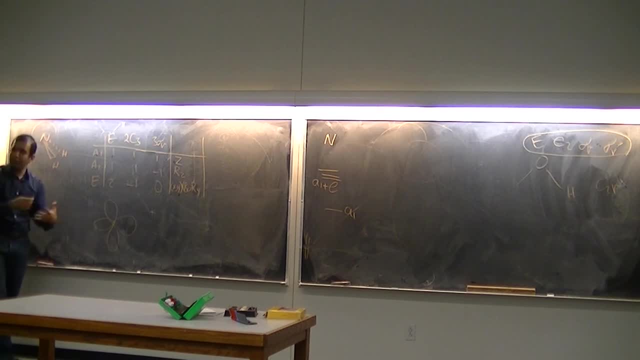 so if you rotate it 120, it goes there, So they will be mixed, x and y together. respond: okay, That's why together there's the. and remember e, 1e is two orbitals. Okay, So you don't want here, you don't want to write 2e, just 1e, But each e. 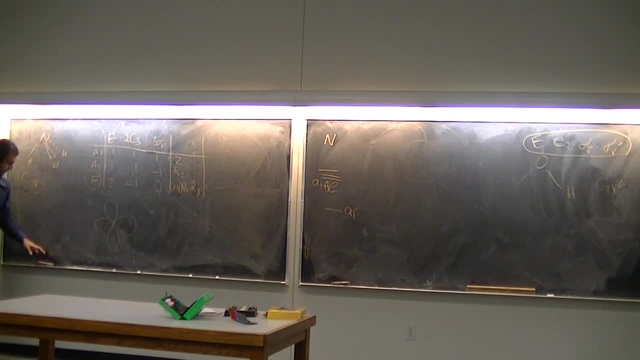 contains two orbitals. okay, That's it. that is the symmetry of p s-orbitals, px, py and pz. Okay, You have to figure out the symmetry of those hypogems For that. this is the. 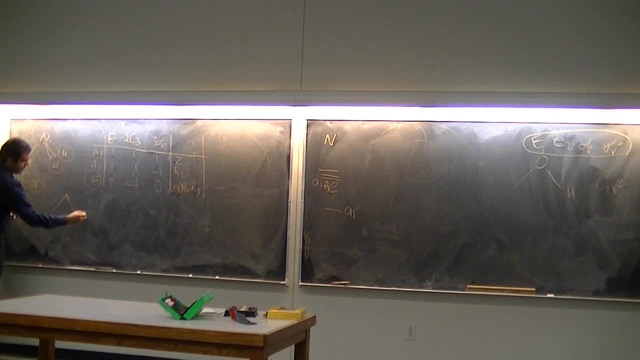 trick. you have to draw three vectors. right? You draw three vectors and you apply these operations and see what happens to those. If they move, you assign 0.. If they don't move, you assign 1 for each. Okay, 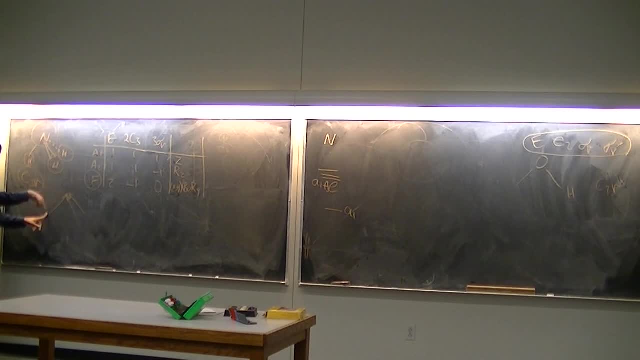 So this is again NH3.. Are you cool with it? So if I apply e how many of them will not move? Does any of them move if I? if I apply? e No, So how many of them do does not move. 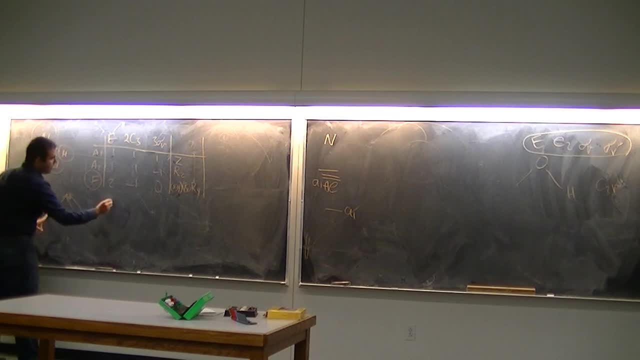 3. So if I apply e, I get 3.. You see, you have to figure out the response because it's not in the table. Okay, So px, py, pz is simple because the symmetry is already listed here. You have to figure out the symmetry for those three, So you get. 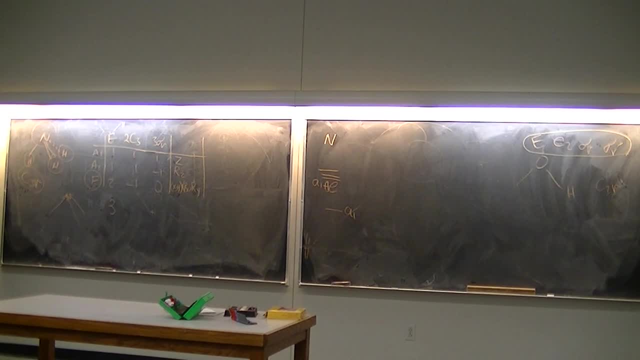 3 if you apply e, If you apply c3, how many of them move? 3.. So you have to figure out the symmetry for those 3.. So you get 3 if you apply e. If you apply c3, how many of them move? 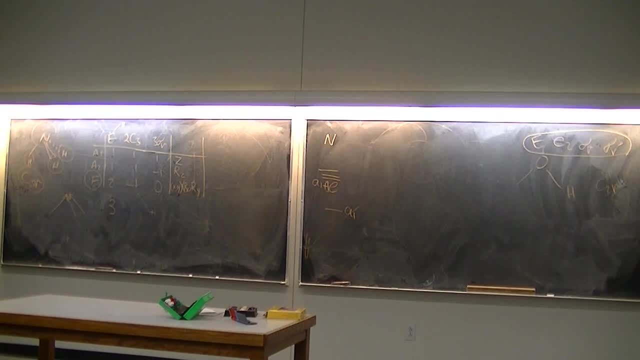 All of them, So you get 0 for all. Remember, if you move any of them, you get 0 for that vector. Okay, So this is here. If you apply sigma v, how many of them move? 2 of them, But one of them does not move Right, So you 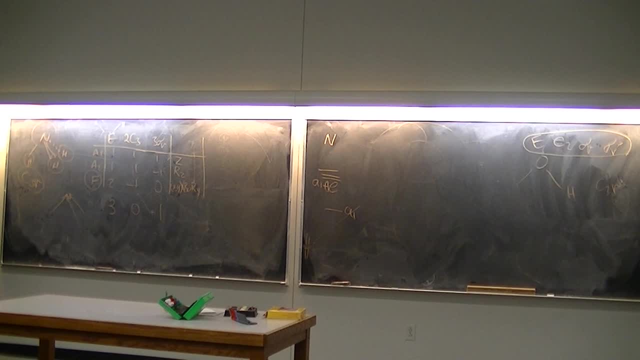 get 1.. Does it make sense? So this is the difficult part. You have to figure out the symmetry of those 3 hydrogens by applying that onto the vectors that those 3 make. This is the symmetry of hydrogens. This is the symmetry. 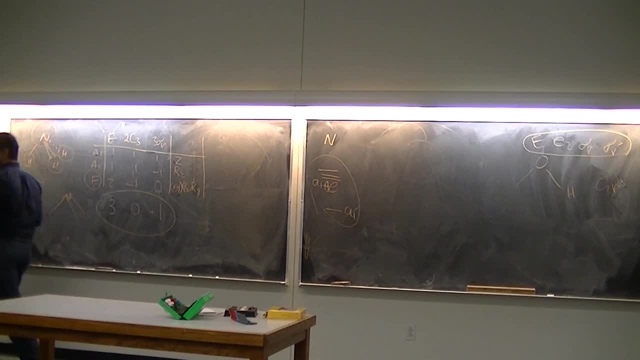 of s and p orbitals on the nitrogen. Okay, But this is a representation, that is some of the that could be actually sum of two or three of them. okay, we call this a reducible representation. okay, which one of them, which two of them were? maybe. 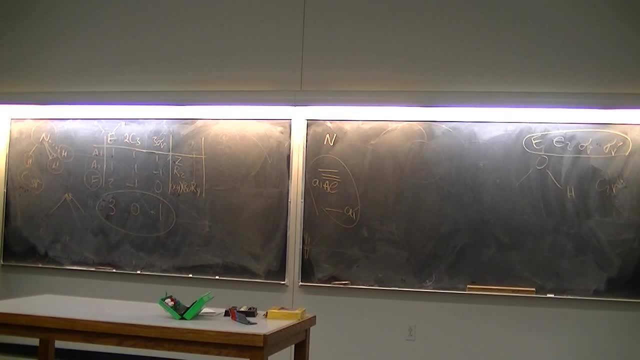 three of them should be added to make that, if I had E, A1 and E, does it make that? in the next session I'm going to teach you a method that for more complicated, like representations, it gives you a formula and you can get one combination of those, because sometimes it's not that obvious. sometimes we have 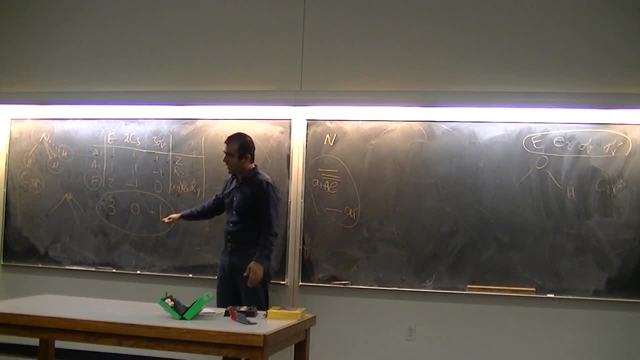 to use a formula to see which one of them you have to add together to make that. but here this is obvious: if you apply A1 and E, you will get that and there's no other combination that would give you that. okay, so the sim n. they show this by- I don't know what this is- by this gamma. okay, so your. 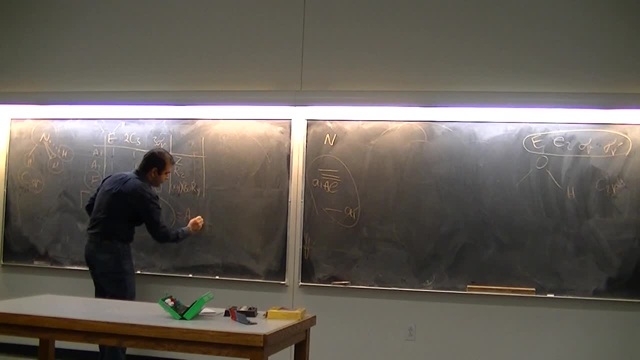 representation is this: which equals a1 plus. this is the symmetry of hydrogen, this is the symmetry of. so the three vectors on the hydrogen that you have has a symmetry of a1 plus. this is the symmetry of hydrogen. that is the symmetry of of nitrogen. anything that can interact will interact. okay, a1 is there. 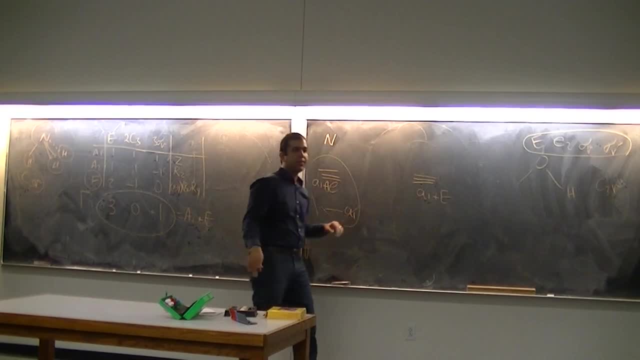 a a1 on the other side, that matches that a1. yeah, you have a1 here and a1 there. they do interact. how many orbitals from this side are you taking? how many a1s here? two right, one a1 here. you know, for this a1 it doesn't matter. 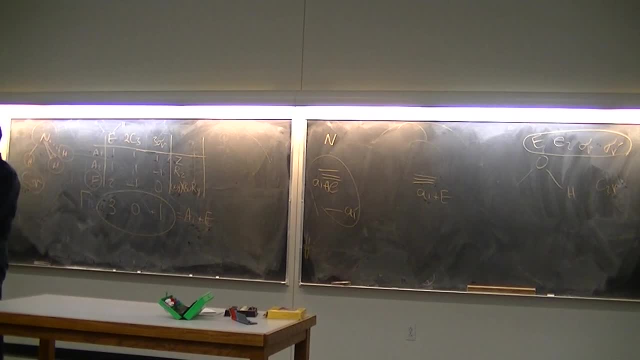 whether it's a1 or a2, it doesn't matter whether it's a2 or a3, it doesn't matter whether the other a1 is s-orbital or p-orbital. as long as they have the same symmetry, they will interact. okay, this a1 finds two other a1s on this. 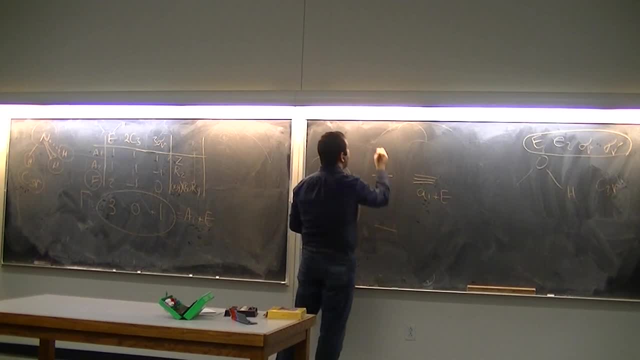 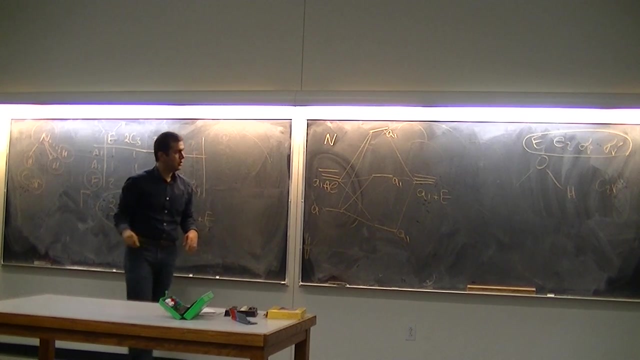 side. all three of them are going to interact and eat three new a1s. okay, now, if you want to draw it, you can draw it like this. oh, you don't have to draw, but okay, one e here, one e here. do they interact? yes, e and e match, so you have two. 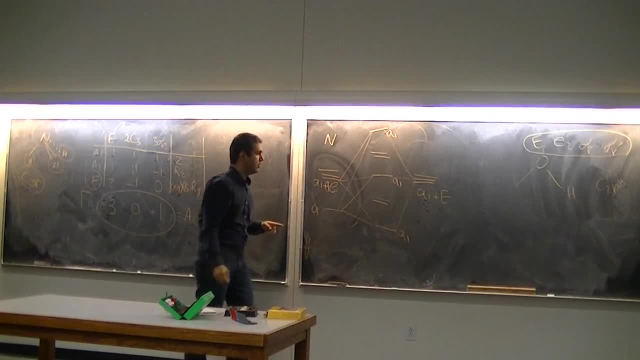 orbitals- remember one is two orbitals: this is e and this is d. If you have odd number of orbitals, you get one non-bonding in the middle and half of them will be bonding, half of them will be anti-bonding. 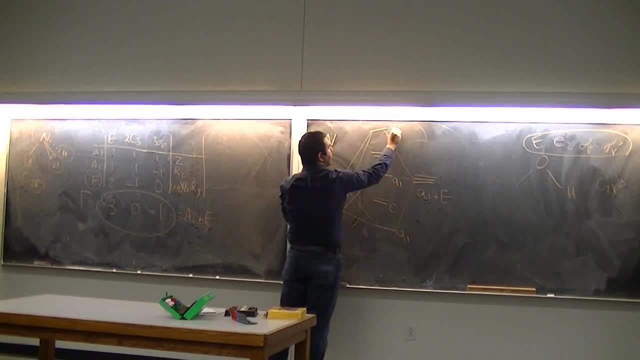 So this is non-bonding, this is bonding, this is anti-bonding And this is non-bonding. If you have even number of orbitals interacting, you get half of them bonding, half of them in the anti-bonding. 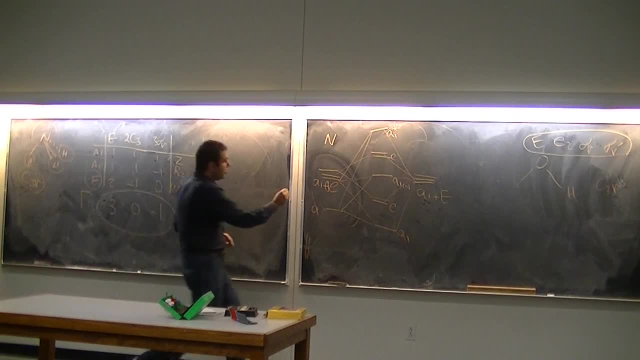 You got it Okay. sometimes you also have another B1 here. It's not the case here- But you have something that does not find a match to the other side. It just remains as it is Because it cannot find something to interact with. Does it make sense? Yeah, 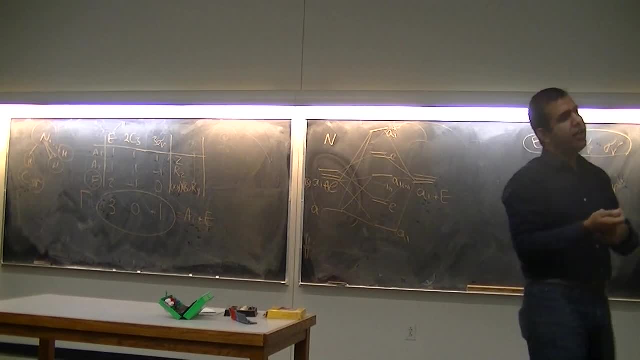 Does that become a non-bonding? Yeah, it becomes a non-bonding. So you get the symmetry and you look what matches from the two sides- Okay, Those that match. You simply match them and write them in the middle. 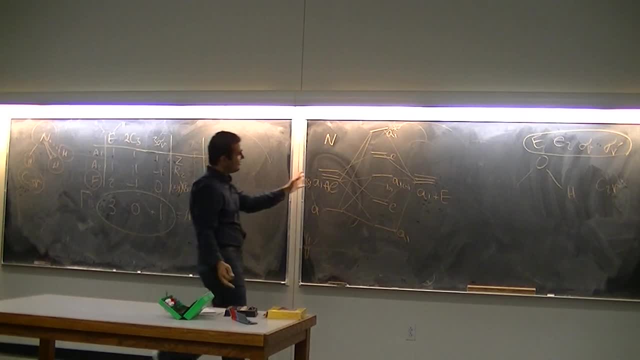 If you eventually have even number of orbitals, you know that have a match to the other side. half of them will be bonding, half of them will be anti-bonding. If you have odd number of orbitals interacting, one goes in the middle again: half bonding, half non-bonding. 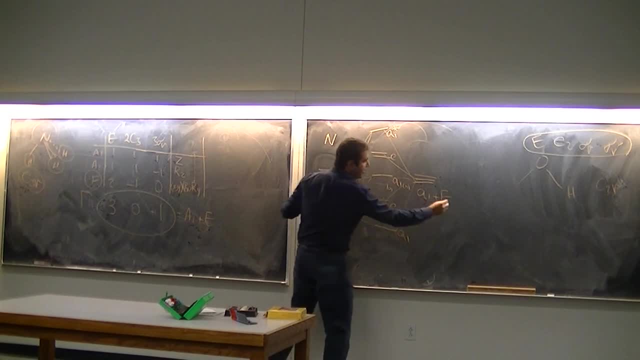 If you don't, if you have B1 here and I don't know T here, for example, if they don't find a match, they simply show up in the middle. They don't disappear, But in the same energy state that they used to. 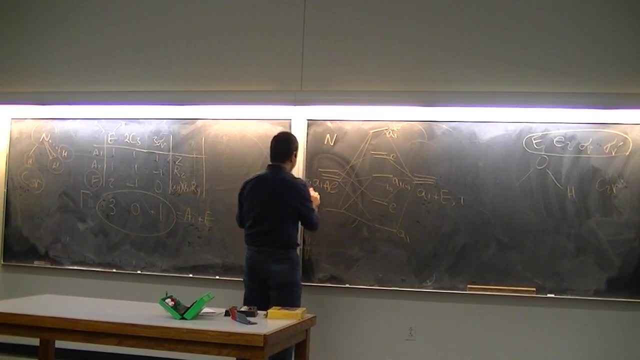 Okay, So we don't have a B1 here. So this is ammonia. How many electrons do you have in ammonia? Five from nitrogen and three from hydrogen. So you have eight. You get one, two, three, four, five, six, seven and eight. 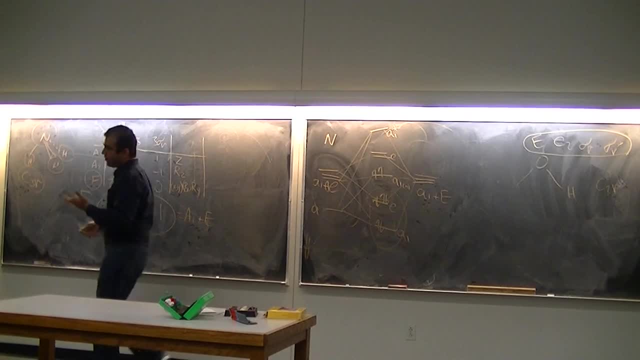 These are bonding, So the bond order is three And this is non-bonding. That's actually the lone pair of nitrogen, And that's it. That's how you draw it. I know it looks confusing, but if you think about it, orbitals that have the same symmetry will interact right. 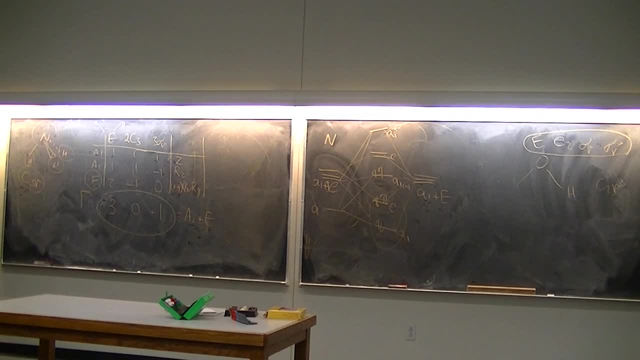 So you have to figure out the symmetry of orbitals under that point group. Orbitals on the central elements simply come. the symmetry of them is obvious because they are listed in the character table Right. So just draw the orbitals S and P orbitals and kind of extract the data from the character table. 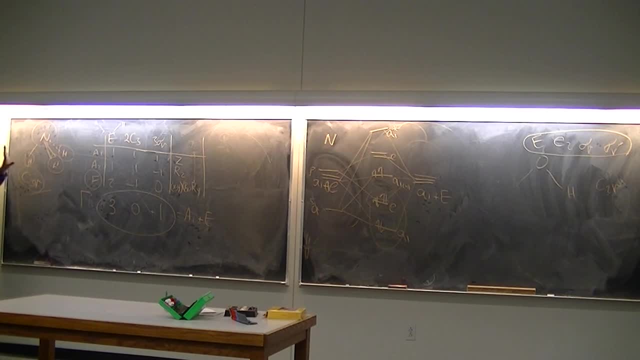 For the elements that are not central, Central, you draw vectors, you apply these and get this reducible representation. Then you figure out what combination of those will give you that. That is the symmetry for the three hydrogens, And then you look at what matches. 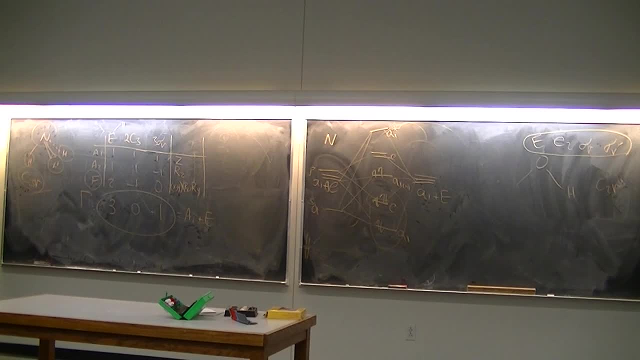 Okay, Do you have any questions now? No, Alright, No questions, You got it Alright. Thank you guys for coming And I'll give attendance to everyone for this. I will post the video on YouTube, probably tonight. Is this still recording?